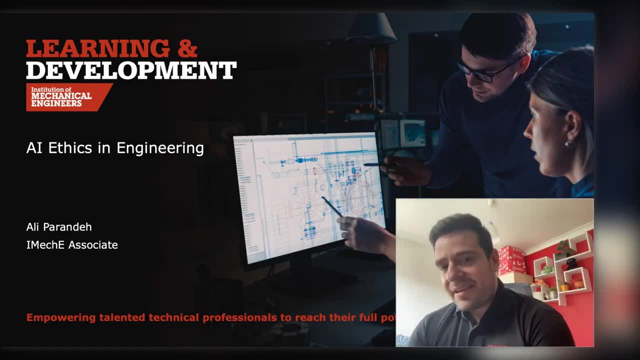 It's a pleasure to meet everyone. Thank you very much, Dan, for presenting the housekeeping and introducing me. It's a pleasure to meet everyone And I'm really excited to share you more about the webinar today and what we're going to be covering, as well as a bit of introduction to 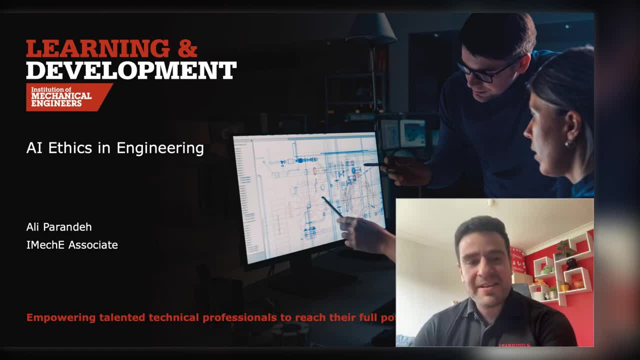 myself, So my name is Ali. I've recently joined the Haimeki L&D as an associate to help develop more content on AI, because it's such a hot topic technology And I think it would have been. it's a great idea to start this discussions around, especially AI ethics. 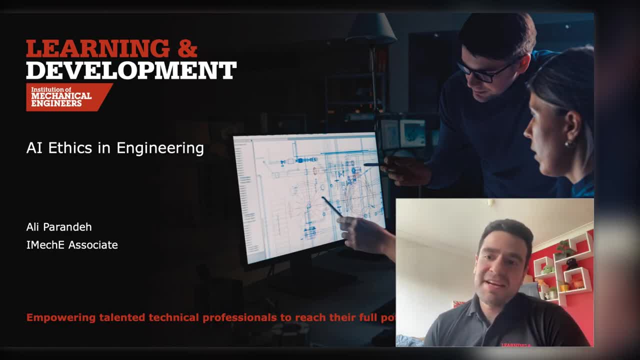 because it's such an important topic And I think in engineering context, everyone is really interested to learn more about it And I feel like it would be great to start these discussions and have this webinar to go through it together. So my name is Ali Parande. I come from a mechanical 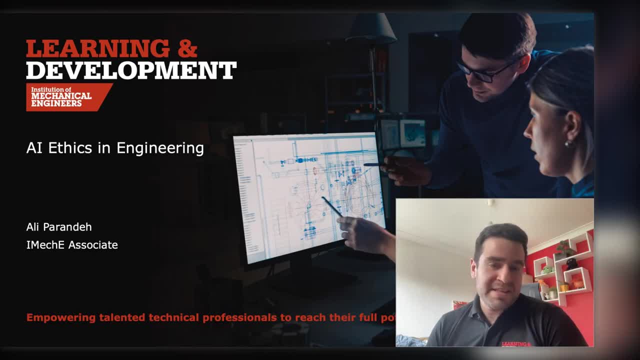 engineering background started my career with Atkins. started as a systems engineer so was mostly working on complex rail projects in the verification, validation settings and system specification settings, But then gradually my career rolled towards more into AI and working with Python, working with all of these latest technologies. So I think it's a great opportunity. 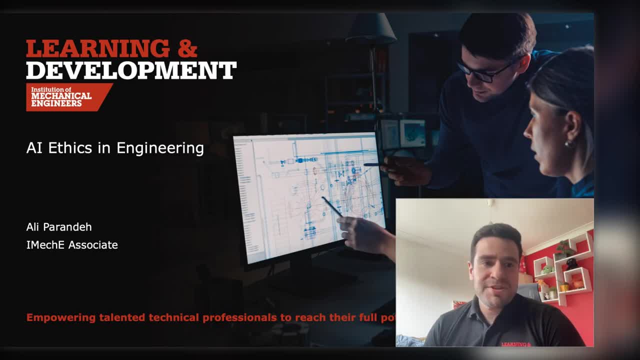 to start this discussion around AI. So my name is Ali. I've recently joined the Haimeki L&D as an associate to help develop more content on AI because it's such a hot topic technology, And I think it would be great to start this discussions around AI because it's such a hot topic technology. 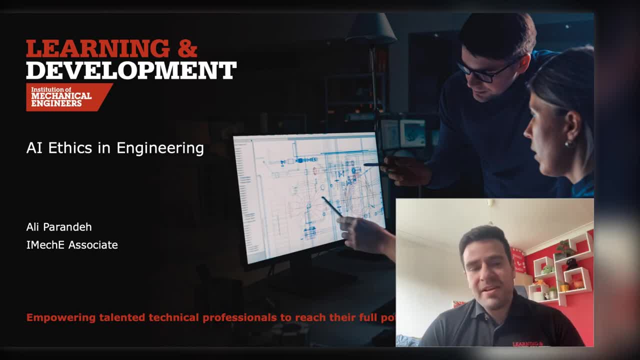 So my name is Ali. I come from a mechanical engineering background, started my career with building computer vision models for vegetation management in rail, as well as predictive delay analytics and predictive maintenance and anomaly detection on pantographs, And basically spent quite a few years over there and recently joined another. 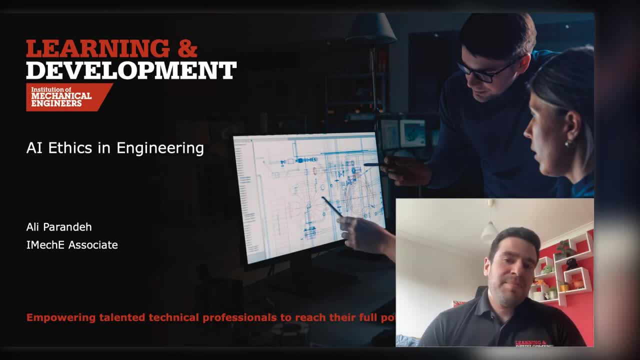 consultancy as a head of engineering and been basically helping with building more and more AI tools to help the engineering sector especially like. my particular interest is in rail and computer vision, But I have recently started gathering some experience and knowledge around large language models such as ChatGPT and latest techniques in reinforcement learning. So I think 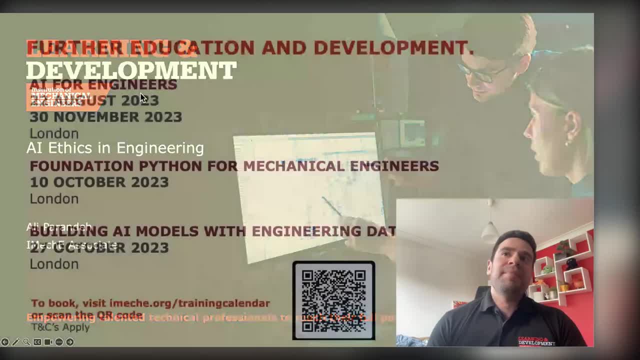 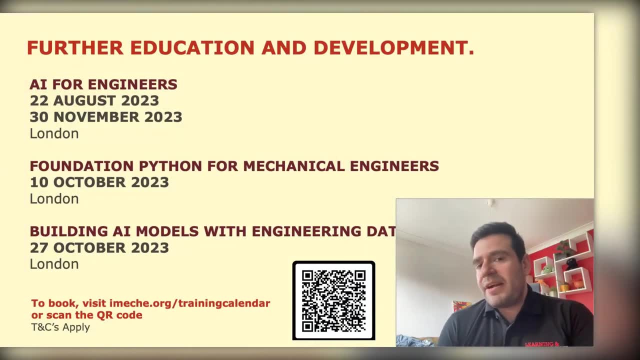 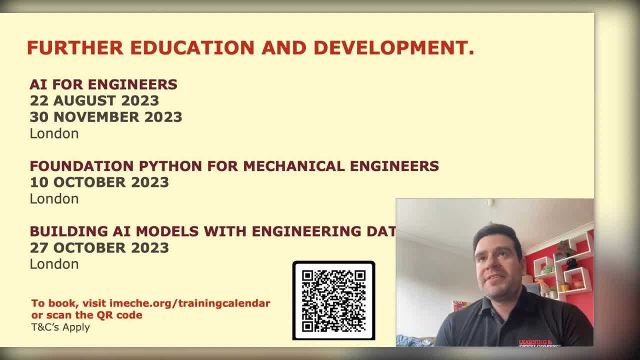 So let's get started. So let's get started. Just before I go into the webinar itself, we just wanted to mention that, as part of the IMechE learning and development training, we are releasing a set of new courses on AI that I will be delivering for you. So these: we have an AI for engineers course. 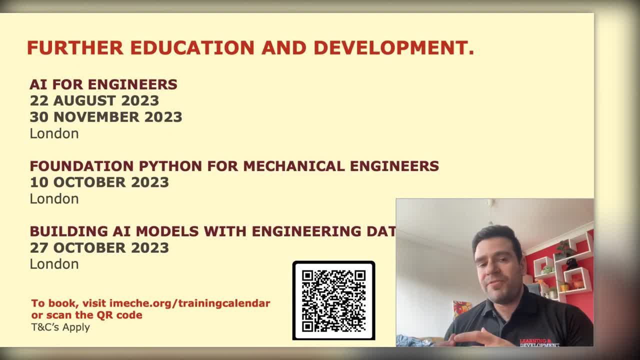 which focus on the non-technical aspects of AI and just provide an intuitive understanding and overview of the whole AI in the engineering context. So we're running the first workshop on 22nd of August. These are all full-day workshops, so there will be a lot of content. 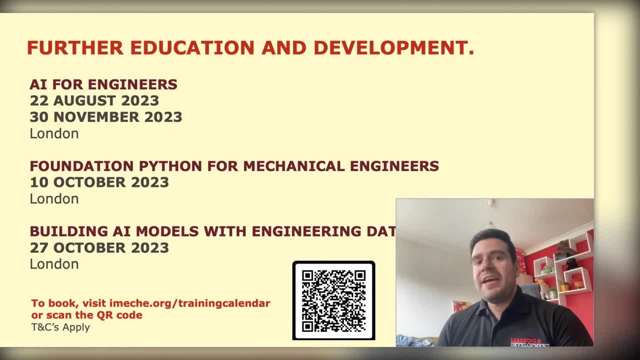 covered. So if you're interested in any of these workshops, you can use the QR code at the bottom to scan with your phone and go to those pages and have a look at the overview of what these workshops are. The foundation, Python for mechanical engineering and building AI models- these are all. 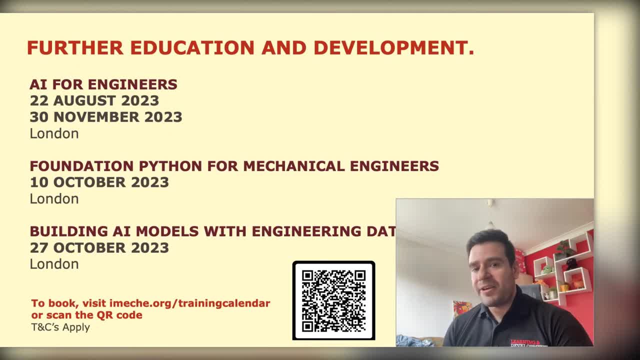 more technical workshops. So if you're interested in actually building these AI models yourself and learning a bit of programming, you can go to the IMechE learning and development workshop. So if you're interested in any of these workshops, you can use the QR code at the bottom to scan with your phone and go to those pages and have a look at the overview of what these workshops are. 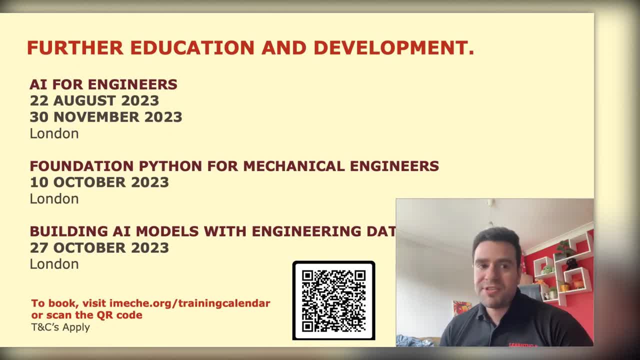 And on how to work with your own data sets in engineering, because you know, sometimes you can't just do everything in Excel. You need to start using Python a bit more if you want to get into building your own AI tools. We do have those two courses. They are all again one-day workshops. 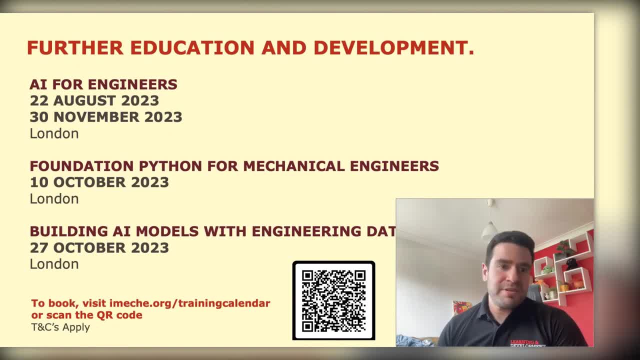 and you will learn quite a lot on those courses. So anything from software engineering practices to how you actually go build your own models and we're going to really play around with like latest AI technologies in those. So if you're interested on the commercial side, I would recommend the AI. 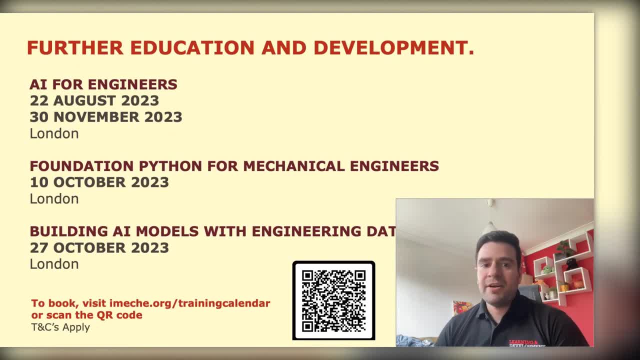 on how to scope AI projects and communicate AI and understanding the intuition behind it and the landscape AI for engineers. we've got two dates: 22nd and 30th November. Otherwise, the other two courses would be for you, So I'll just leave this for a second if you want to scan the QR code. Otherwise, 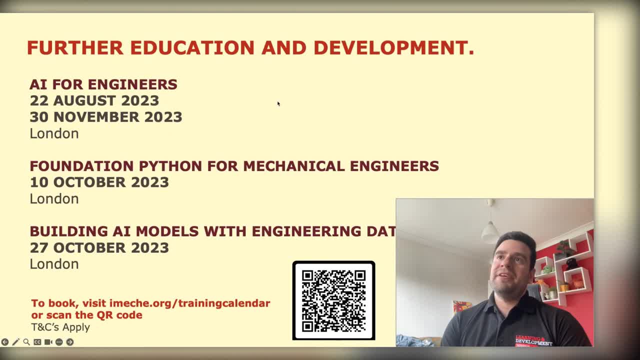 let's jump straight into the webinar, where we're going to be covering a few topics that might be interesting for you, And then, if you have any questions, please feel free to post them in the chat and then I will be trying to answer them with Dan at the end of the session in the Q&A. 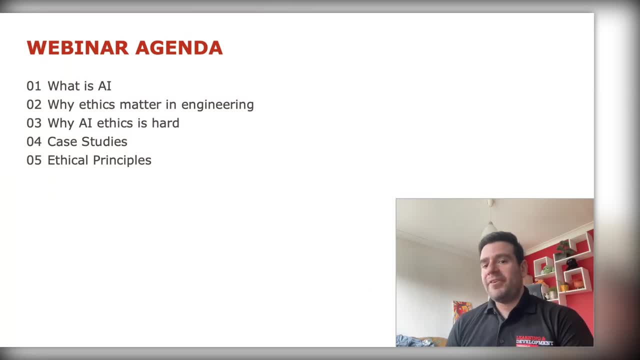 So today, what we're going to be covering mostly is five specific topics on the AI ethics Before we can actually delve into the ethics of it itself. what I'm going to be doing is just talk about what is AI. You might have heard of it quite a lot in different areas and on the internet. 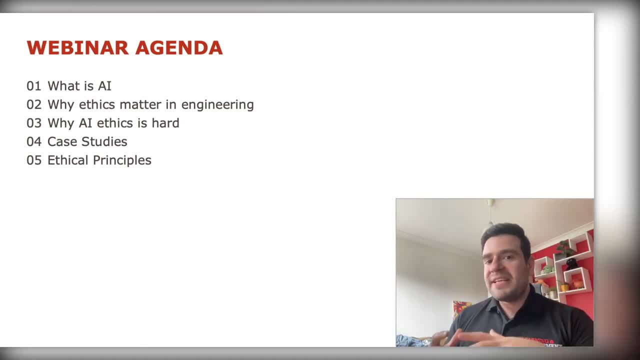 but what I want to do is just give a very overview understanding of what it is. So I'm going to start off by explaining what it is exactly, especially on the neural network side and more of the advanced techniques that recently come with the technology. Then we're going to talk about a bit: why ethics? 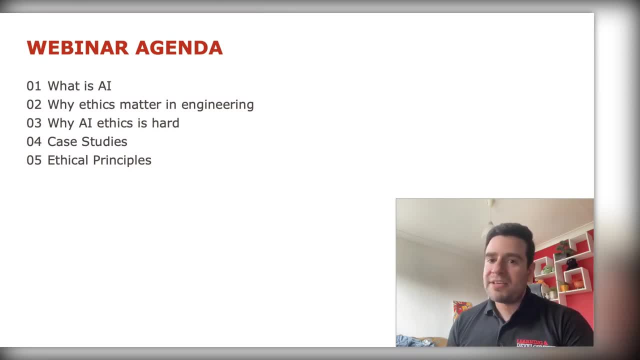 matter in engineering, and how does it then relate to AI, and why does it make it so hard to actually try to implement AI ethics in engineering or in general? just because, even if you really want to, there will be still bottlenecks and drawbacks and challenges for you? 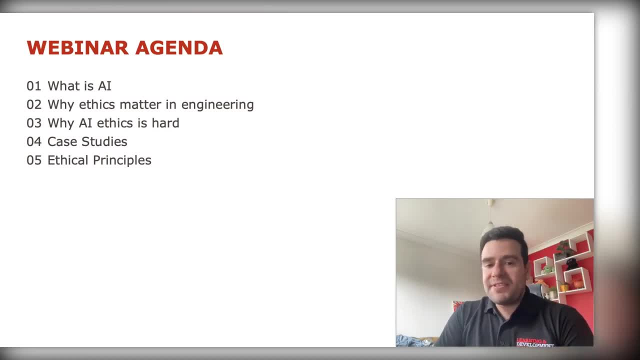 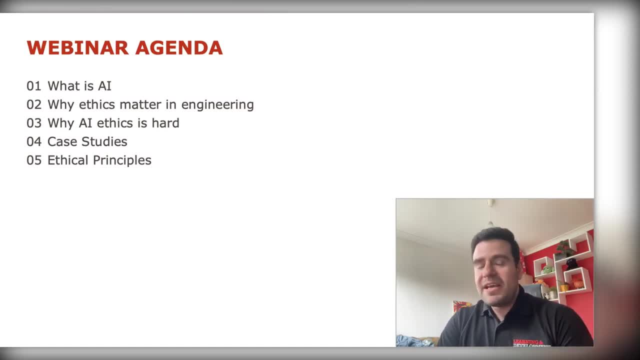 session is: I will have about five to seven case studies, depending on the time that we have. We will go through these case studies and I will give you some time to post in the chat your thoughts, what you think will happen, depending on those scenarios. So these are. 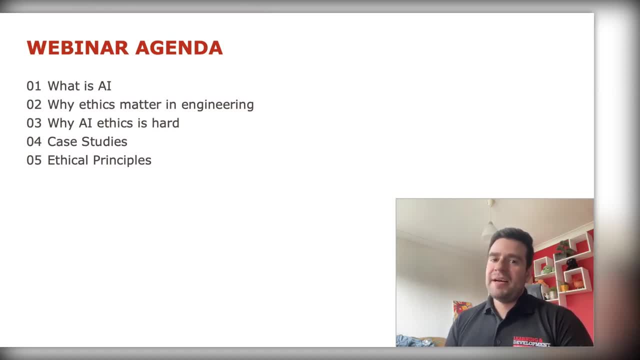 like more like situational judgment scenarios where you can think through what will happen if a company starts doing those things without considering the ethical aspects. And then at the end, I have two or three frameworks I want to show you. So one of them is from government, The other two are from Microsoft and Ethical Institute. 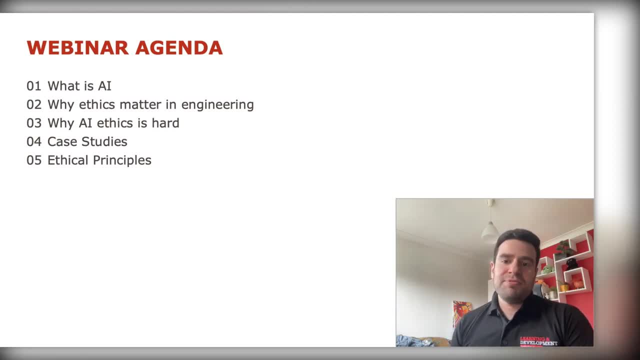 which are, I think, quite really good frameworks if you're trying to assess projects within your organizations against these ethical frameworks, so that you make sure that you've not missed anything when it comes to implementing and adopting AI in your own organizations. So let's jump straight in into the beginning of this. 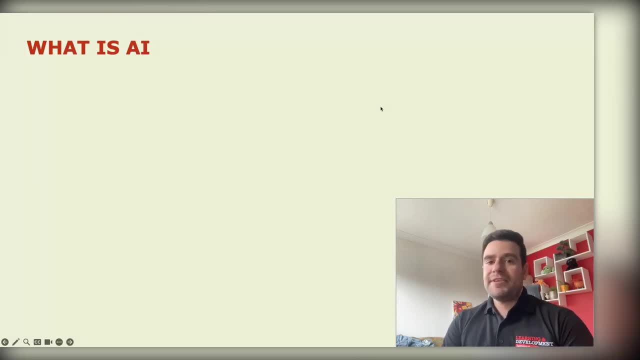 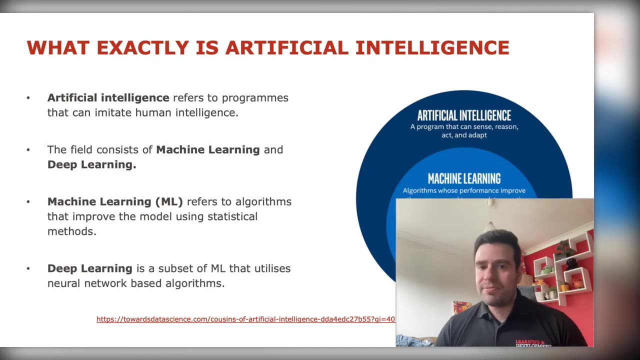 So the first section we're going to talk about what AI is. But overall, when we talk about AI we basically talk about any computer program and any application that mimics human behavior. So any program that can sense, reason, act and adapt similar to a human would, And it's a very 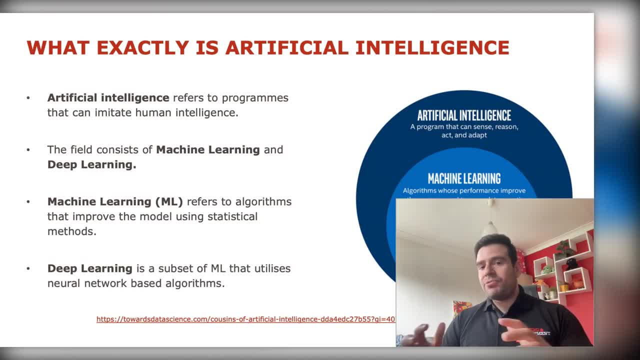 very broad topic And, to be fair, it's been around since like 1990s or since the computer, like the beginning of computer science. people were still really interested in it. However, it's not a very common topic And it's a very, very broad topic And, to be fair, it's been around. 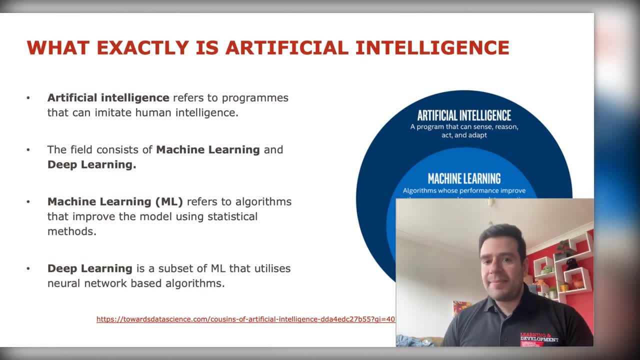 for a long time And it's a very, very broad topic And, to be fair, it's been around for a long time At the moment. at that moment, the algorithms and the applications were not advanced enough. The graphical processing units, the central processing units, all of these. 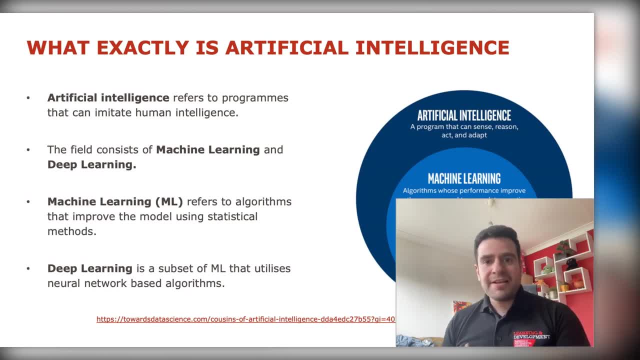 components of hardware were not advanced enough to actually catch up with those algorithms and performing the computation mathematics for it. So now it's such a big topic because the hardware has caught up to these algorithms and the algorithms at the Bastian level, where you can actually get performance. that is much better. 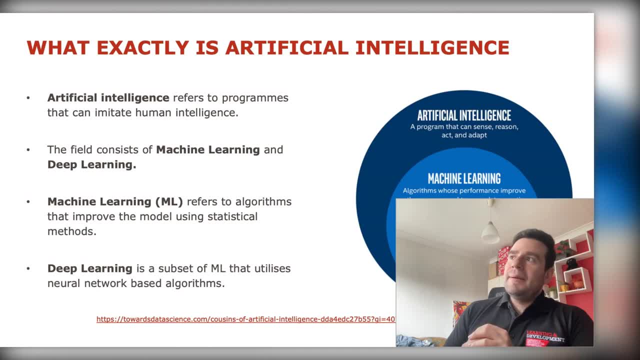 than humans in some aspects, And it's a very, very broad topic And, to be fair, it's a very, very Now this artificial intelligence discipline has come across, which allows us to build programs that can mimic human behavior. Now, a subset of that is machine. 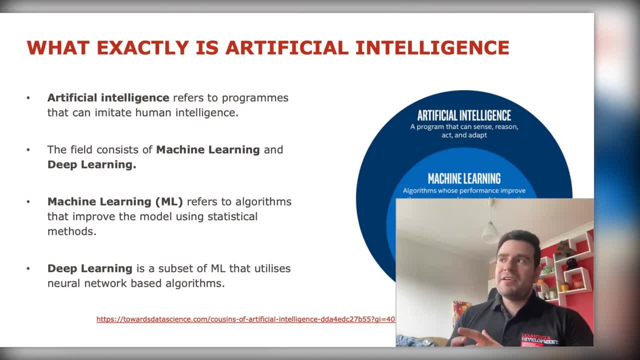 learning, which a subset of AI is machine learning that we might have come across. And when we talk about machine learning, we just talk about algorithms and techniques that use statistics under the hood to perform any sort of AI tasks, such as prediction, forecasting, classification. 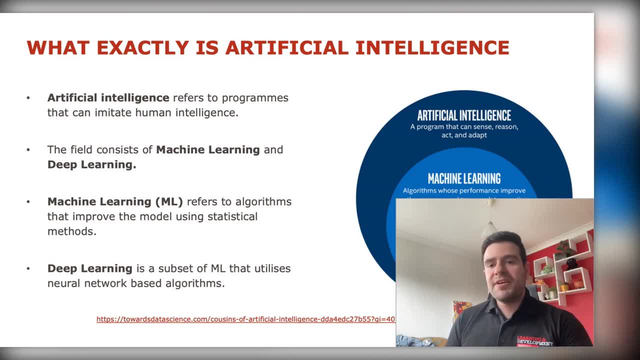 decision making, automation, optimization, optimization tasks, all of those things. So these normally use statistical models under the hood to perform those predictions and refers to algorithms that basically improve the model. that like creates those models based on statistical techniques. Now a subset of machine learning is deep learning. 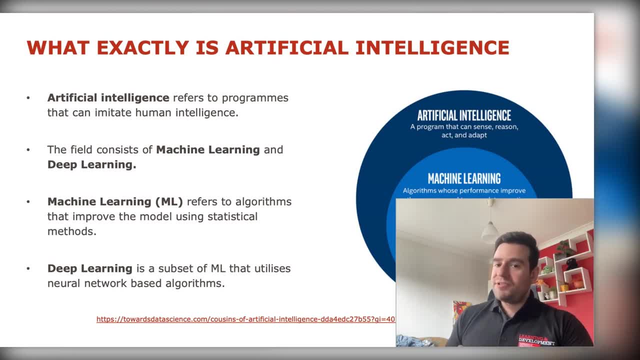 and deep learning is where basically all of these recent tools that you've seen, like ChatGPT and MeetJourney, where they can produce, or generative AI tools that can produce very, very human, very realistic items and like assets like pictures or text, those normally use deep learning and deep 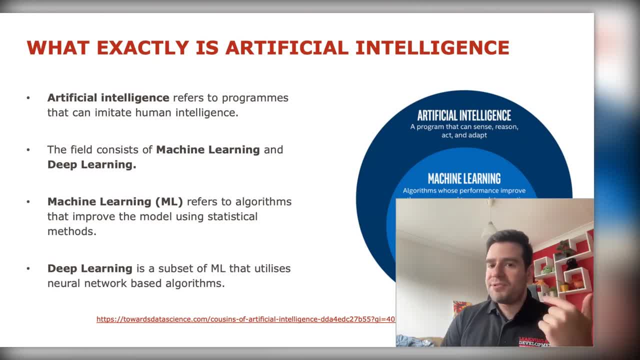 learning is inspired by how our human brains work and it's basically a mathematical representation of neural networks, which is basically how our brains work, but a very, very simplified way, and even with even the fact that it's a simplified mathematical expression of how our brains work, these can achieve very, very good results to the extent. 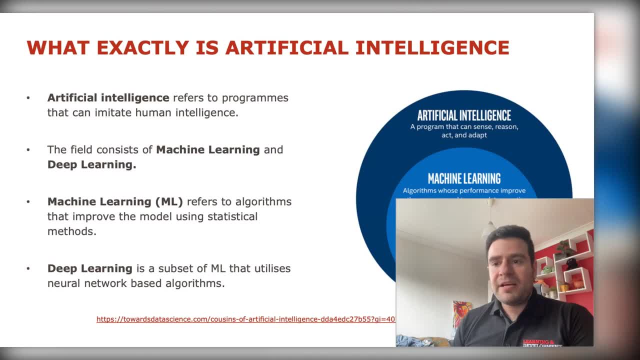 that, like. sometimes it can surpass human performance- and that's why it's such a hot topic- and you can actually use deep learning now, these days, to perform tasks that humans would probably miss or there is a human error in those situations. However, with AI overall and machine learning and 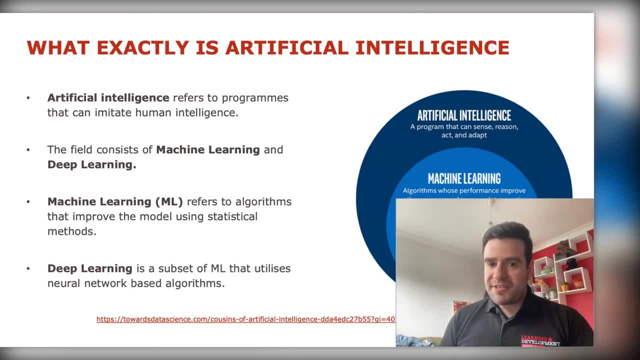 deep learning. these are all probabilistic models, they are not deterministic. so because they're like 100% chance that something, the outcome is always 100% or the accuracy is always 100%. so because of that there is always going to be ethical implications when it comes to. 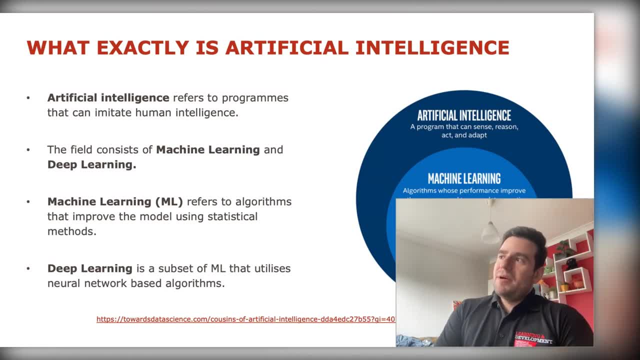 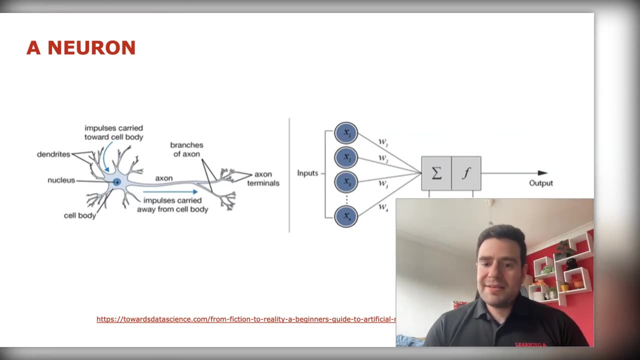 building and working with these models. but because today's webinar is more focused on the AI ethics, normally those come from the deep learning area, and when we talk about deep learning, we talk about a mathematical representation of human brain. Ali, sorry, Dan, here just to jump in. you might want to turn your camera off because it's covering a lot of the screen. 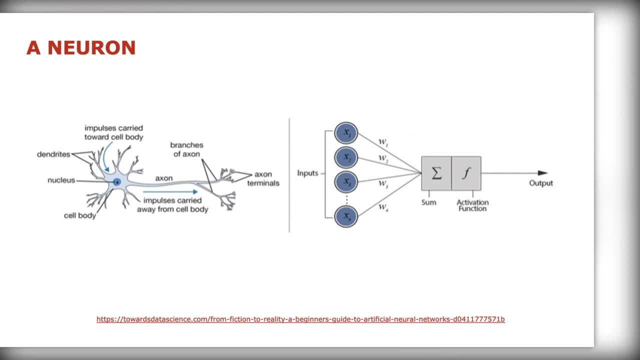 Oh, yes, yes, we'll do Sorry about that. so basically, today, when we talk about deep learning, we talk about a mathematical representation of human brain and neurons in particular. so neurons are just basically cells in your brain that activate depending on the signals that they receive, and 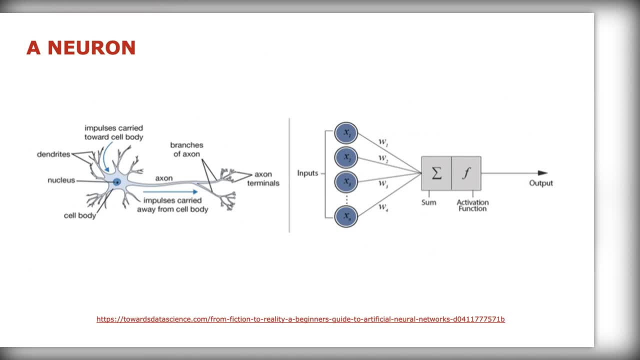 if this signal is above a certain threshold, they fire to the next neuron. So basically, what we're talking about is a neural pathway and these neurons together firing will cause a pathway or a neural pathway that creates the this, basically the neural pathway that helps you learn a skill. so for 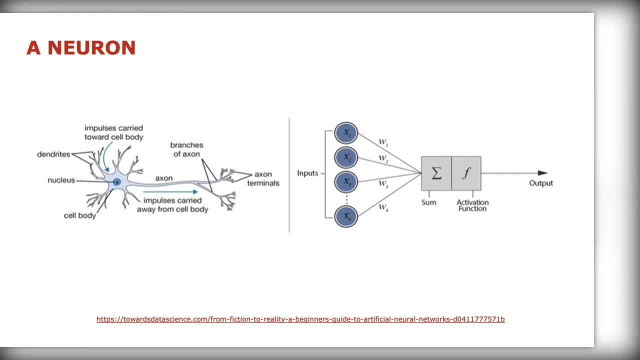 example, when you learn a programming language or you learn to play with piano or you learn like a mechanical engineering concept, these are specific neurons in your brain firing, creating certain pathways that like, solidifies that skill in your brain and in that specific set of knowledge or skills that you need to be able to use in order to be able to use your brain in the right way. 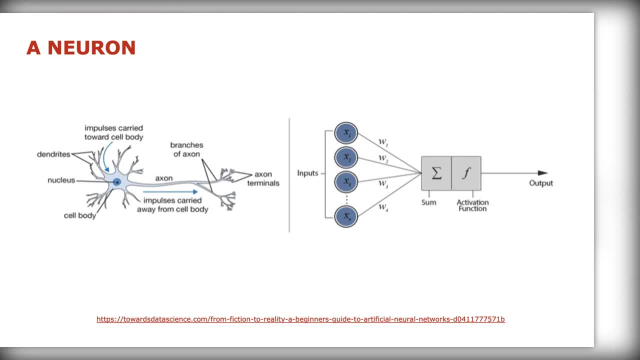 So basically, what we're talking about is a neural pathway, and this can be modeled mathematically with a bit of a simplification, using the mathematical model on the right, where you take a series of inputs multiplying by the weight set of weights, then you sum them together and apply an activation. 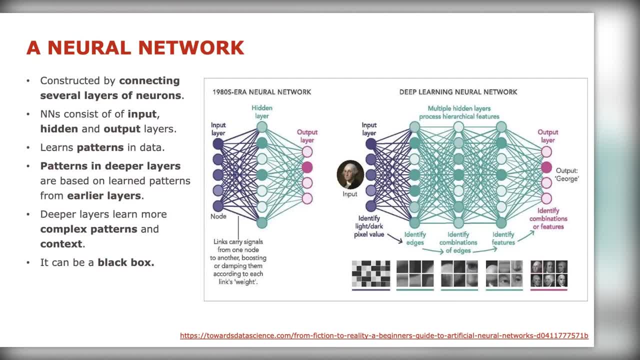 function on top to introduce non-linearity to the model. and when you connect these neurons together, you get these neural networks that can achieve outputs that are basically the interactions of these neurons, and these outputs are quite complex. so the way it works is when data flows from from one side of neural network to the other side, the neural network. 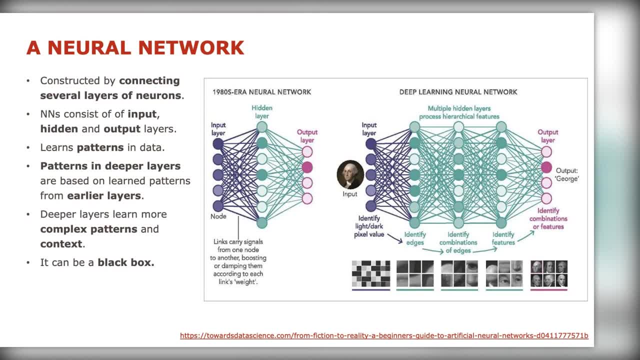 starts learning patterns in the data, from the basic patterns at the near the input layers all the way to the more complex patterns and the decision making abilities at the output layer. So a neural network normally is just constructed by connecting all of these neurons together. so when you connect layers of neurons, 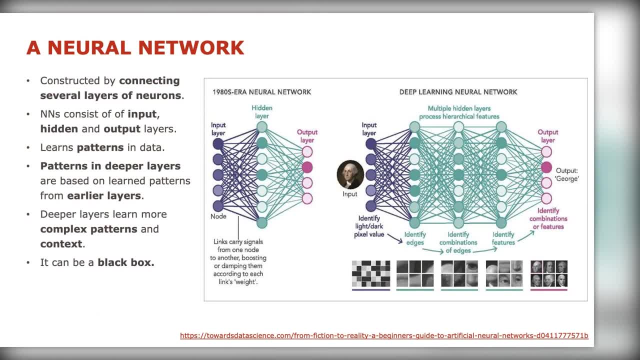 together you end up with a neural network, and neural networks normally consist of a series of layers, three of them, that are most. we classify those layers as our input layers, hidden layers and output layers, so any layers in between are in hidden layers and any layers at the beginning and 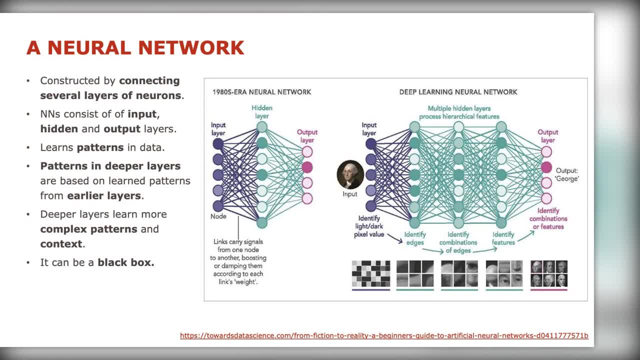 at the end are input and output layers. so what these neural networks do, because of the way they work mathematically under the hood, they learn the patterns in the data. that's basically what they do when they're connected to the neural network and then they're connected to the input layer. 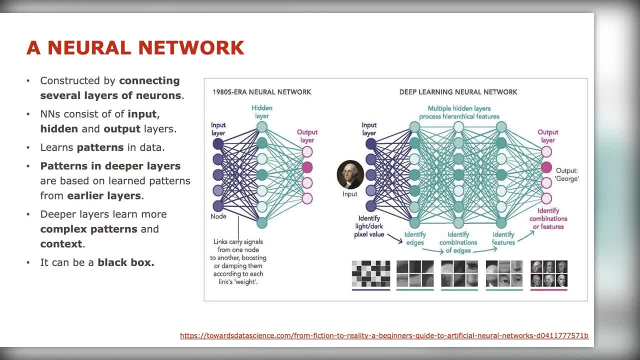 so then you pass your data through them and the network figures out itself by adjusting its ways and biases to basically connect the patterns in the input data to the patterns in the output that you expect from the network. so, for example, in this picture in, in this example on the on the slide, 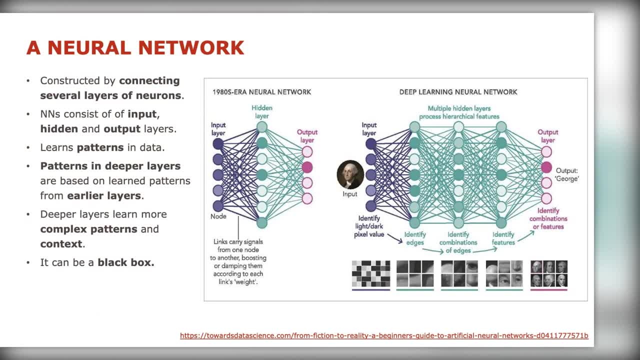 we want this network to predict who this person is. so what the network is doing is as that, as the picture is basically going through the network from left to right, the network is learning simple patterns in the data, such as, for example, the edges, vertical edges, horizontal ledges, diagonal. 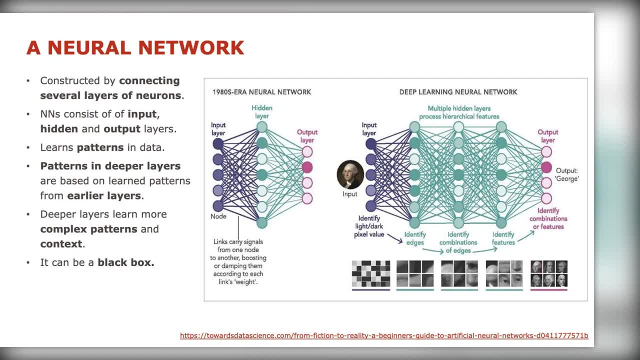 edges, and then it combines the edges together into patterns like shape of shape of an eye, shape of a nose, shape of a face, and then those then come back, get combined together into understanding visual patterns of what um like, for example, george washington's face looks like, or what 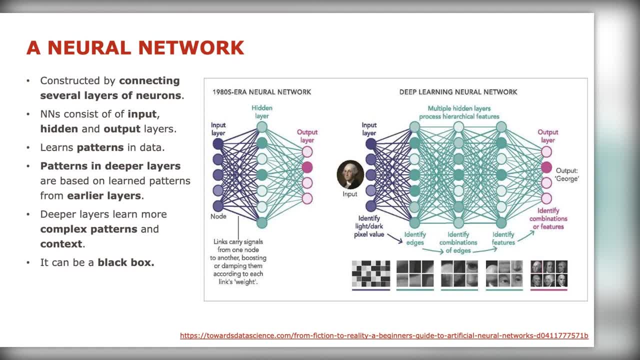 obama's face looks like, and this specific property. you can also use it on any of the other applications, any other application that you have- imagery data, for example, in a manufacturing environment, you can make. you can help it to learn patterns in defects of products and then, once it learns those patterns, you can then use it to identify if there is any faulty. 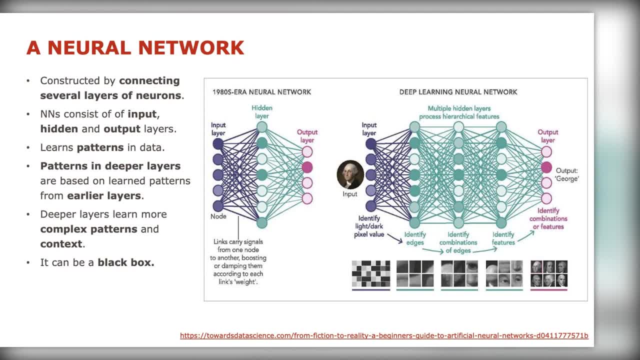 items on the on the product line, as long as you have enough data for it to learn those patterns. so as you go deeper into the neural network you start the network starts learning more complex patterns that it learned from the previous layers. the thing here is these neural networks especially. 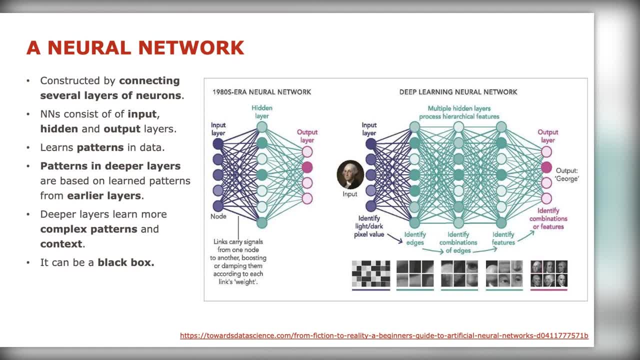 the bigger they get and the more complex the architectures become. they are like mathematical black boxes. basically, they're just like a function, but they are such a complex function that you don't know what it's doing under the hood. you don't know how the data is being wrangled and mathematic. 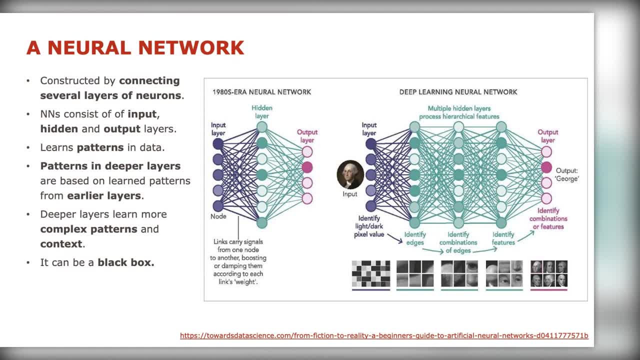 how the mathematics work inside these neural networks for us to fully understand what's happening. and sometimes the outputs make you feel like you're getting a good model but under but that model, when you put it into the actual real world scenario, may not perform as well. so even though it performs well in the testing scenarios, it may not perform well. 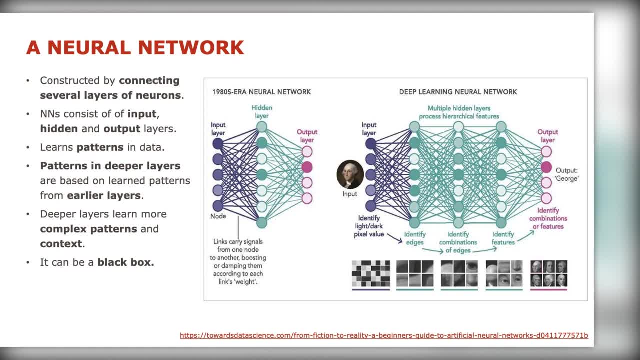 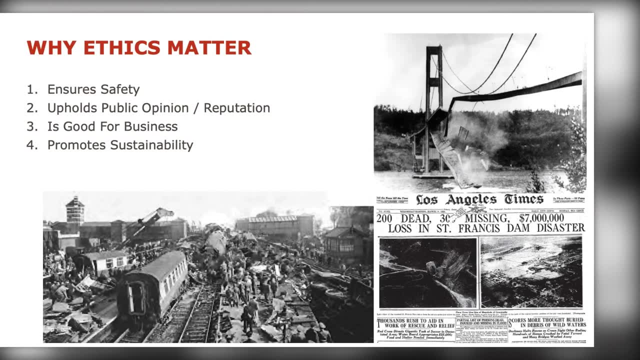 in the actual real world scenarios, because it's such a black box and that's what is causing the ethical issues. so, when it comes to ai, ethics itself- and what one thing i want to talk about is the ethics itself- is very important because of four main reasons. so in engineering, we were 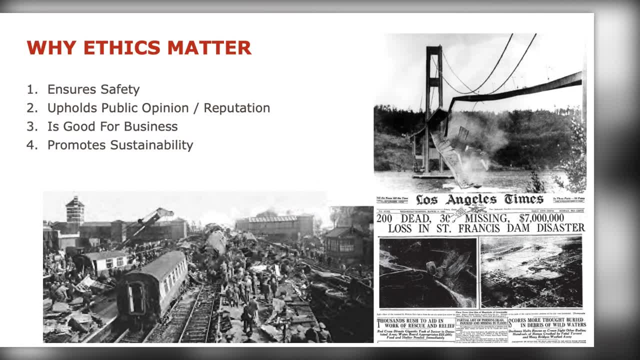 always really concerned about what was going on in the real world and what was going on in the real world, and we were very concerned about ethics. it's actually one of the main competencies of engineers, like competency e of uk spec is all about ethics, safety and sustainability. the reason 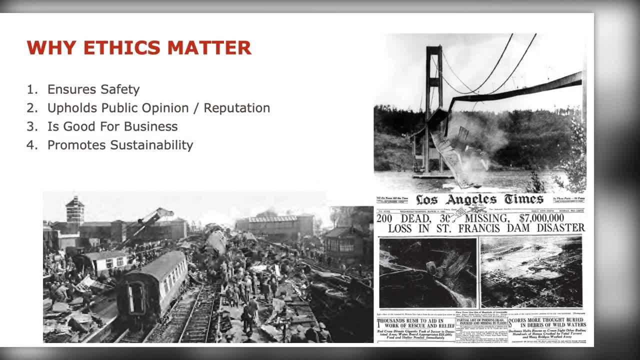 is engineers. if they make a mistake, a bridge can break, a building could fall down and there could be a train crash. um, lives could be lost. so it's very important that we are all ethical and um, and it ensures the say. when we are ethical, as part of it, we ensure the safety of anyone. 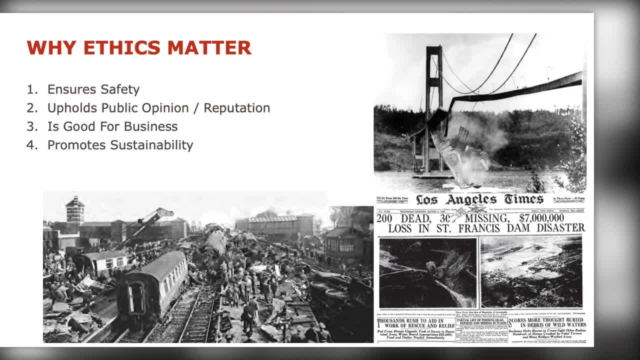 who's going to be interacting with what we build. The other thing is when we are ethical about our profession, it upholds public opinion and reputation of the engineering profession And because of that any business that upholds a professional opinion gets more business. 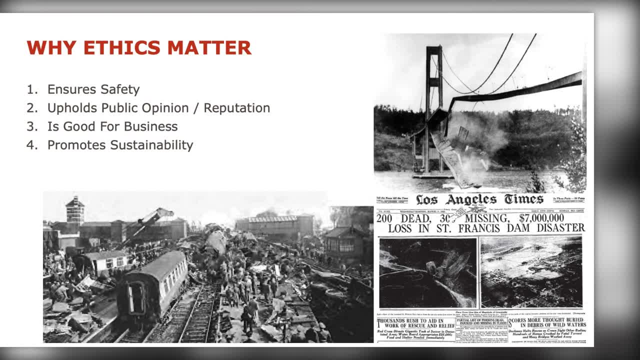 because people and companies trust people and other companies that are ethical and they do things by the book, And because of that it's also good for business. So it's one of the main reasons why we should be ethical. And the other thing is it promotes sustainability. So when we 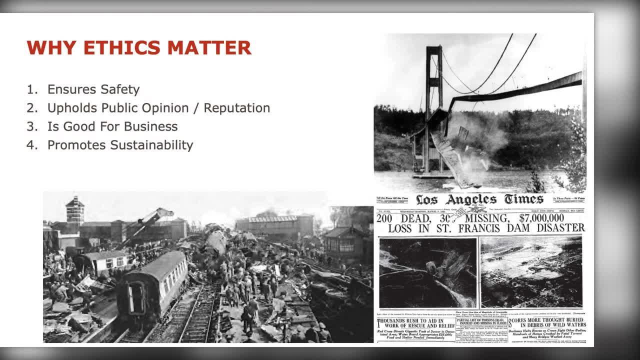 consider all the aspects of what we're building, from the sustainability, environmental aspects and from anything else. we help advance the engineering profession and all the aspects of it also, at the same time making sure that we keep the environment in the same place that we left it. 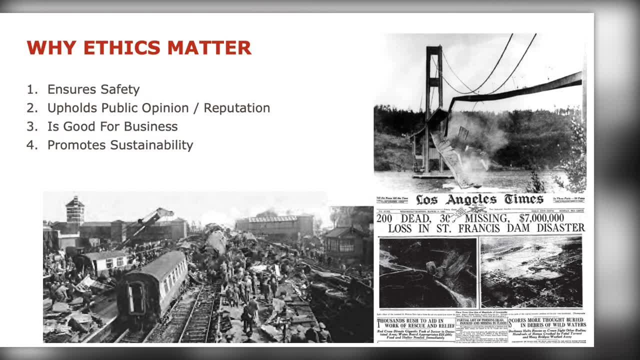 and, of course, at the same time, we're providing value to the society. So, because of these four items, ethics is very important, And it matters that everything we do is ethical, including any innovative projects that we work on, And some of these projects may include adopting AI. So we need 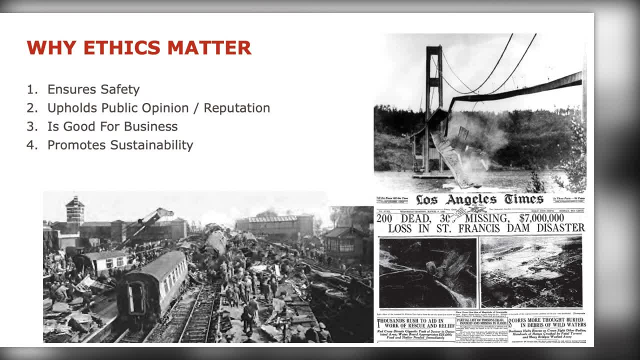 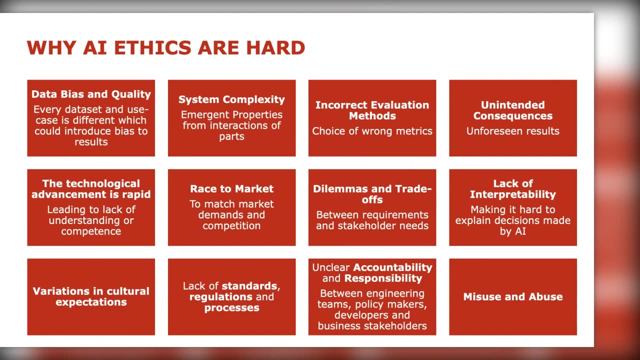 to be also worried about the ethics and the safety of any AI system that we build. because of these four reasons, However, it is actually quite hard to do that. So, because of all of these reasons, on the on the on the slide today, it's very hard to implement. 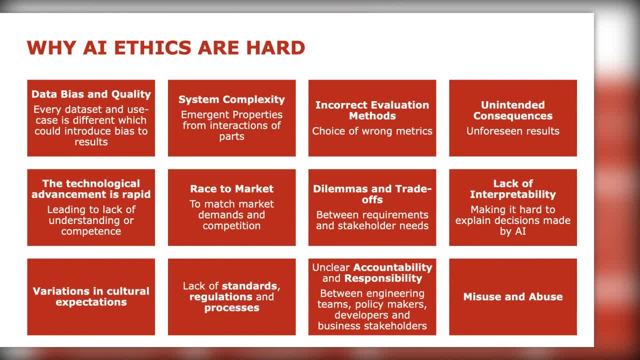 AI ethics and to follow these principles. So let me start from top left all the way to the bottom right and explain them why. So one of the main reasons it's hard to perform AI ethics is because of data bias and quality, So every data set is different, And some of the data sets that you 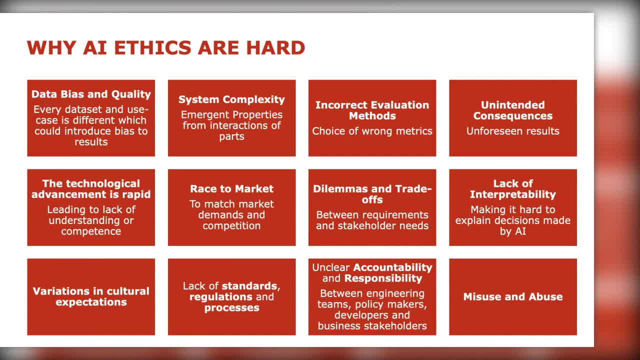 will collect or measurements field. measurements that you collect from real world scenarios could have bias in them, And bias could be the fact that the data sets that you collect could have bias in them, And bias could be the fact that the data sets that you collect could have bias in them And bias. 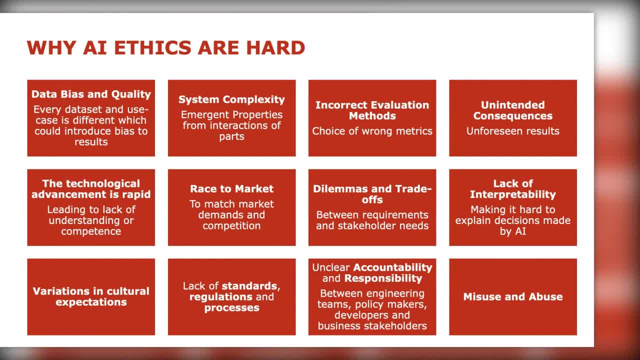 could also be introduced by all sorts of variety of places with variety of factors. It could be introduced by algorithms that you use. The bias could be introduced by the fact that there is bias already in the real world environment that you're collecting data from. You may inadvertently 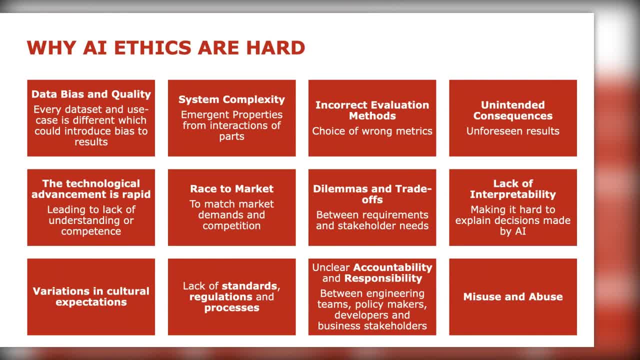 include bias by the way you sample your data for your, for your modeling techniques So, and the quality of your data may not be good enough to build AI model on top, And because of that, there is always data and bias and quality issues that will could be present. 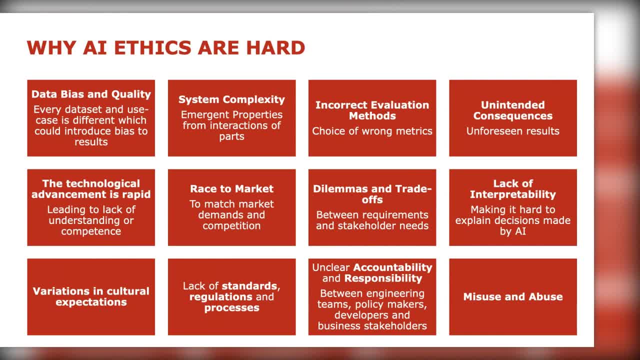 that will prevent you from building AI models and AI systems that perform well and in an unbiased matter. So because of that, it's very hard. The second one is the system complexity. So neural networks are a complex system just because a neuron by itself is easy to understand. However, 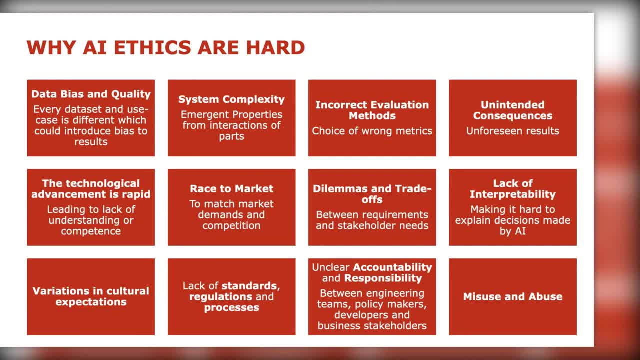 when neurons connect together and interact with each other, especially if the architectures of these neural networks are complex, they create emergent properties. So these are properties that doesn't exist. They are not possible to be understood by their individual components alone. They exist because 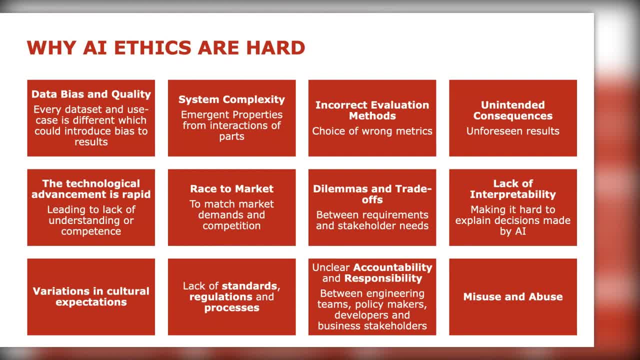 of the interaction between these individual components, And because of that, it's very important to understand what our AI models are doing, layer by layer, and understand the mathematics inside these models, And there are actually lots of movements around AI explicability and transparency when it comes to building AI systems, and that's why it makes it. 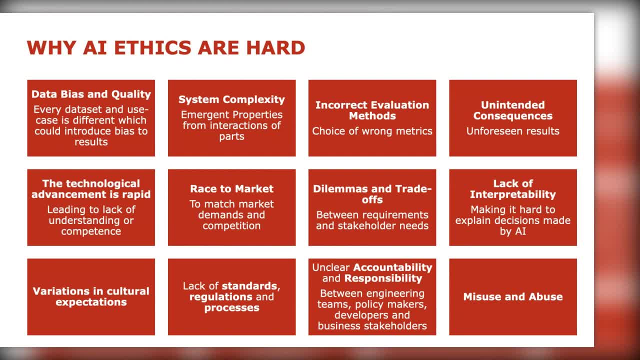 complex. The other thing is lack of understanding of what the problem is. So if you don't understand what your problem you're solving, you may end up choosing wrong evaluation metrics and testing metrics on your models. When you do that, you think that your model is 99% accurate and you basically put your 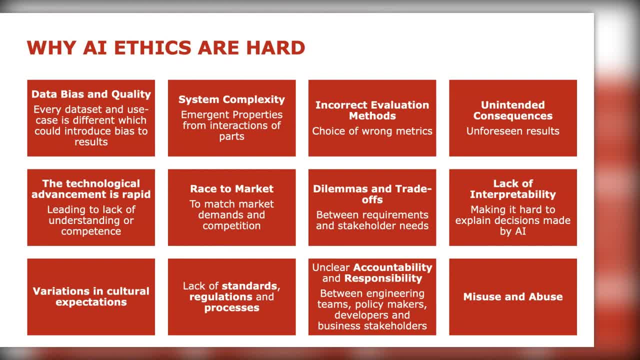 model into a real-world environment, whereas in the real-world environment it may not perform at that level because that metric that you used to evaluate your model was not the right metric. So it's more: it comes down to the understanding of the metrics that you can use to evaluate. 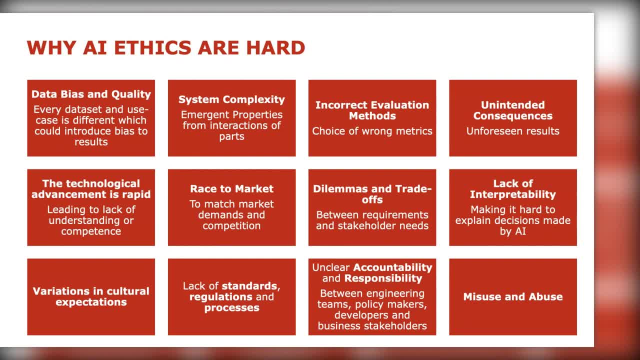 your models at the end and test them versus the problem that you're trying to solve, And we will have an example on this in one of our case studies to help this understand a bit better. The other bit that makes it difficult is unintended consequences. 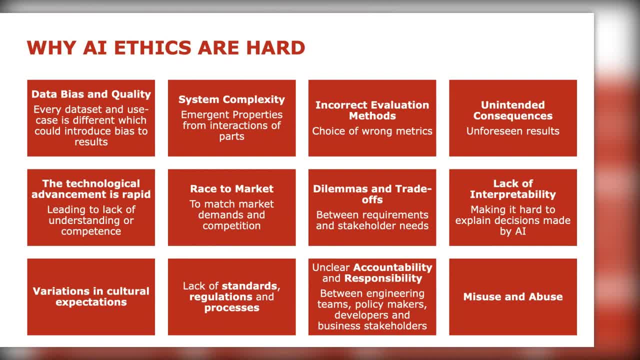 So you may build something but then put it into a real-world scenario to start using it and you've never considered how people may use it and how it may be used in production and it may create unforeseen circumstances. So it's always part of innovation. 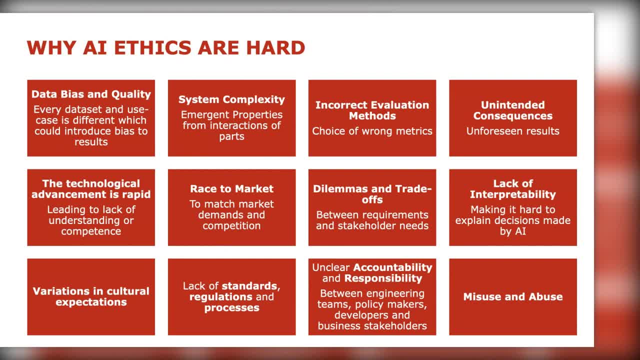 Because it's just a new thing. there is always elements of usage that you've not considered or misused. So this kind of relates to the last item down there, misuse and abuse as well. Engineers may not necessarily understand all the various scenarios that someone may use. 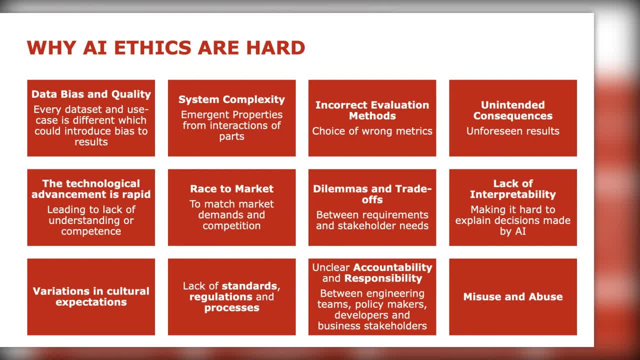 these new innovative tools and it's very important to have done a proper risk assessment before any kind of AI system goes into real-world use. Last, one of the other items that may be important is that you have to have a proper risk assessment. 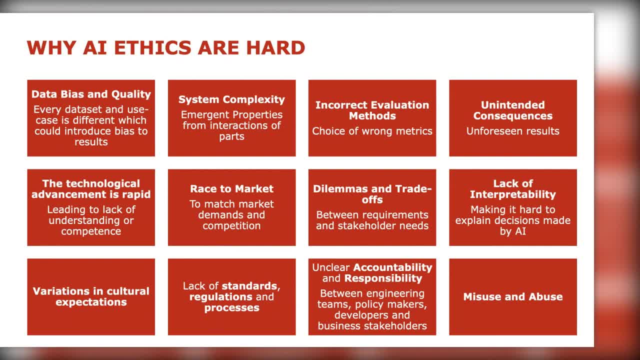 What makes it really difficult to comply with AI ethics is technological advancement. It's so rapid that by the time that the organization starts to understand certain techniques and algorithms for building AI tools, a new algorithm has already come out. At the moment, the current rate of release of AI papers are about 100 a day. 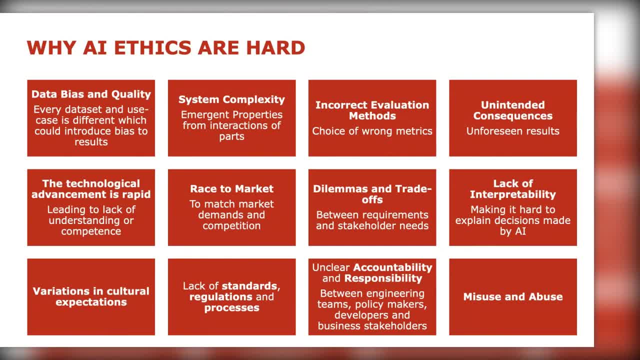 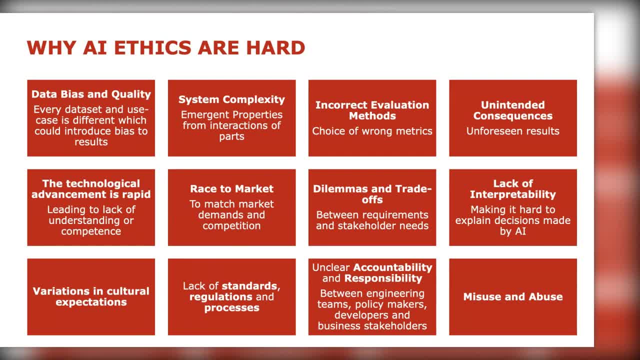 with the introduction of attention heads and all of these ChatsGPT, large language models are becoming more obsolete and they don't matter as much because of these new techniques that came out. So if your organization spends all of that money building AI tools based on those algorithms, 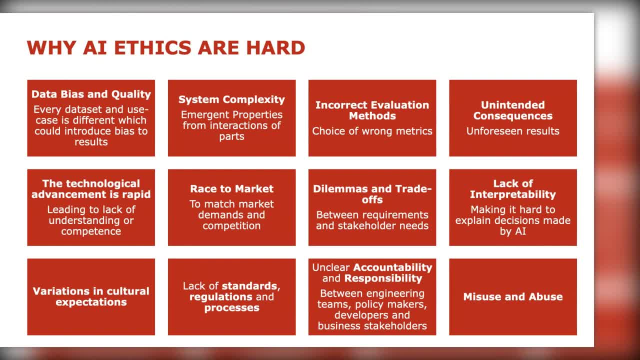 it may not be relevant anymore, because better algorithms now exist, And those new algorithms may not necessarily be the best still, but they could have their own implications when you use them, So you have to understand them again. That makes it really hard as well to comply with AI ethics. 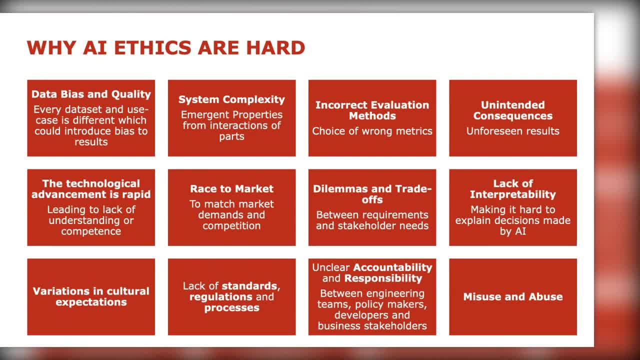 there is pressure to race to the market, so you want to release your models, but at the same time you want to be ethical. but there is this pressure to release the models on time so that you'll be faster than your competition, and that may cause ethical issues and ethical concerns there's always. 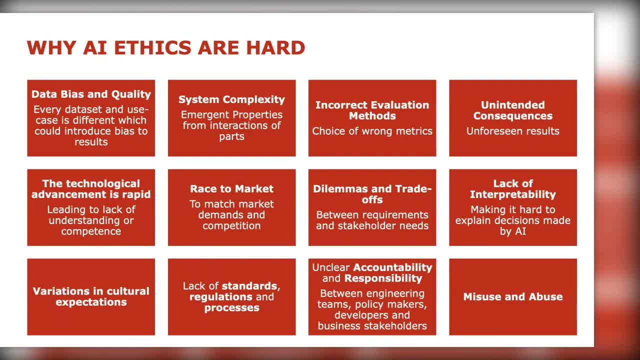 trade-offs, dilemmas between requirements and stakeholder needs, as well as issues around understanding and interoperability of of what you're building. so it's hard to explain to the business why an AI model is working the way it is just because of the same thing I mentioned. 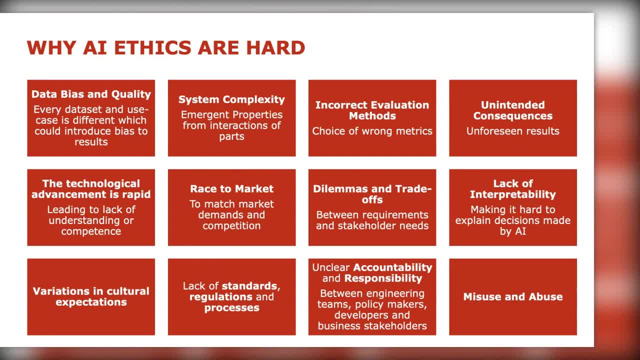 because of the system complexity and the fact that it's quite hard to understand how the model is making those decisions. how is it taking the data learning patterns in it and then making a decision based on those learned patterns at the output layers? when we talk about deep learning, 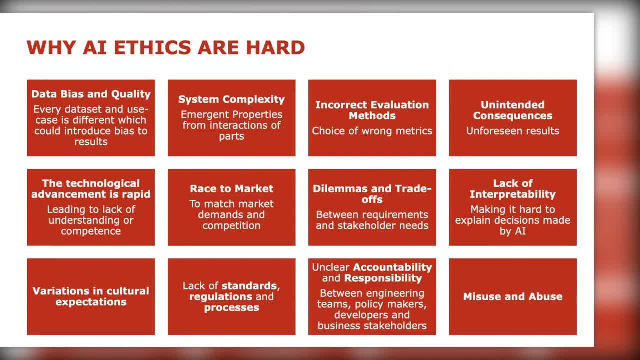 for example. so it makes it quite difficult because of that to understand what it's doing, and there are lots of new frameworks and techniques that came out um a xai, explainable ai- and, like all the other frameworks, tools, that allows us to now debug our neural networks and our ai models at like, lower levels. 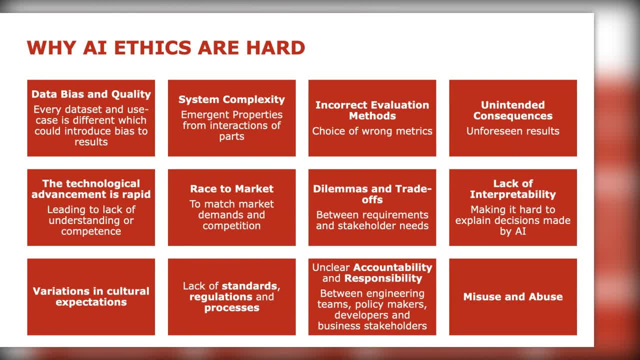 but still, it's still an area in development and um, if you don't really understand fully how our black box models are working in um in our testing area, we should be very concerned and we should always be very cautious how we start using them in real world scenarios. the other issues are: 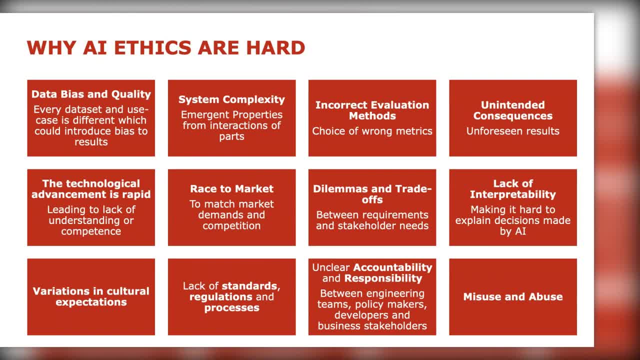 variations in cultural expectations. um, so this is a bit hard to provide examples for, but some outputs from ai models may not necessarily cause concern in certain cultures, whereas in other cultures it may be very sensitive. um, normally things to do with racial issues and things like that come into play here, but it could also be applied to engineering. so how it performs. 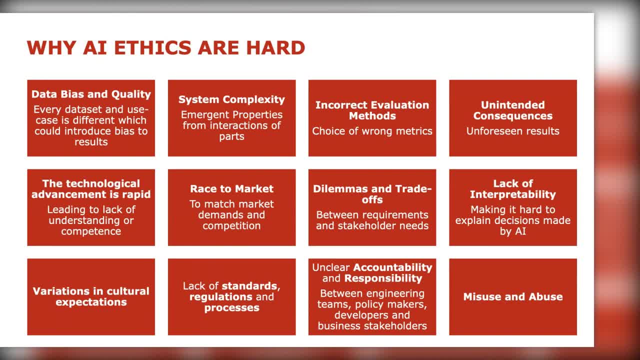 in engineering context, in different cultures and different countries may have different implications, so you always need to make sure that, like, even if they're performing well, the cultural expectations do also align with what the objectives of the organization are in relation to performance of these innovative ai systems that we're going to be building. another issue: lack of 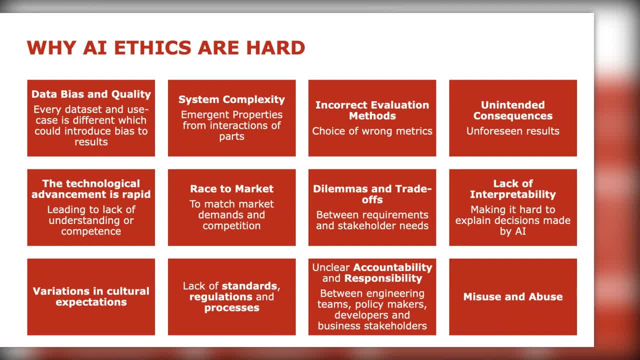 standards, regulations and processes. pretty much most of engineering projects these days have lots of standards, so you always have standards you can follow. it's part of the requirements of projects, well understood, you can just follow them and it's a it's basically if you've done it, you're kind of 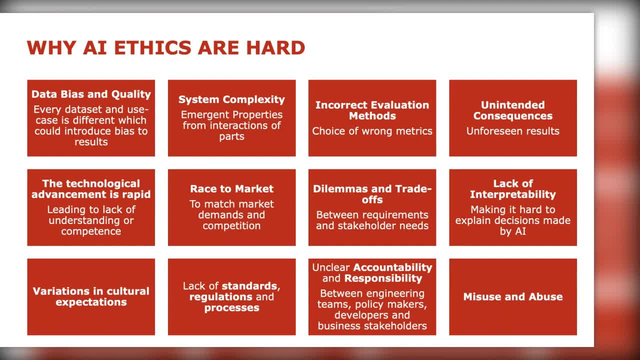 sure that it's, it's going well, but if you've not done it, then like you need to do it and basically projects don't go into uh, into an actual production environment, without those standards having been met. however, the problem is we don't have those in ai and because of 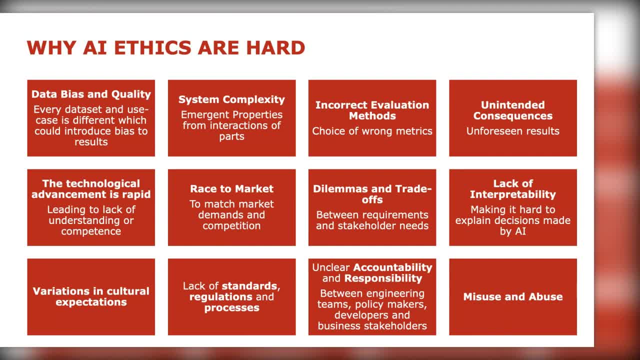 this problem. because of these reasons i've mentioned, it's hard to build the standards. there's just not enough examples, there is not enough uh data and past experiences to build a standard for long- short-term memory networks. so we need to build a standard for long- short-term memory networks. so we need to build a standard for long, short-term memory networks. 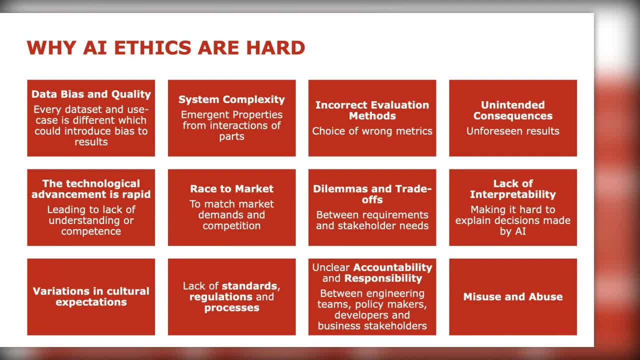 and because of this still like it's quite hard for the legal systems and for regulation system to catch up with the advancements of the technology that's coming in if someone starts building a standard for long, short-term memory networks now that the chat gpt llms are out- large language. 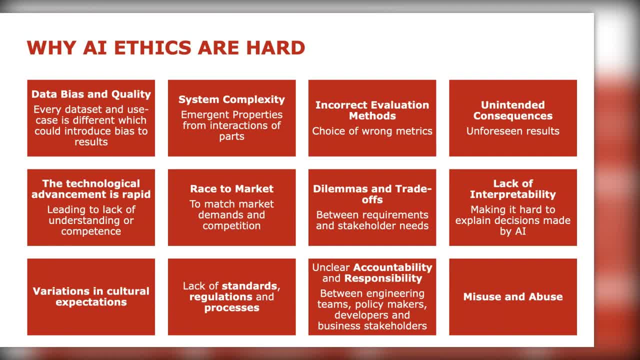 models. all of those should go out of the water because people now start using chat gpt's technologies instead of lsdm technologies, for example. lastly, it's accountability and responsibility. sometimes it's hard to define responsibilities and accountabilities in projects- ai projects, between engineering teams, policy makers. 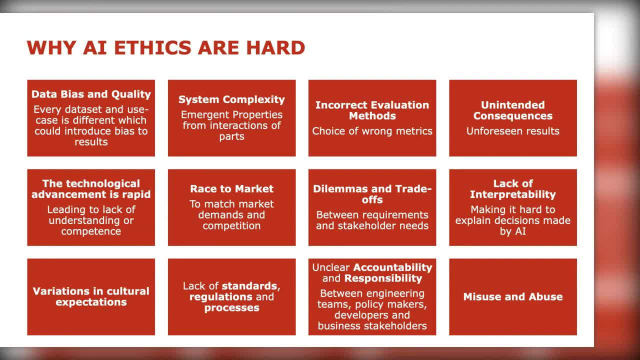 developers and business stakeholders, and if something goes wrong, it's kind of hard to understand who is who is responsible for it, like who must sign a sign off a set of outputs and deliverables on an ai project, because these are novel projects and their scoping might be different. 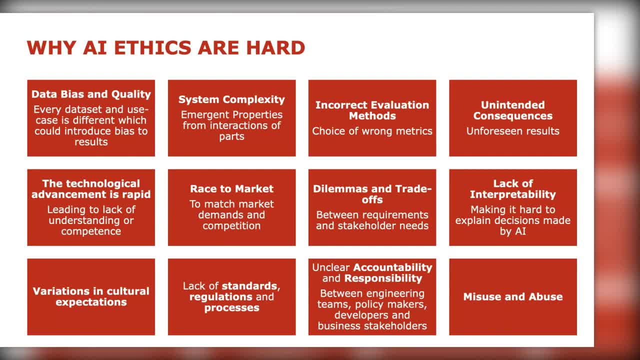 compared to traditional software or traditional engineering projects. it's also hard to define accountability and responsibility demarcation points and because of these um, it makes it quite difficult to comply with ai ethics, and that's what makes the problem really hard. so we do have a quite um. so dan has a poll for us to do, because on these and what we want to do is understand what- 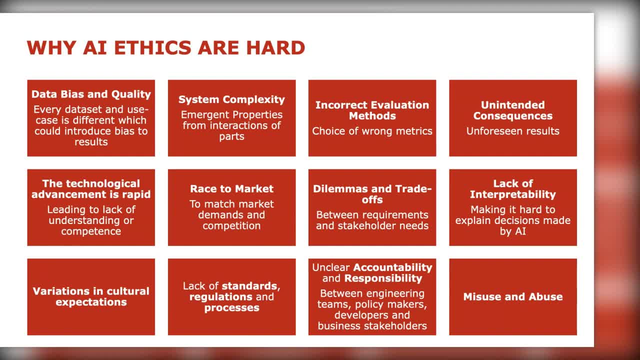 you think is the most important issues around ai ethics based on these elements. so, and then, if you can share the poll, and then we can have a chat about what everyone thinks are the most pressing matters when it comes to building ai systems in engineering. okay, yeah, thanks, i think we're just going to get it set up and it should be landing onto your screens. 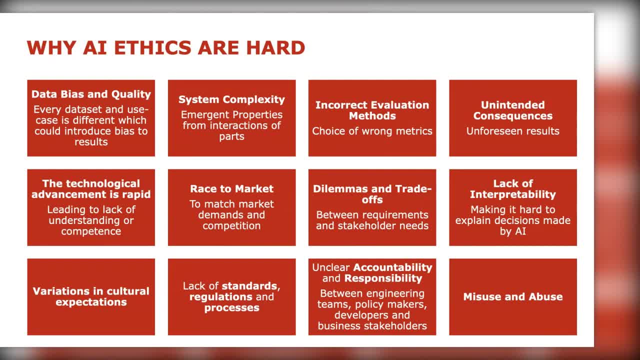 um, right about now, we'll just give it a few more seconds to so we can gather these poll results and then we'll post them. okay, let's, let's get the results in. okay, let's, let's get the results in. okay, let's get the results in. 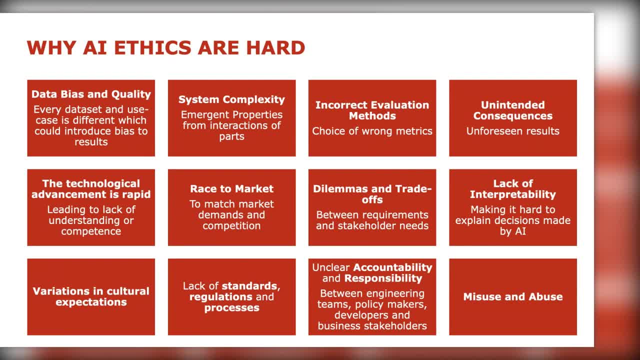 let's get the results. and, ali, can you see these results now appearing? just say, if not, i'll read them out to you. okay, i can see the results. uh, maybe uh, publish them to the audience as well so they can see them. yeah, i've published them. they should be able to see them as well. excellent, 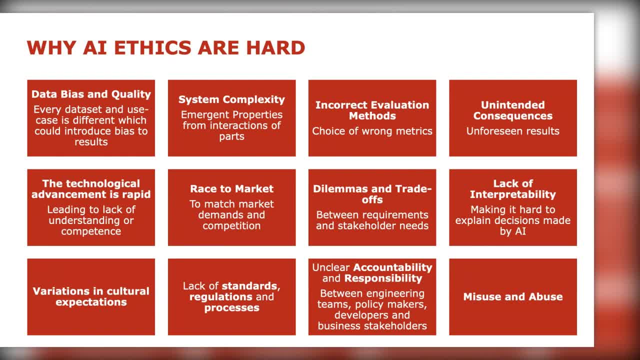 Wow. So this is a very interesting pie chart. Pretty much it's like a quadrant. So we've got lack of standards and regulations at the biggest, 33%, Bias and data quality issues at 22%, System complexity at 21.5% And then lack of clear processes at 23%. 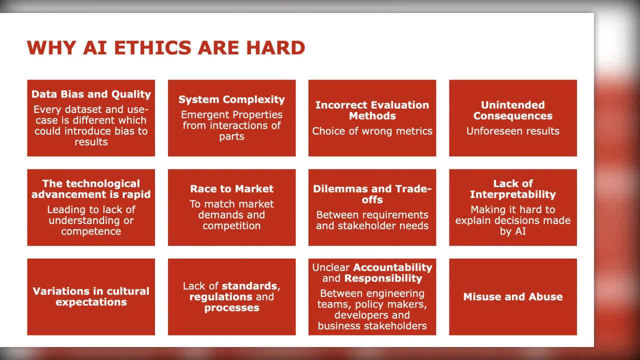 So it's pretty much all across the board, With lack of standards and regulations at the highest, And then technical issues, which is the red and yellow Bias, and system complexity. They take the other half of the pie chart. So I think, based on this, the problem is very complex, Just because it's both across the technical side and the commercial sides. 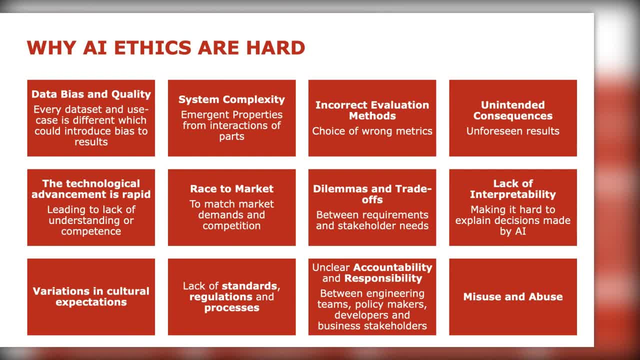 And non-technical sides. That makes it very difficult to understand the AI ethics. So I think with the standards and regulations, it also the fact that they're hard to produce and there is not many of them, it's because of the technical side. 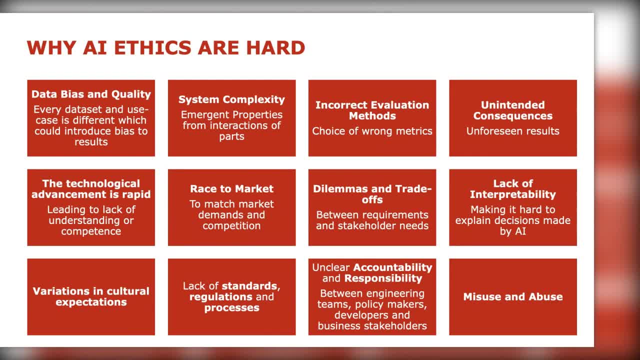 So the more people understand how AI works and the more people understand how the neural networks works, the more people can help with building the standards. There are already efforts underway, But when the standards come, they would provide the frameworks And they make it much easier to tackle these problems as organizations. 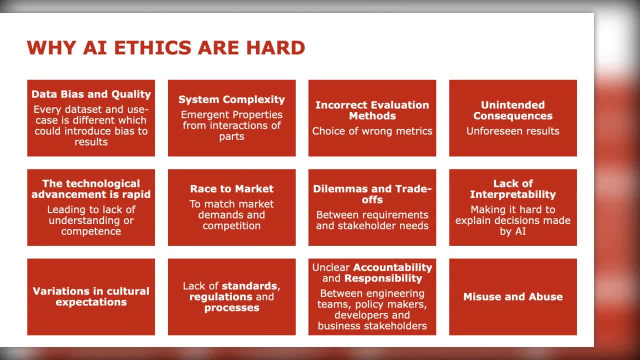 However, because there are not a lot of innovative projects on AI in existence And because these technologies are so complex and they're just moving so fast, it makes it really difficult. So it was a really good understanding that this chart is kind of like into a quadrant right now. 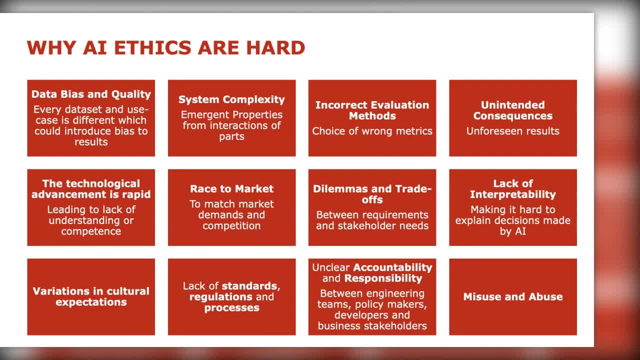 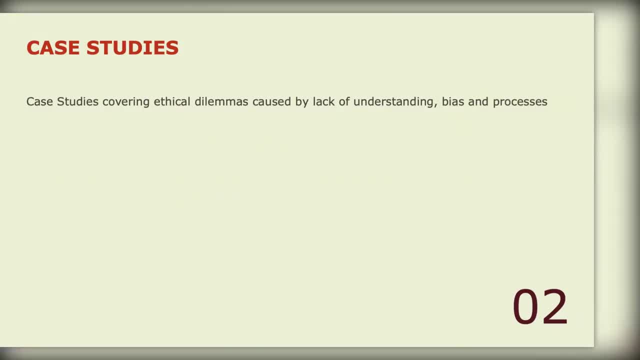 And understanding of how everything works. So, with that said, Let's do a couple of exercises. So I think just talking about the AI ethics might be a bit not very engaging. So I think what would be interesting is I'm going to present a couple of scenarios of engineering companies applying AI. 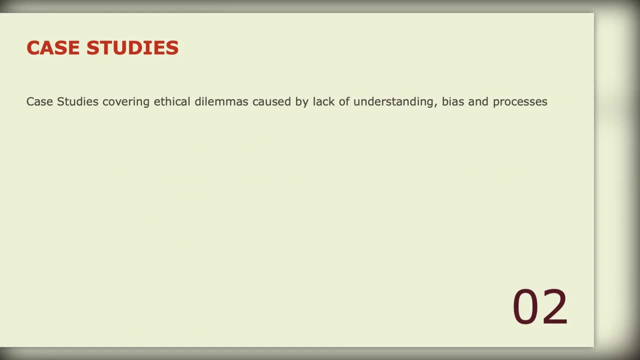 Just to disclaimer, these are fictional And the main thing is there are not many engineering applications that have gone wrong because perhaps not many engineering companies started implementing or it's not like published yet. on the Internet There are some. There are some case studies of failed AI projects, mostly around the ethics side and models not forming or being racist. 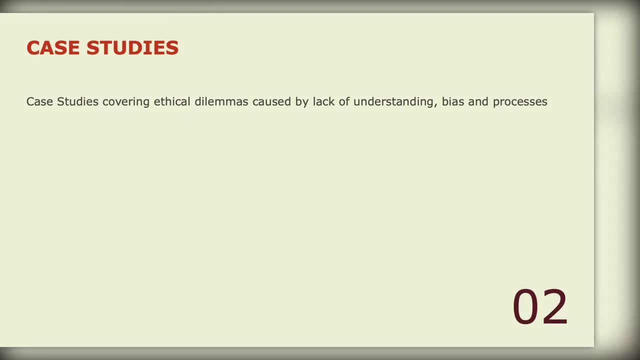 But what I'm going to do is go over where things could break down in terms of the ethics and AI And I'm going to give you like a couple of minutes to have a go and just post in the chat what you think is going to go wrong in each scenario. 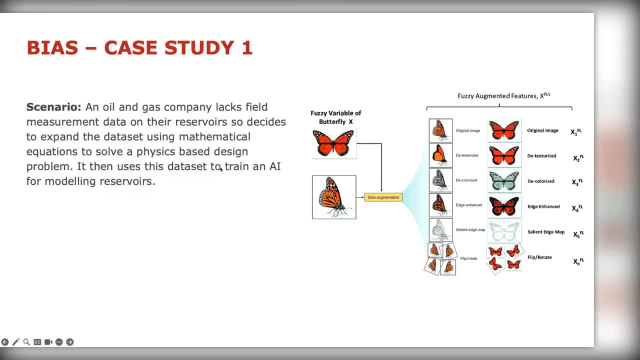 And then I'm going to discuss the implications. So the first scenario is case study one. So this is an oil and gas company- It's a very fictional company. They lack field measurements under their reservoirs And basically they want to build an AI model to predict the reservoir specification depending on the measurements that they have on the data. 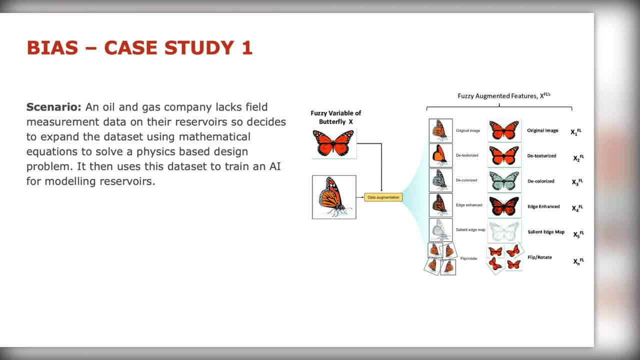 So they decide to expand on the data set using mathematical equations to solve the physics best design problem. And what they do then is they use this mathematical equations to create new data, because they don't have enough measurement data, So they use mathematical equations to generate. 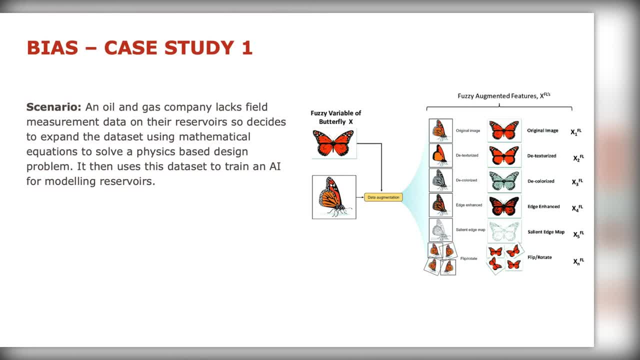 Additional data. We call this data augmentation. So they create lots of new data based on this And then they include it in the training data set for training their AI model so that they can predict new designs of. they can basically use it to help with designing new reservoirs. 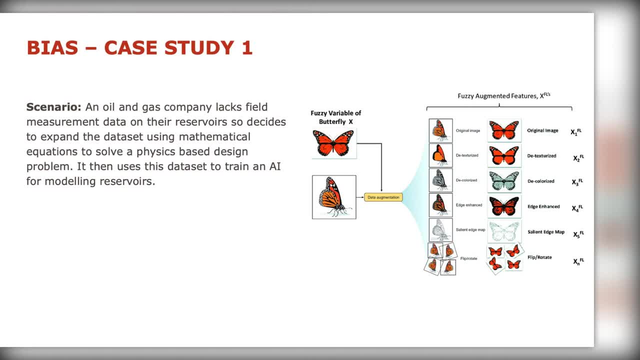 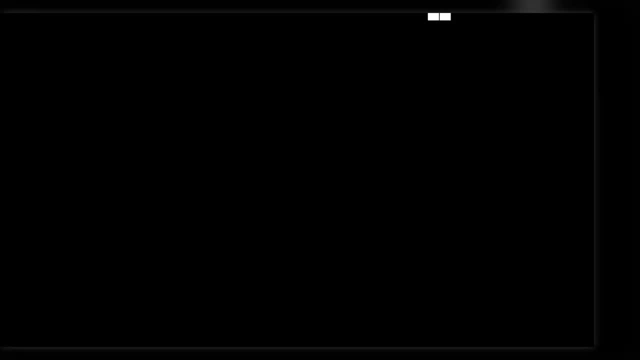 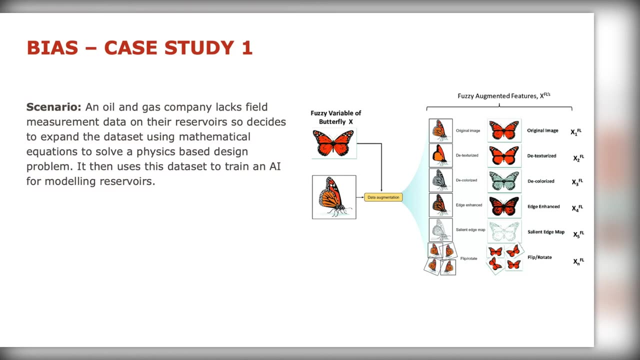 So what do you think is the implication of doing this in an engineering context? So just to talk about data augmentation, these are like algorithms you write, where it takes a set of real data and, depending on some fuzzy variable- X for example- it generates variations of data in conservation. 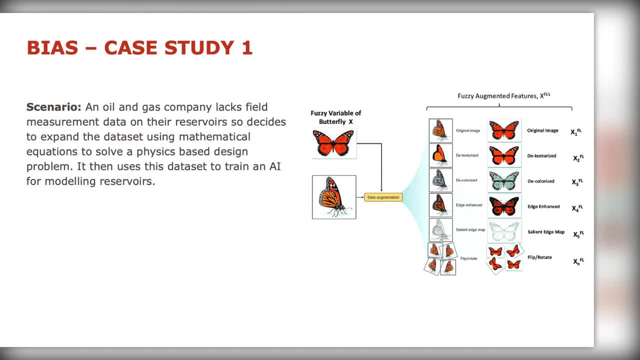 This includes rotating pictures, flipping them, I don't know, changing the color a bit and doing those kind of stuff. So it's a lot of different things. So it's a lot of different things. So it's a lot of different things. 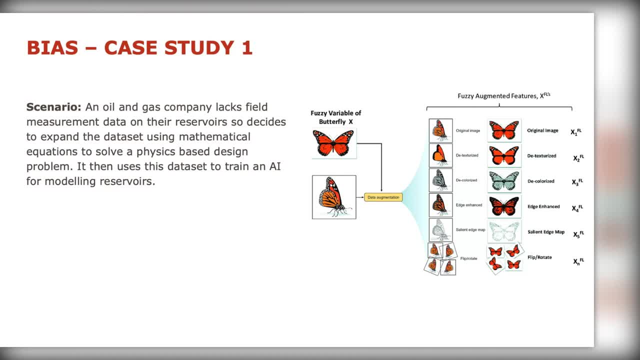 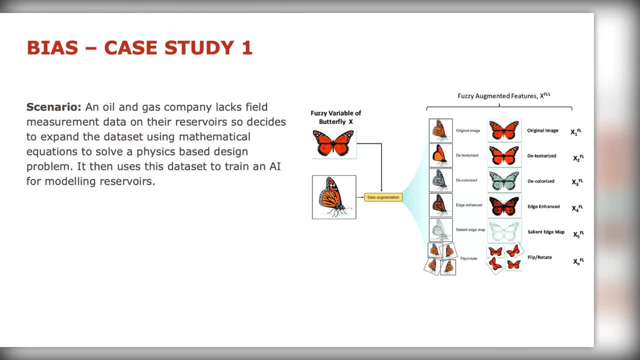 So what they do is just they use mathematical equations to come up with new numbers. Okay, so this one, you've said it really well. there would be compound errors, there would be mathematical errors and reliability errors. So Thomas says: rubbish is rubbish in, rubbish out. 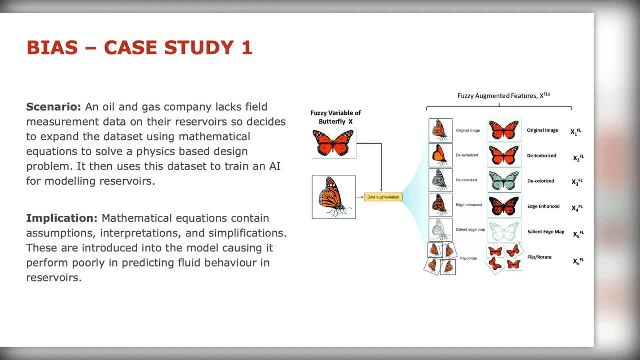 So it doesn't necessarily mean that it's rubbish. but the main thing is: mathematical equations have assumptions And I think Manoj has really put it firmly like put it on the nail, put the nail on the head here by saying: because mathematical equations have assumptions, interpretation and simplification. 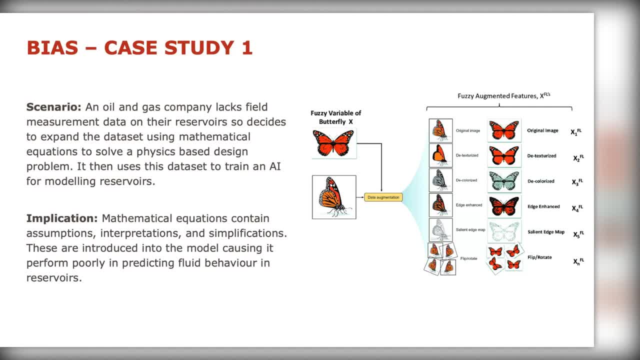 what happens is that you're not considering a lot of real-world variables in it. Some of these field measurements you take might have already been correlated with a bunch of other factors that you don't know about. that makes it a real measurement, whereas, like if you start using mathematical equations, you may end up introducing biases into your 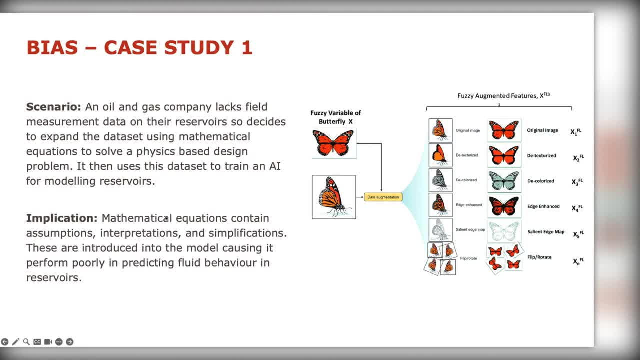 data that may not necessarily predict the behaviour, And this is normally a problem with the engineering team, And they're- They're the person signing off on these models, And if you don't have enough proper processes in place, you may introduce bias into your 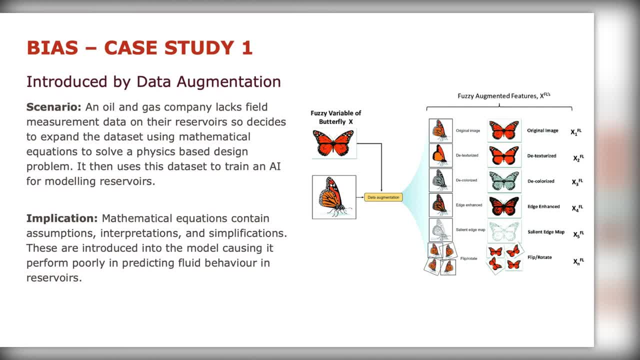 data and into your model by data augmentation, And this is like one of the examples of how bias could be introduced. Because you don't have enough data, you have to make it, so you start making fake data, but the fake data doesn't represent reality. 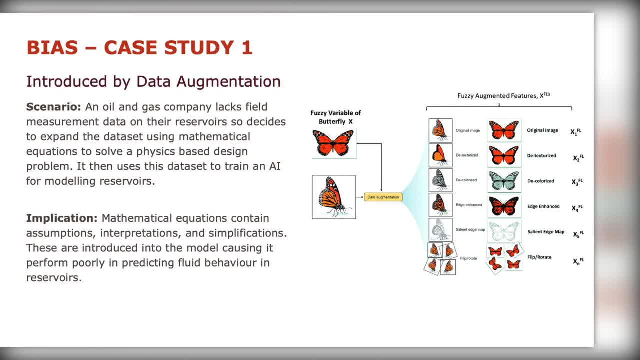 And you test it on the fake data again, not on the real data, then you don't catch it And it goes into a real-world scenario because you think all your tests are passing. So let's put it in real-world scenarios. So this is where you need a set of processes in place to make sure that your models are. 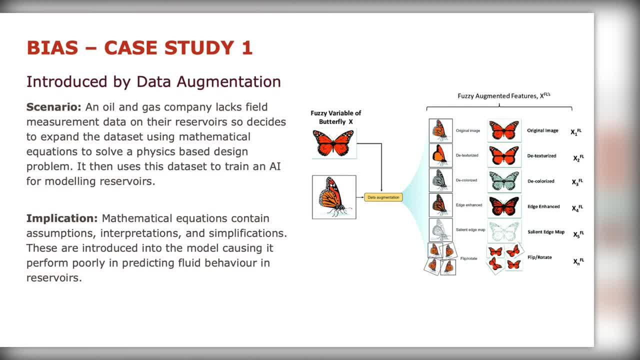 actually working against real-world environments rather than just your testing environment, And there are, If you think of the Swiss cheese model, there are basically layers in the Swiss cheese that prevents any hazardous situation from occurring, because you catch it before it goes into a real-world scenario. 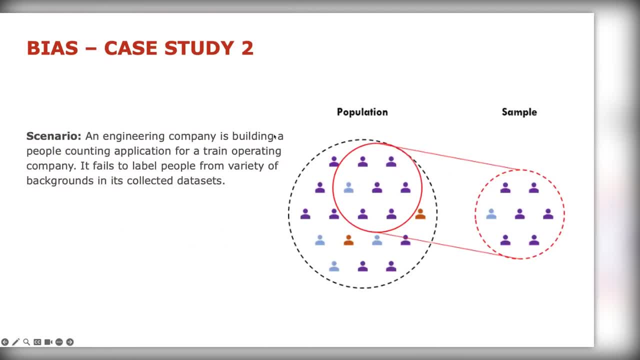 So that's the first case study. Let's look at another one, Let's look at this one. This one should be easy as well. So this one is an engineering company who is building a people counting application for a train operating company. So they are building a computer vision model to count people on and off the train. 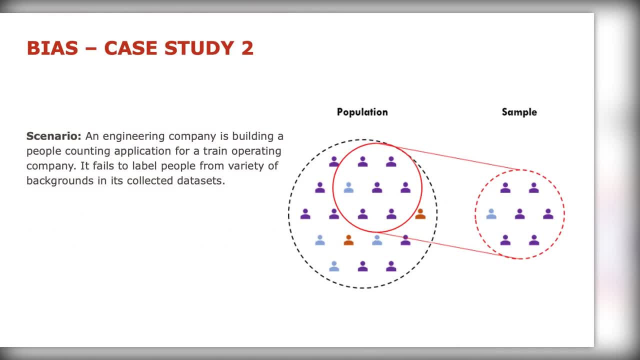 They want to see the demand, and so they want to be able to predict demand And, based on that, basically optimize their train table schedule. Now the thing is this model: it fails to label people from a variety of backgrounds in its collected data set. 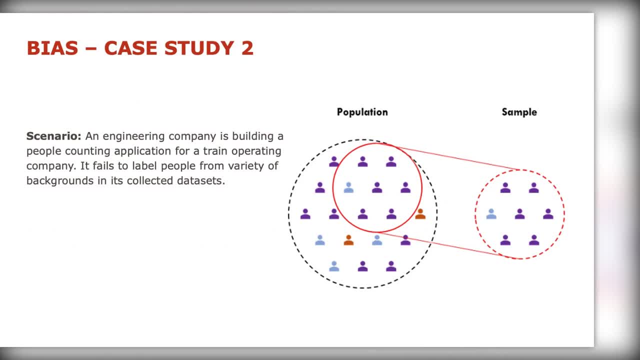 So what do you think is that? Okay, Let's look at that, And what are the implications of it? So they train a computer vision model. however, it can't see some people, And why can it not see those people? Okay, 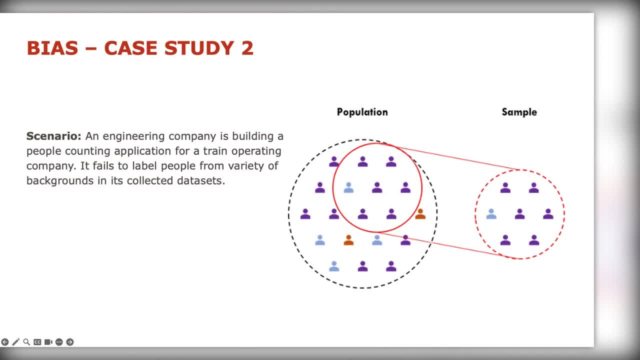 So I'm just going to look at the data set and I'm going to try to tell you what it looks like. Let's look at the data set, Okay. So I'm going to look at that. This is an example of bias. 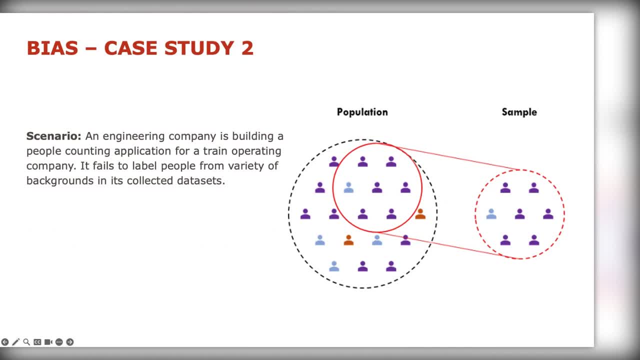 And this one is actually more common than you think And it's also very hard sometimes. This is why you need to know statistics and you need to understand the. you need to understand what a stratified sampling is. You need to understand sampling bias. 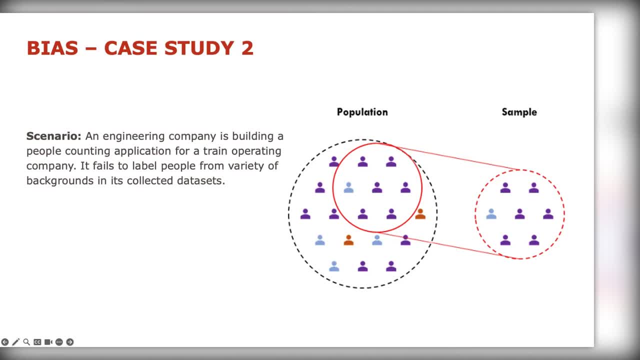 And this is a, this is a, this is a very common thing. This is a very common thing- And I'm going to look at this- is an example of bias being introduced by sampling. So when you sample, when you have some data set of 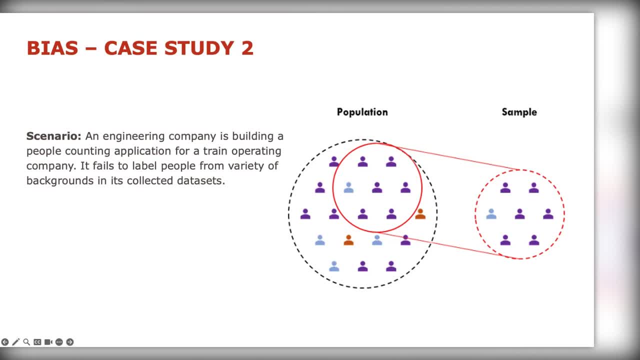 your environment and you're trying to build an AI model on top, you need to make sure that the sample represents the whole population. Even if the sample is not enough data, at least it should represent the same number of people in here. So, for example, in this example we have a lot of blue. 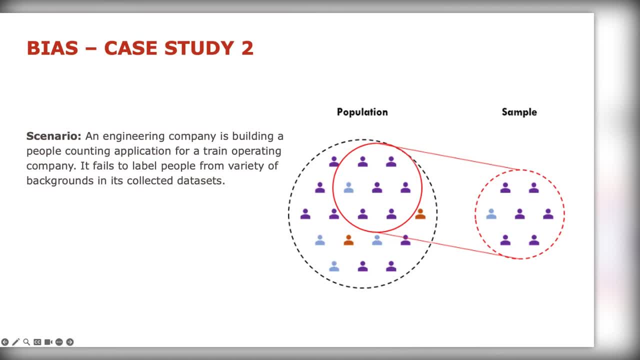 we have basically a lot of purple and blue and one blue which kind of like represents their full population, but we don't have any orange persons in it. And basically this example is what happens is you don't, for example, see black people, like your model cannot see it, or you miss. 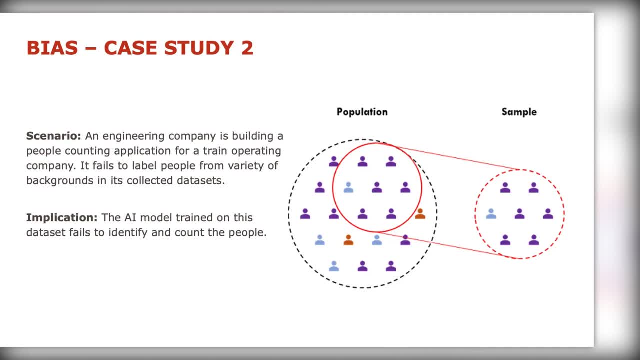 blonde people actually like. because of the lighting conditions of your computer vision model, your model from the CCTV camera, for example, cannot see blonde people, So it doesn't actually start detecting them and tracking them And basically in some stations you may not have. 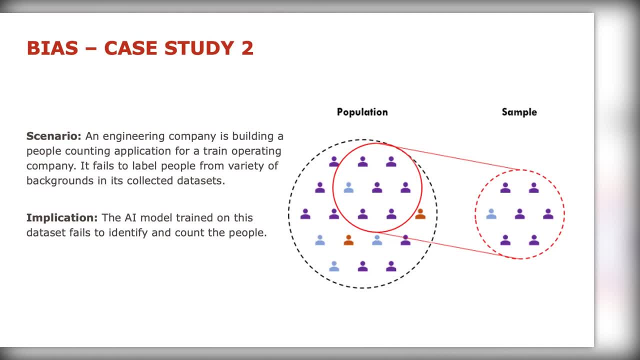 any demand. So if any city in the country has a lot of people with blonde hair, they will have not a lot of trains scheduled for them. because then, because your models are predicting there are no people there. So this is an example of a model basically being biased, because those bias is introduced by 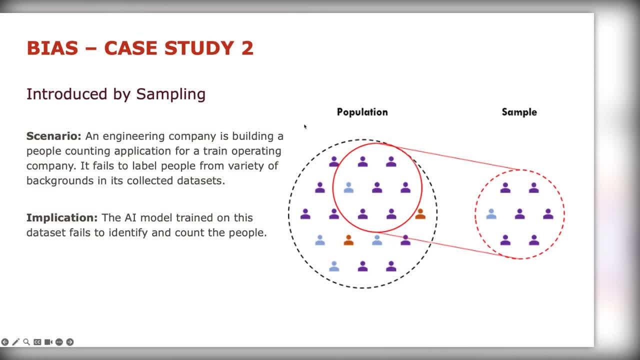 sampling, So you need to make sure you have a distributed classification across all of your samples. You have enough classes of each sample, So you have samples of each class in your data to make sure your model gets trained on all of them at the same rate and there is no bias on gender or any of those other factors. 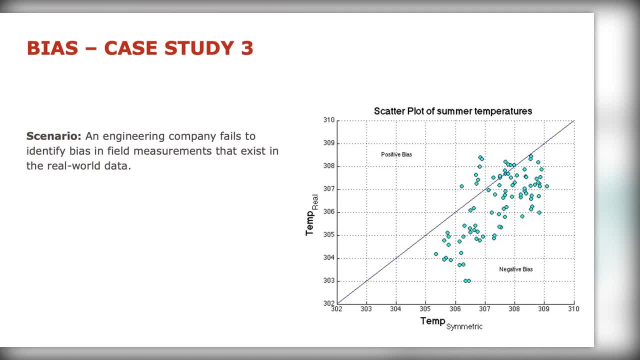 Let's look at another one. So this one is interesting because it's not your fault that this may happen, but it may happen. So this one is an engineering company that fails to identify bias in field measurements that exist in the real world data. 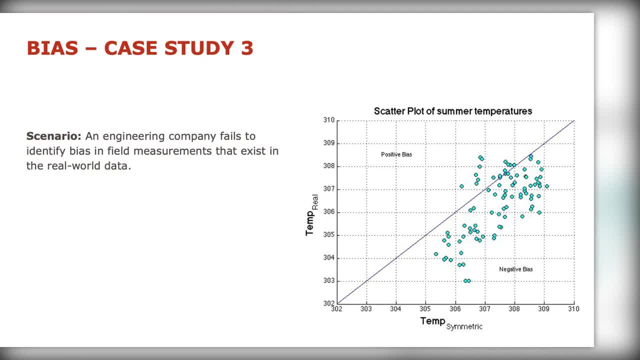 So one part is understanding why this bias exists and the other part is basically catching it, And this comes down to one thing that you may identify: but what do you think the implications are and what can they do to identify it? So in this example here we have a system that has collected field measurements on temperatures. 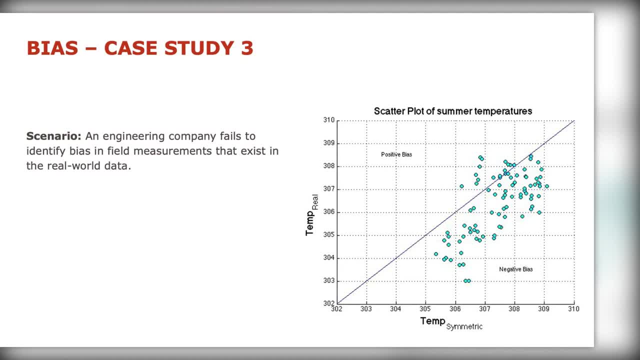 but because we are in the summer seasons, the temperature data is biased towards higher temperatures, towards the negative side, because of the seasonality, And their modeling team didn't consider the seasonality factor. What happens with this one? is it normally, when you train an AI model on real-world data sets, that you haven't done? 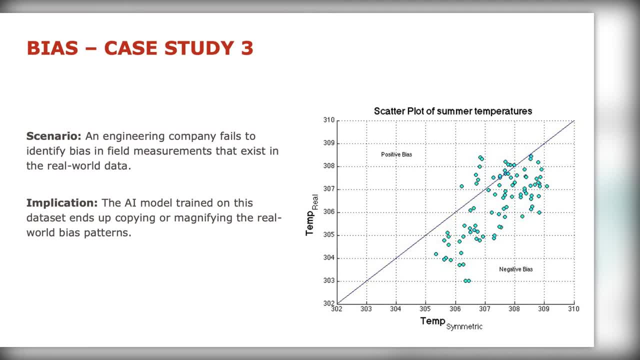 performed enough exploratory data analysis on to identify these biases and cleaning that bias out of the data, you will end up building AI models that then generate more data with those biases in it And it's like a loop, So the model starts actually magnifying. 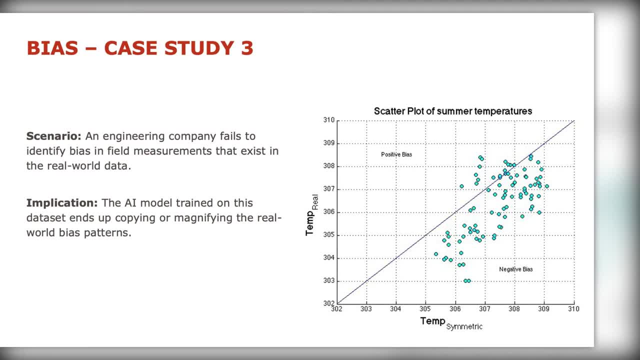 copying, or worse, magnifying, those real world bias patterns, depending on how it works. so this is actually reflects the real world patterns in the data that introduce their the biases and add. layer detection can help with removing these biases but also understanding your data. so that's why it's important to have competent people on the project with real world. 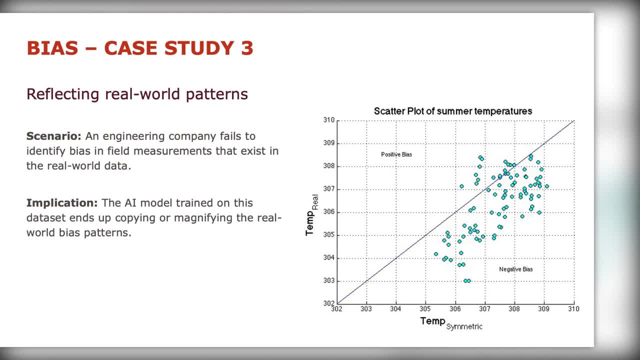 understanding of what the data is. so your project teams: it needs to include people who really fully understand the data at the same time, people who can build models and software engineers, and those those different, different team uh- skill patterns, in order to make sure that all of this is included. 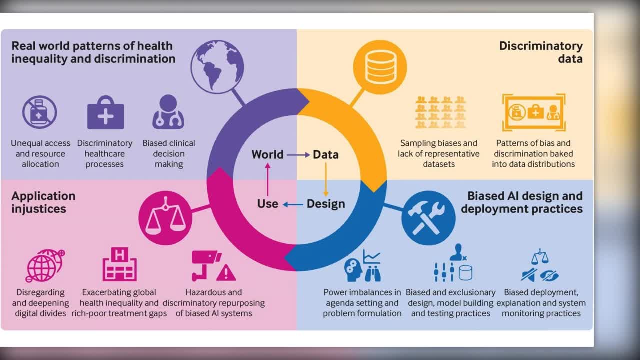 so normally what happens with bias is that if you start from top right corner and we go around in a clockwise manner, um, so basically when you collect the data from the world, there could be bias in the data, and normally these biases could be introduced by sampling. it could be patterns in the bias and discrimination baked into data distributions. 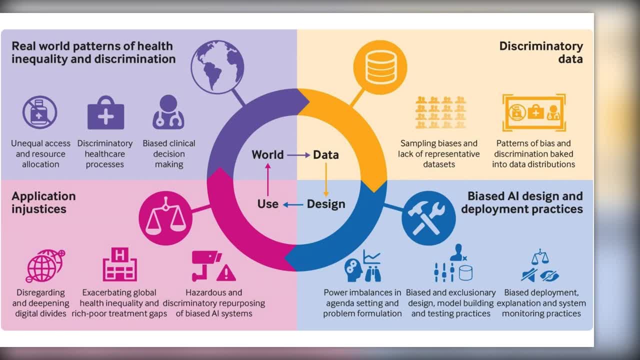 and when you build models on it and your design could also introduce some bias into your data, such as imbalances when you, when you're doing, when you're writing your algorithms, how you build your models and how you clean your data sets could introduce bias, and also, if you don't have enough monitoring systems in place, you could also magnify this. 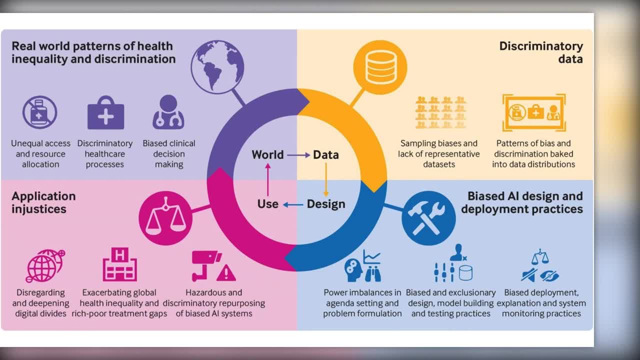 bias. so what happens is when this, when this model goes into use, um, it into it, starts introducing in era, you can identify the control main risks of this model and think about how high these biases are and with this and so on. once you gave all these categories a little bit, uh. 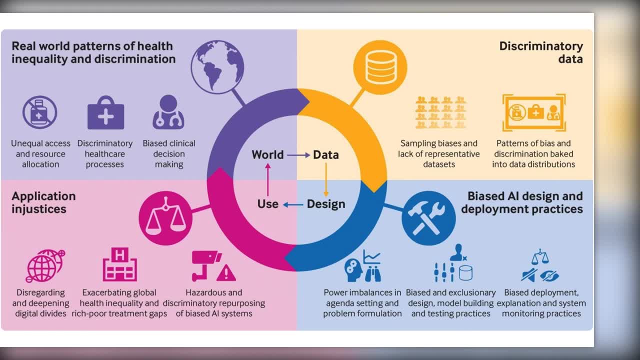 but those are not actually undeclared, so it it actually falls into considering for every entity, so, for example, for terms ofjustices in the world. so it deepens digital, divides it. it promotes health inequality and promotes gaps between people. it creates hazardous and discriminatory situations and then 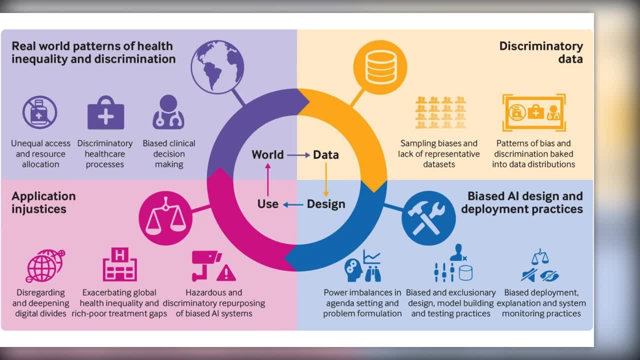 And this is a self-fulfilling loop. So this is how AI models can start introducing and magnifying biases in the real-world scenarios. So this is how what happens. This is why, when you collect field measurement data, you may have bias in it because of pre-existing bias. 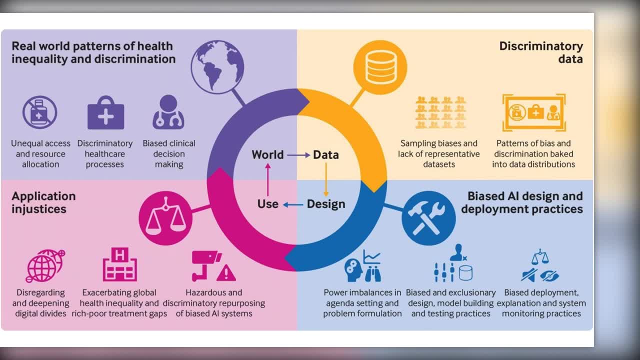 in the past or because someone deployed an AI model and that also starts adding bias into the environment. So you need to make sure that you detect this bias and then clean it before you start building your own AI models on top. Let's look at another case study. 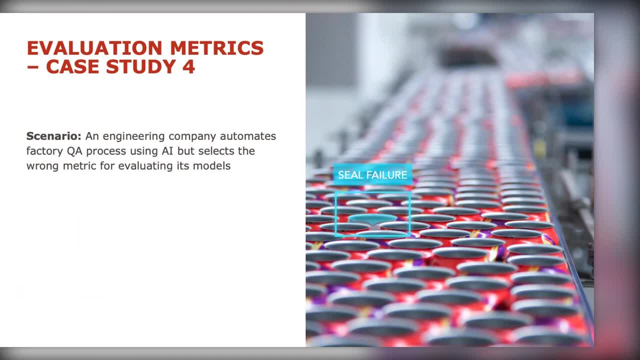 So these are not from bias, but let's look at evaluation metrics. This is related to evaluation metrics that we talked about previously. So here an engineering company wants to automate a factory Q&A process using AI, but selects the wrong metric for evaluating its models. 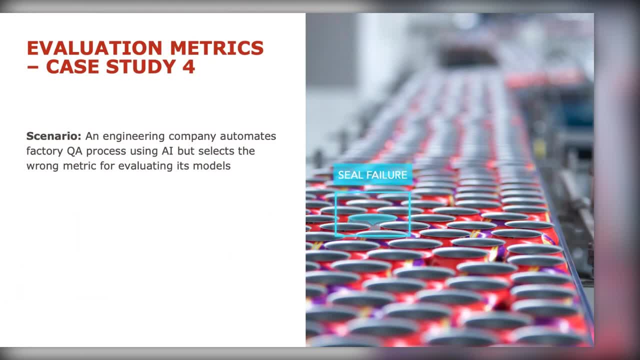 What happens in this scenario And what kind of metric could they choose instead? What have they chosen and what they could choose instead? that has caused this issue. So this case study is all about analyzing the bias in these models by looking at the neural networks. 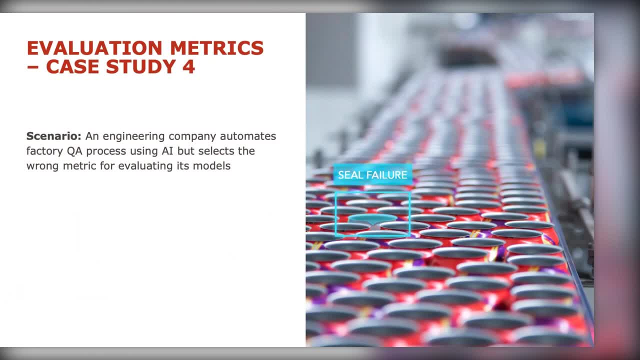 and looking at the biomechanics and monitoring them. So the first thing to do is to look at the real-world wide and see if there are any problems with the models. So the problem is that the model itself has some cognitive issues. It doesn't have enough information. 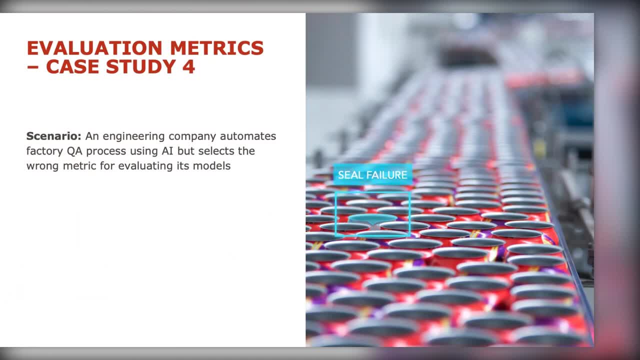 to be able to do that And the problem is that the models are not able to automate these. So, if I come back to the system, this falls in IE or it falls in the IE model because it's very complex problem at hand. So in this case, when you're trying to detect a faulty item in the factory, 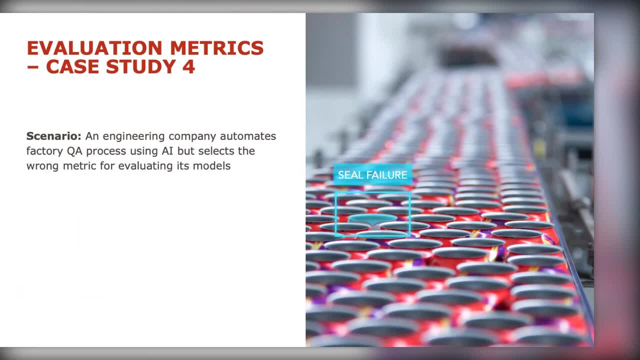 production line. you are looking at a model that classifies items as good or bad, So it is like a classification problem, And if you start using a metric such as accuracy, you may end up with a model with a testing method with evaluation metrics that suggest. 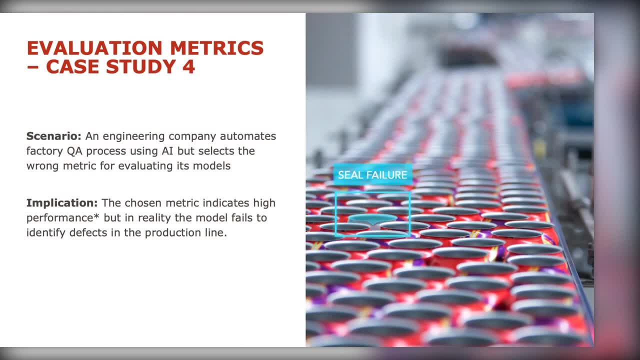 99% accuracy. So if we say accuracy is the metric that we're going to go for, what happens is we end up with a model that basically suggests 99% accuracy. So it's good enough, We should put it in production. But let me give you an example. A good example of this is spam detection in your 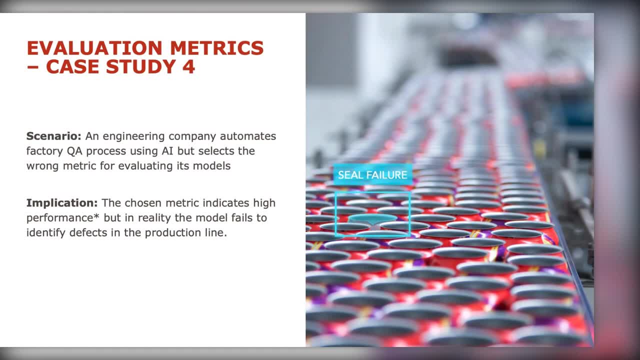 email. So if you have a spam detection in your email and you have a spam detection in your email and you have a spam detection in your email and you have a spam detection in your email systems, So in spam detection a 99% accurate model is a model that can detect all the non-spam. 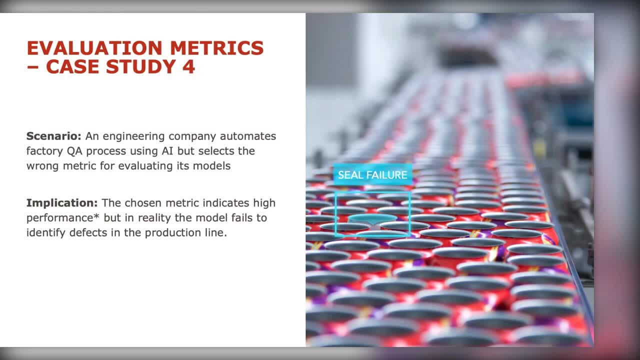 items from 100 items. So let's say you have 100 emails, only one of them is spam. If your model detects 99 of those items, as if it detects all of the items as non-spam, it is 99% accurate. So if 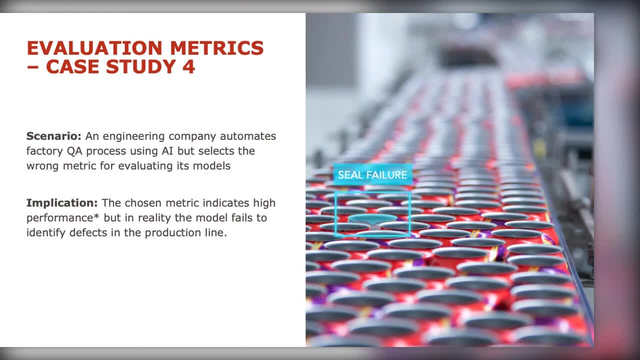 it fails to detect the spam one, it's still 99% accurate because it has identified the other 99 as non-spam. So if you use accuracy, you end up thinking that you've built a model that can detect spam items in this scenario, in the manufacturing scenario, If your model fails to. 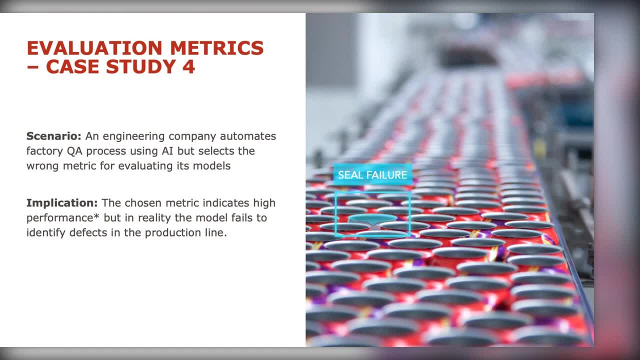 identify any faulty products out of 100 products, and there's 99 products that are non-faulty. you have a 99% accurate model. In this scenario, the chosen metric is incorrect And what you need to do is you need to make sure to use the right metrics, And that comes down to understanding. 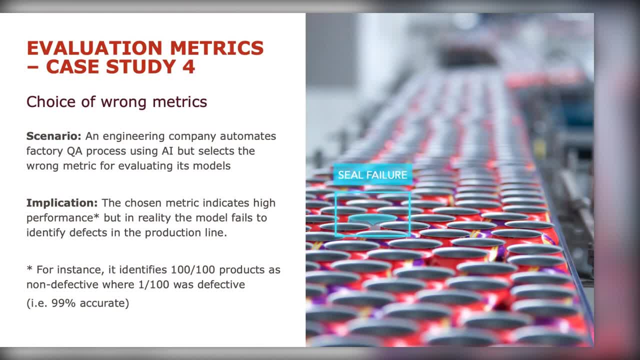 your problem Here. the problem is not a problem that you need to solve with accuracy. This is a problem, a classification problem, And classification problems come with their own set of metrics, such as recall, precision, F1, scar. So these are like the metrics that we will start discussing. 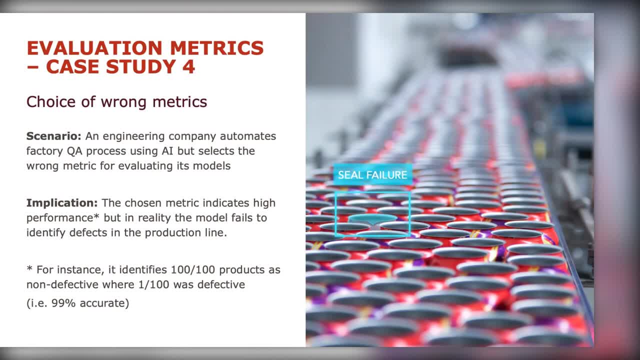 when it goes to more technical workshops in our courses, But you need to make sure that you use the right metrics when it comes to building a model. So, if you have a problem, you need to use the right metrics when it comes to building your AI systems, because those metrics could then 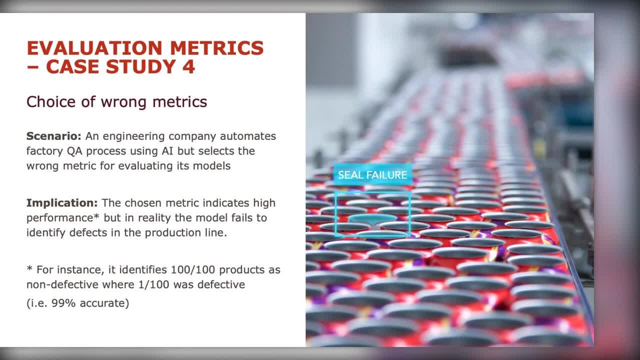 help you identify how many of the items you've selected are actually correct. the predictions that the model has given is correct, and has it even detected all of the positive cases correctly? So, how many false positives you have, how many false negatives you have, And using those, 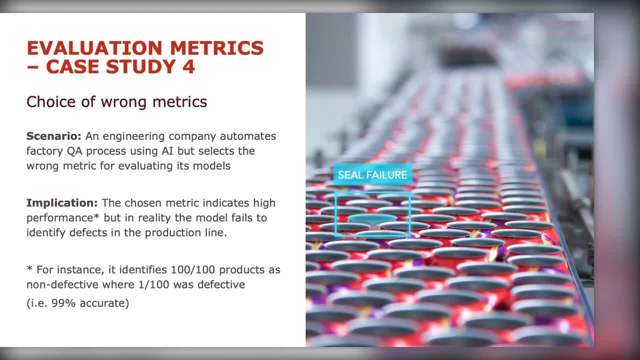 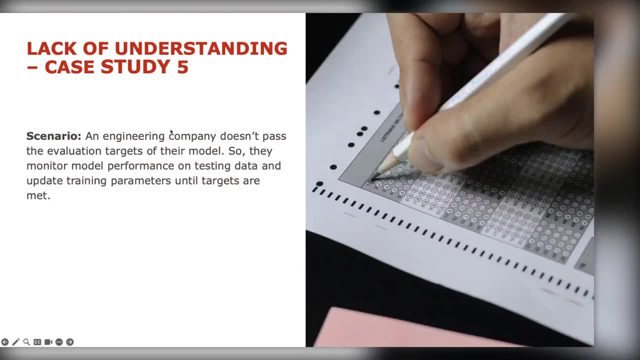 you can then measure the performance of your factory fault detection AI model. Let's look at another one, scenario five: An engineering company doesn't pass the evaluation targets of their model, So they monitor the model performance on testing data and update the training parameters on the targets are met. So let me describe this a bit more. So you have. 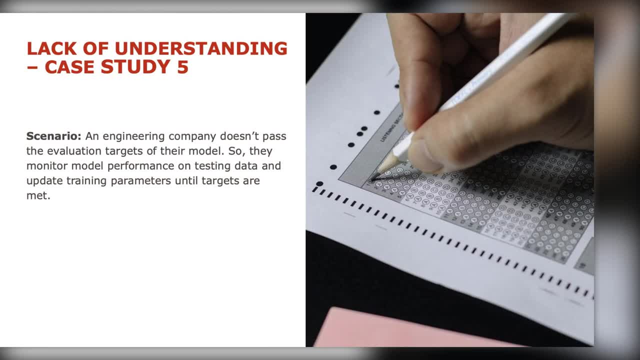 a team. they're training an AI model with some training data, So they keep training it and it's not passing the tests. So what they do is they just keep tinkering with their algorithms until the model that they create passes the tests. So what is the problem here? 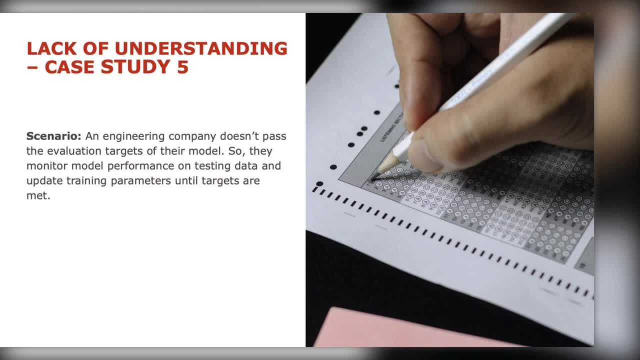 And then, once it passes the test, they feel confident that it's good enough. they then put it into an actual real world environment for use. they sent it to customers to use in actual real world environment. So this comes down from lack of understanding of how. 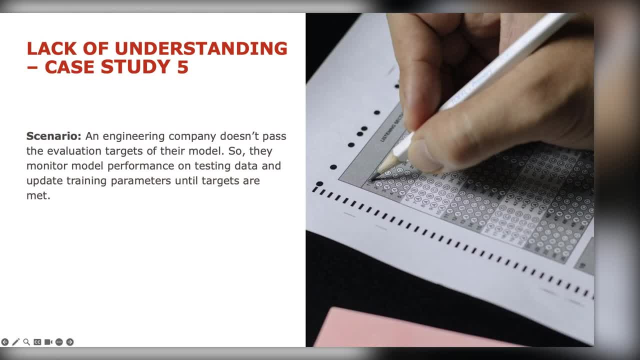 ai models should be built. so lack of competence, lack of understanding, is one of the major concerns when it comes to building ai tools, because if you really don't understand the full process of why, well, i mean on the surface, they're doing it wrong. they are building a model, um, but 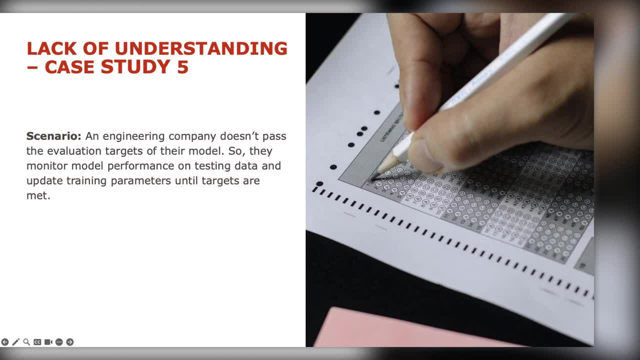 they are testing it and they make sure the tests are passing, but they are missing a very important step. so so robert is saying designing for tests without fully understanding the implemented changes, ben says not a robust validation of the model and usa says hard to determine. neil says giving the model the answers. essentially, 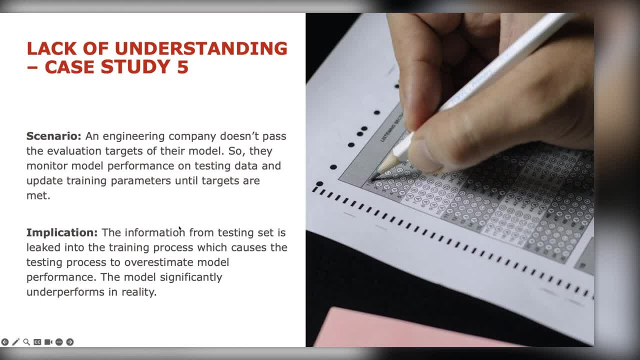 so the actual answer yes- is the fact that you are trying to test any student, so think of ai models as like a kid. so if you are trying to, you know, put the kid to an exam and help them pass the exam. you don't sit down and give them the exam answers um, until they pass the exam. it's as if you are sitting the 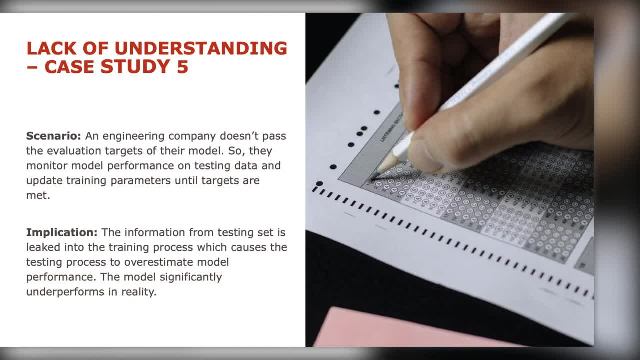 model and he's giving it the answers basically. so what happens is the model will perform well, like if your homework is basically the exam questions, um, they will pass the exam. but in the real world scenario the questions are different again, and if they haven't generalized, if their learning is not generalized well enough, they will not pass the real world exam. they will. 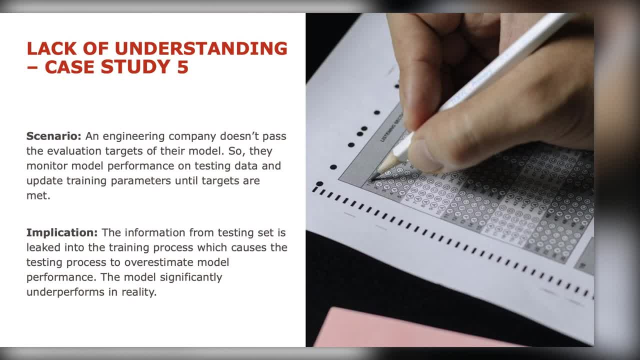 just pass your exam. so this is what's happening here. what they've done is something called the data leakage, um, where the data from the testing set is leaking into the model. by just you playing around with the hyper parameters of your algorithm, you're effectively telling the algorithm that like. 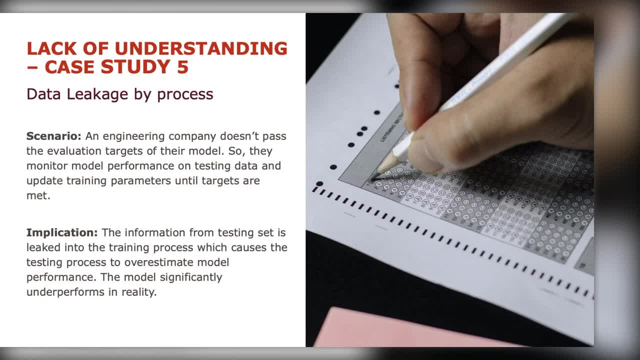 you're just giving it lots of hints until the- until the model figures out what the actual, real answers are. that's why normally what happens is you divide your data set into three sets: a testing set, a validation set and a training set. you only test and you do this process with 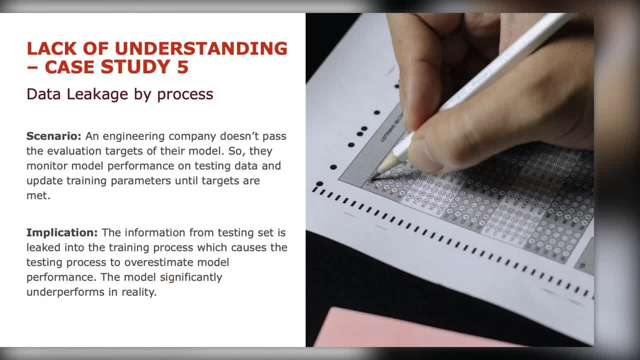 the validation set. you'd never touch your testing set and when you're happy with how the model is performing on the validation set. so your own exam. you also do a real world exam. so you have an additional step where you perform a real world exam of the model. 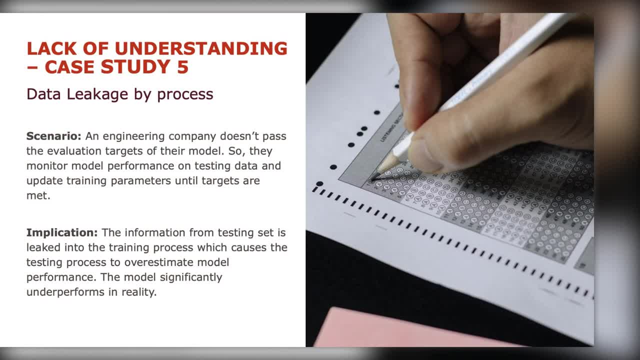 if it passes the real world exam, then you can be confident that it could, probably, it probably will- perform well on other real world exams. but if you just pass your own exam and you then put it in real world environments, you may end up introducing issues because your model is still not ready. 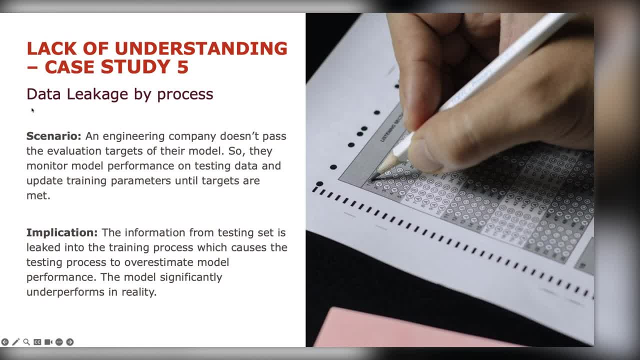 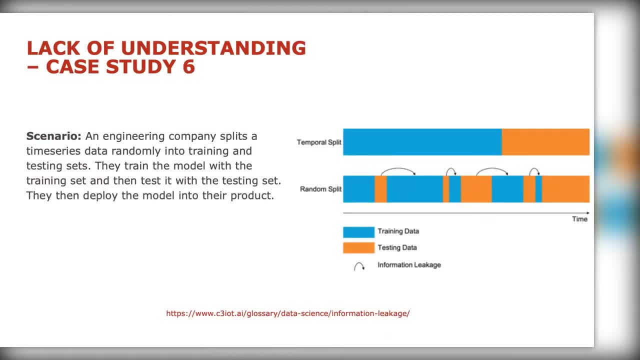 to go into real world environments. so that's called lack of understanding. data leakage by process. this one is very interesting and this comes down to your understanding of what a time series data looks like. so an engineering company splits the time series data randomly into training and testing sets. they train the model with the training set and then test it with the testing set. 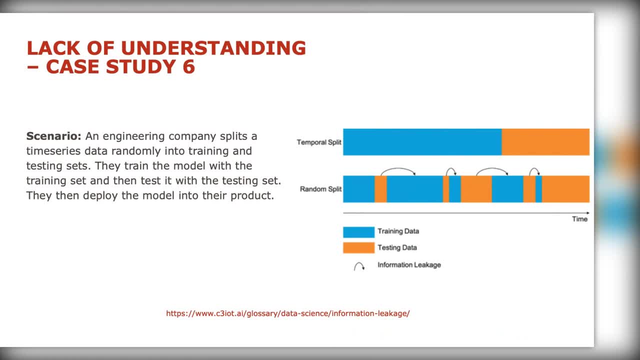 they then deploy the model into their product. what is the problem with this one? so this one is very. this is a technical understanding of what time series data is and um, why, why it's a problem? i mean, to some extent i'm giving you the answer by that on the picture. 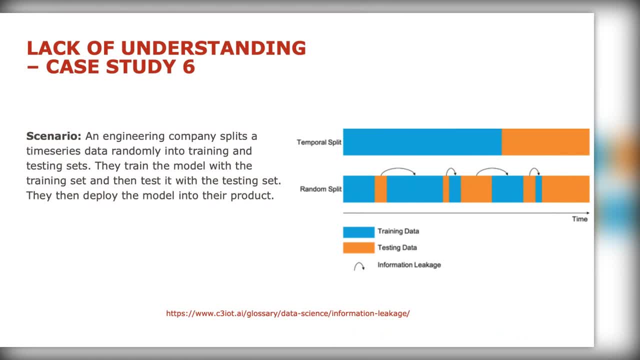 but what is the implication here if they do it this way? so they just basically, let's say, the engineer on the project, they follow the tutorial online and they just follow the tutorial to the t on their on their time series data. the tutorial is using uh, structured data, tabular data or something else. it's not time series, there is no. 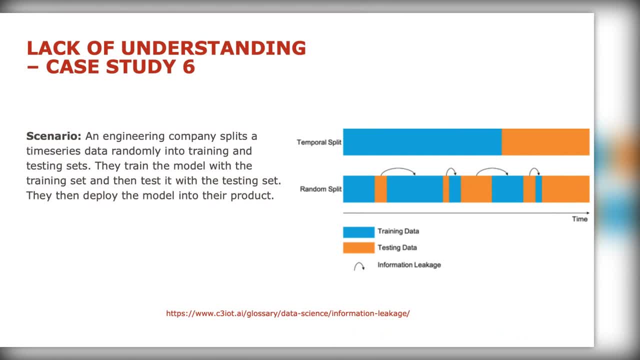 time. so this one lives for like five minutes, so let's regulate it. and if it's likeuffle and over time, this is similar to where we go to the model sc Miles, the model again, but there you do what you like. there will be a week. Ew, what's the root theorem? like what happens if you do a random split. 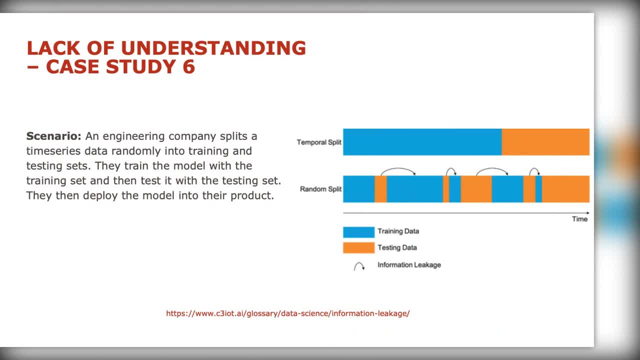 like what is exactly happening and what happens if you do a random split of the data into training set and testing set. so let's say you have a. you have a table of data, some rows. it's sorted by date, so you sort it by date time, so you have a column that has data on it and you store the data by date, let's say temperature over time, right? so like you're predicting the day time that you have a problem, you have a. we've already calculated your Gaza as our data. that is connected to no data. so by which time I'm zie an object. so you are, if you and your other climate, and that's we are a t on the contract. 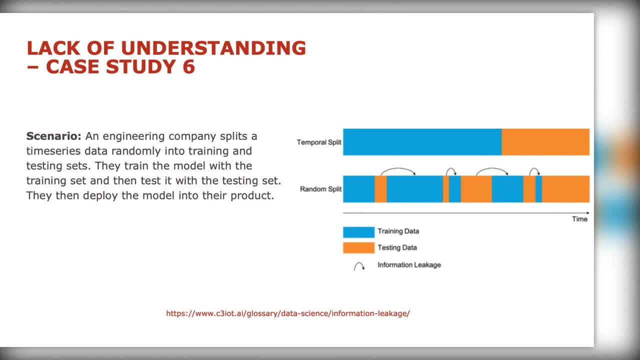 right. so like you're predicting weather patterns- and you have, you're trying to predict the temperature of the weather. it's a time series data. you then basically shuffle the rows and then you pick some rows randomly for training and then you pick some rows randomly for testing. 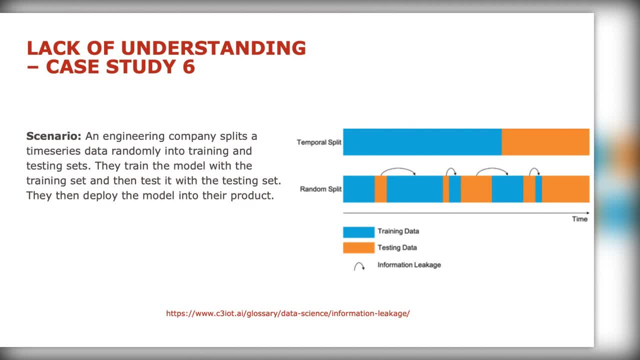 so this one is more like a technical understanding issue of how time series data works. so sarpsis: effect of time on the data not mitigated for not a realistic data set. any other ideas? validity of the sample- okay, so this one is quite hard. um, you end up ignoring the wider context surrounding the data. 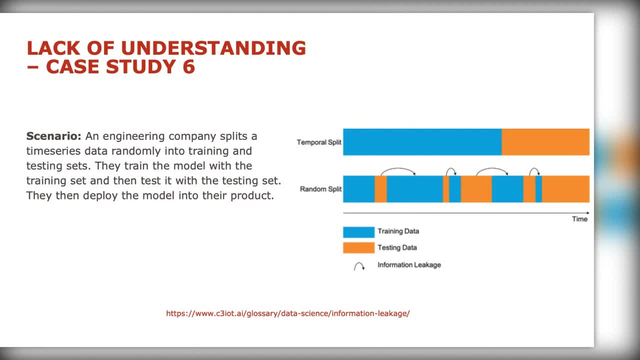 any, any other ideas? no constants in the data used. giving ai the answers by doing the random splits. one of these is quite common. it's called the random split, correct? anyone guess which one of those answers are correct? effect of time on data- another realistic data: validity of the sample you end up ignoring. 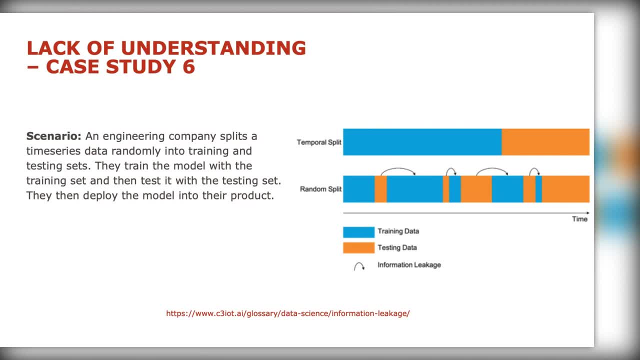 the wider context giving ai the answers: no validation before deployment, no constancy in the data used. so, jonathan, well done. that's the answer. you've given the model the answer. it has the future info of the training data. so, when it comes to using time series data, you have two different ways that you can split your data set into. 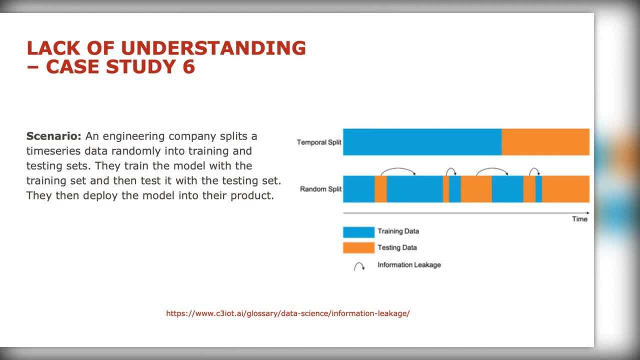 a training set and a test set. so the process is: you train your model with a training set and then you test it on the tester to make sure it works. the problem here is because you have a time series data. your data is ordered by time. when you do a random split, you have some future data and some 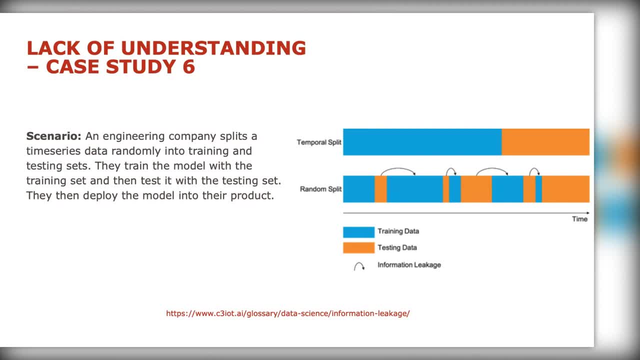 past data mixed together and you give it to the model. the model learns the future patterns. it's It's like asking someone to predict the future, but telling them what the future is. So what you need to do is you need to split your data using the temporal spirit. 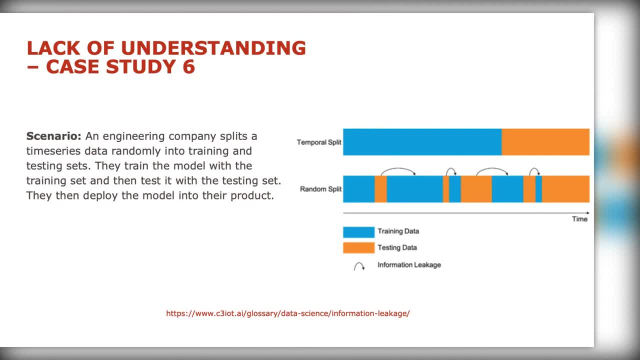 So you completely take a piece of future, you hide it from the model completely. that's your test set and then you train your and then whatever is left is the historical data. So the demarcation point in the first, so in the temporal split, if you look at the diagram, 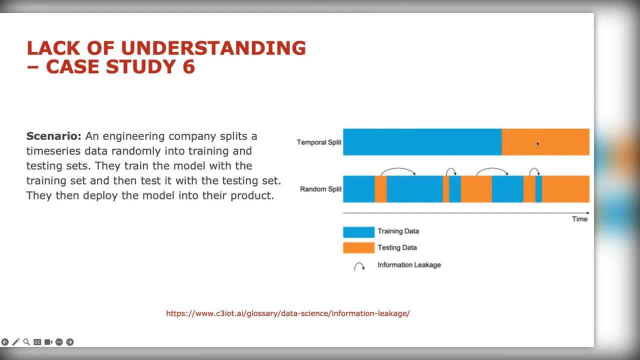 where the blue meets the orange. that's the demarcation point. let's say that's the present time. Anything before that is historical. anything before that is future. anything after that is the future. You should only give the historical time to the model to train. 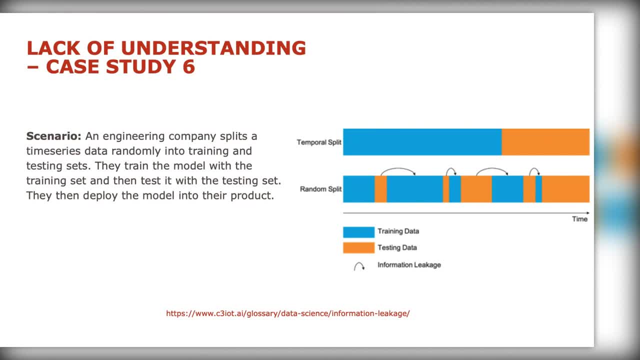 If you start mixing the future with the past in this context, what ends up happening is that it will perform poorly when you apply to the real world, Because on your tests, even you've chosen the metrics correctly. you made sure there is no bias. 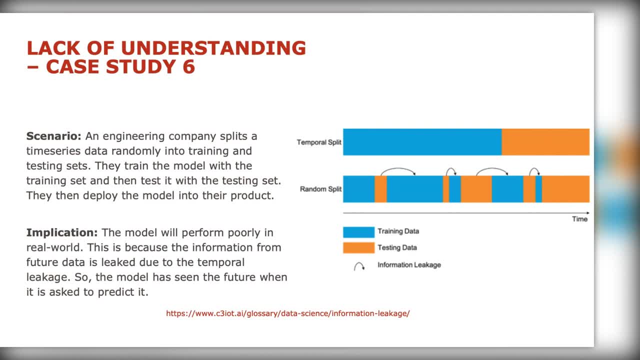 you've done all this stuff. what happens is you are leaking information from future into the past And this leakage is called a temporal leakage. And because of the temporal leakage, the model kind of is seeing the future. So if you've seen the future, you can predict it. 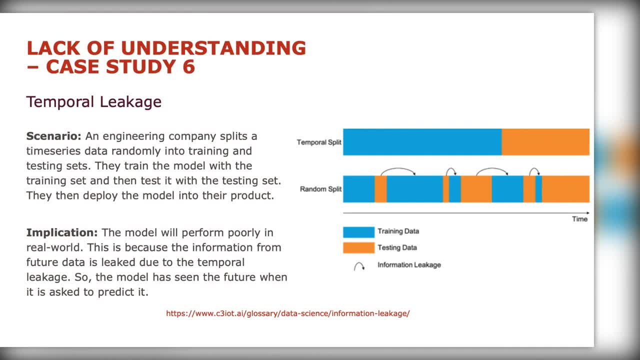 If I see what happens tomorrow, I can tell you what happens tomorrow. You've trained me to tell you what happens tomorrow. It's just basically giving them someone and watch and then they just tell you what happens tomorrow. So the way you, 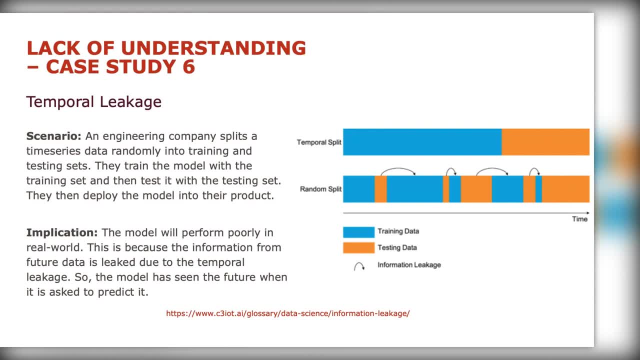 this comes down from a lack of understanding of how time series data work and how it works. How does it apply to the process of building AI models? So a data scientist or an engineer who's building AI tools, they need to understand this phenomenon. 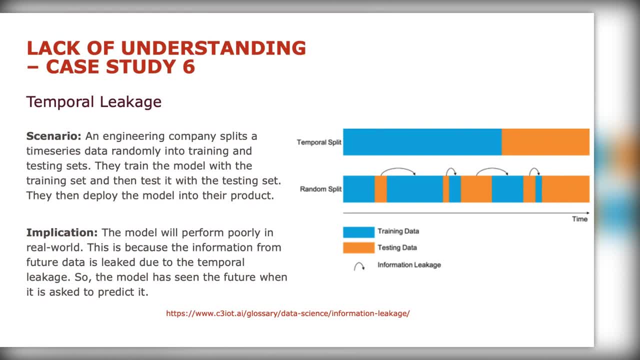 The fact that when they're working with time series data, they need to make sure that when they're splitting their data into random training set and a test set, they can't do that with the time series data, because the information from the future could leak into the past. 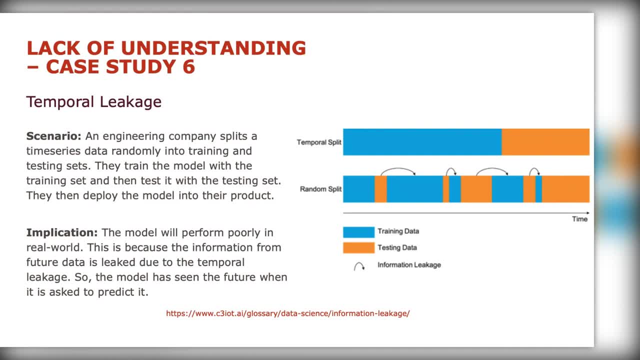 And that's like one of the other reasons it could cause ethical issues. because you are testing and you are the processes may you may skip through them because you are getting good results back. So every time your model is performing really well- 99%, 100%- there is something wrong. 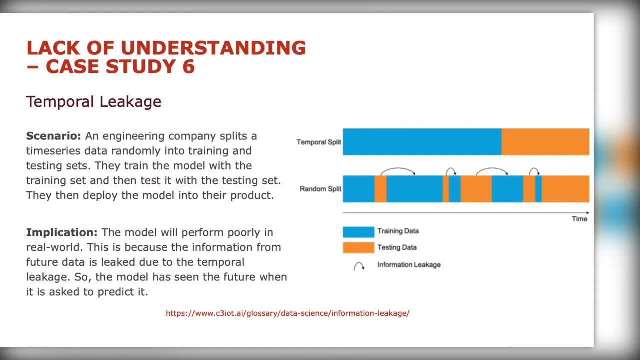 Most of the time there is something wrong. It's not that your model has learned perfectly. There is something wrong with your process. You need to go back and look, And if you just trust your model performing at 100%, there is something you'll probably have missed. 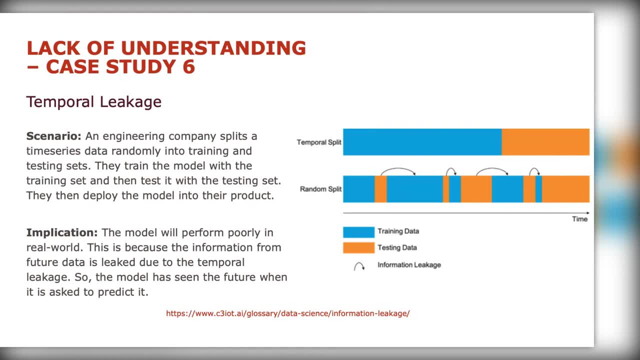 either some correlation or co-correlation, the data that you've not looked for and the model somehow managed to. you know, cheat and understand the exam questions and answer to exam questions, or that you're giving them the question the answers, inadvertently or unconsciously, by doing this kind of work. 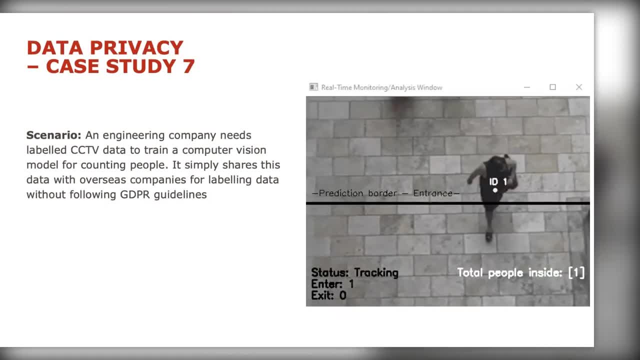 one last example, and then i think that would be the end of it. um, here an engineering company needs label cctv data to train a computer vision model for counting people. so, like something like down the right, they've got a line of judgment, they've trained the model to detect people and 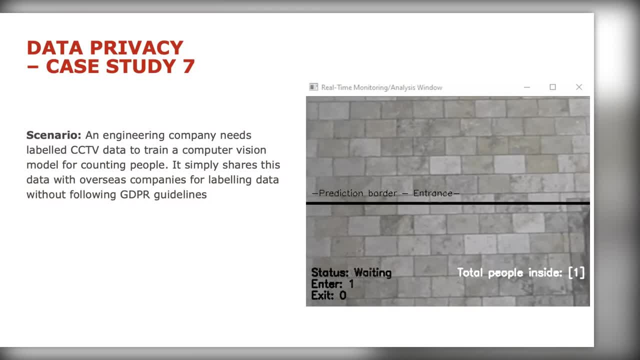 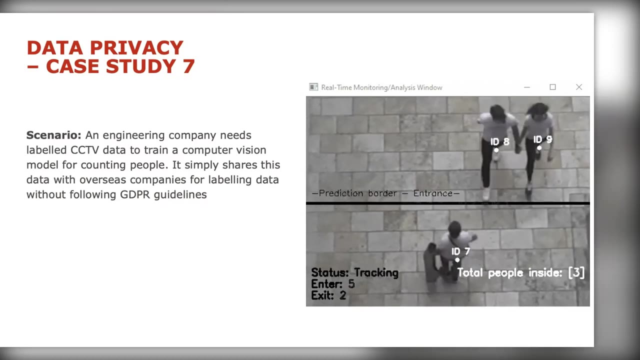 then track them, so each person gets a, gets a dot on them, and then that dot has an id and then, if that dot goes past the line of judgment in a certain direction, they can then count someone as entering or exiting a vehicle, for example a train or here, a building. but what they do is most 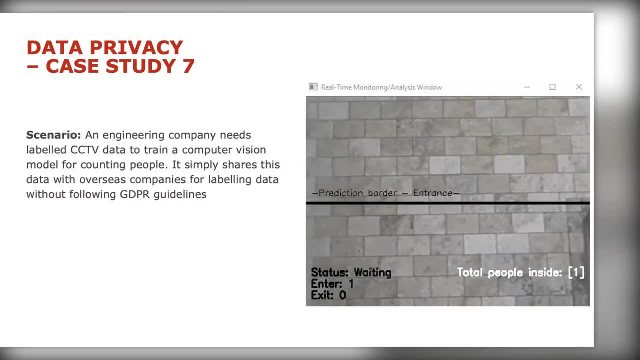 of the time when you're building ai tools, you have to label. you have to basically label your data so that your ai can then learn from that data using those labels. so often this is a very tedious process and it's very expensive if you, if you try to do it, for example in the uk, may 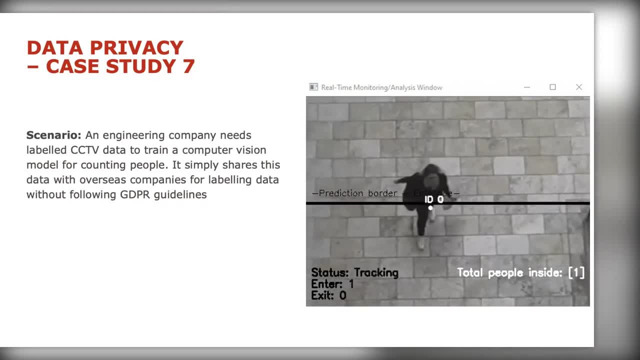 end up being very expensive. so what normally some companies do? they send this data to others overseas countries at a cheaper price to label them. so what they do is they just simply share this data to an overseas company for labeling, but they don't follow any kind of gdpr rules or 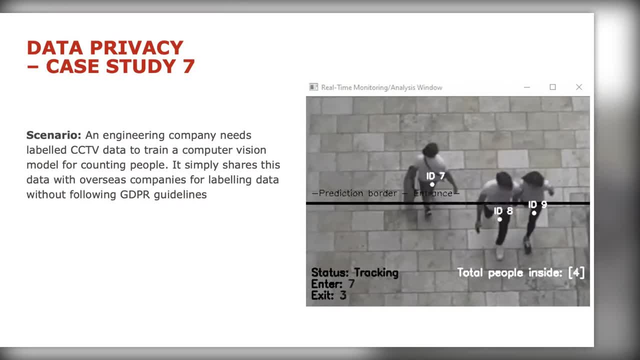 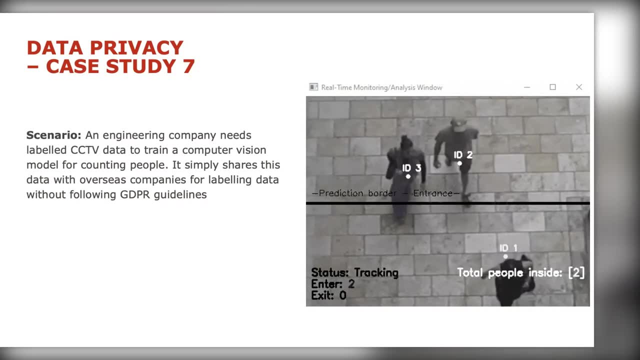 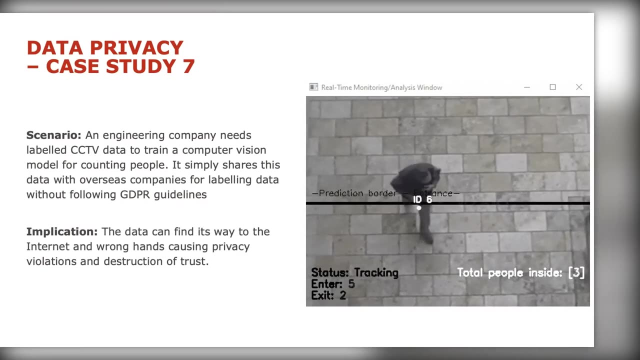 anything like that. what is the implications here? i mean, this is quite easy. um, if you don't follow gdpr, you are basically just giving your. let's say, this is a cctv data. this is, this is basically sensitive data. it's called pii information in it. 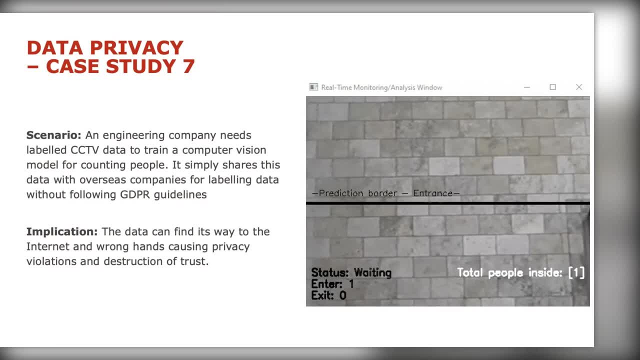 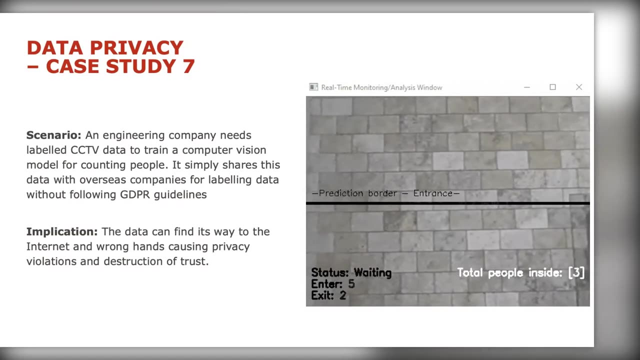 um, personally identifiable information. so what happens is, when you send this to an overseas company to label, you could end up with a financial lawsuit because, for example- i'm just i'm just giving a very, um, very exaggerated example- let's say we have some refugees that come here from another country. 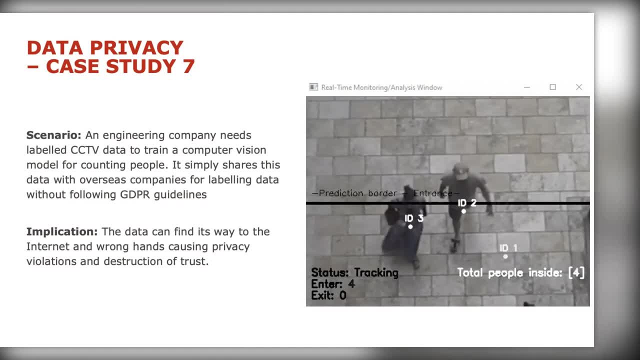 to the uk and then you have some cctv data of them. you send this data to a company in the country that they fled from and this data gets into the government's hands of that country and then they can start hunting them. that they know now where these refugees are, they can hunt them down. 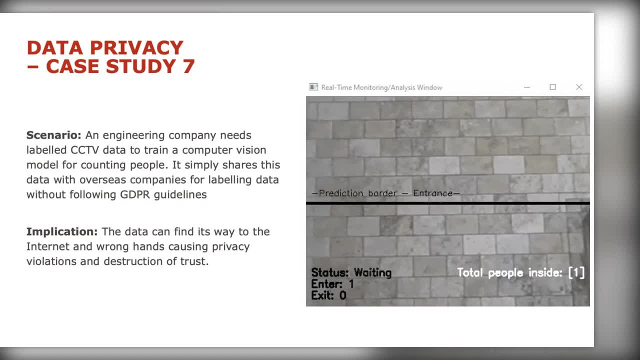 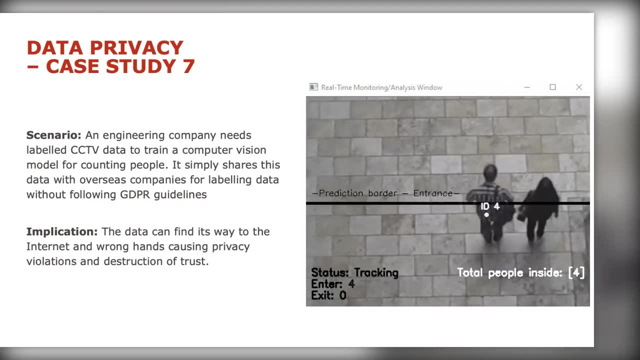 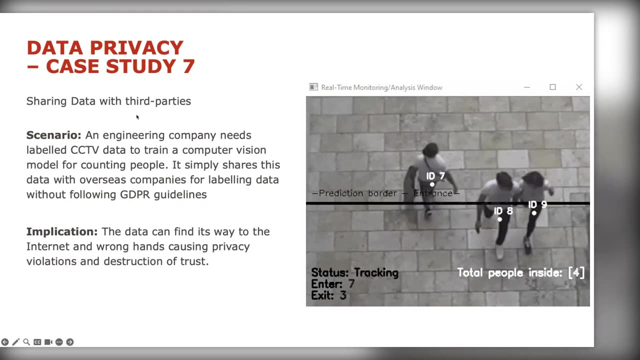 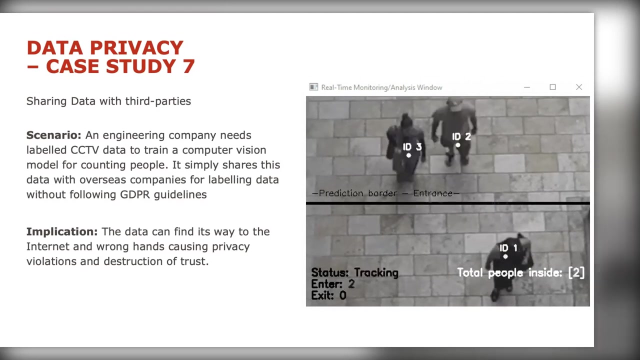 um channels, the whole um, she, uh and where they are in the country. and you know what's the concept of aButting in a tool which is τουςable, resources like cybersecurity and there of security practices in place. so that's like another reason. like ai, ethics come into play. 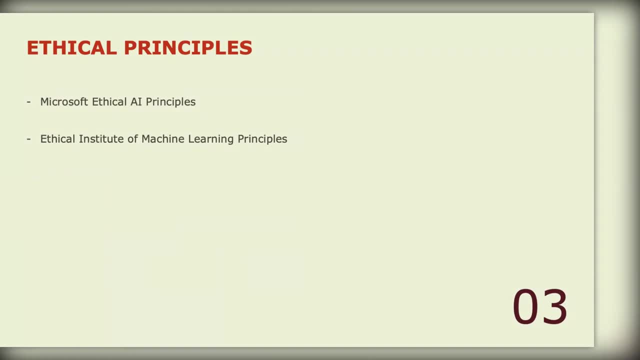 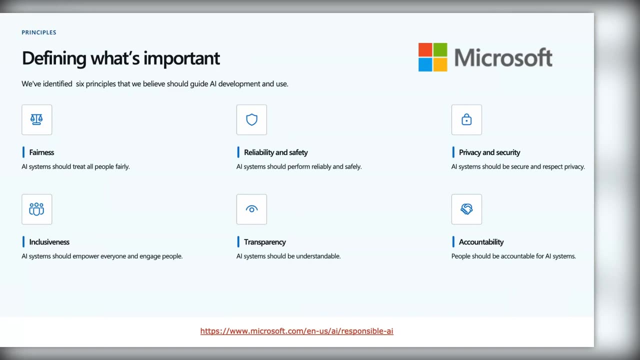 so, um, there are actually solutions to this and that we're going to go over quickly. um, so there are three different frameworks that have come into play. that allows us to, um, go over, um, like these various scenarios and make sure that we are applying them correctly. microsoft has put together. 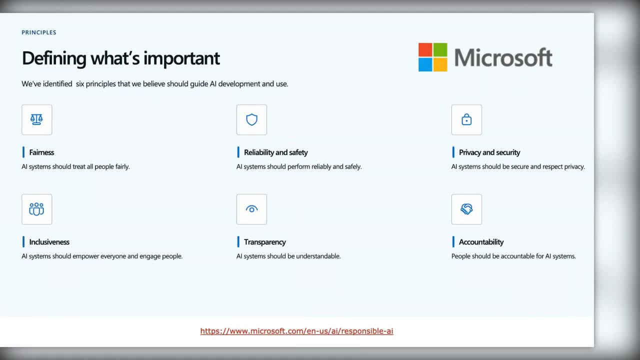 a framework um for what's the six principles that are important when it comes to applying ai models? fairness, reliability and safety. privacy and security. inclusiveness, transparency and accountability. so making sure that there is no bias in your data. making sure that it can perform reliably and safely so you have enough processes in place to make sure it catches those issues. same thing with 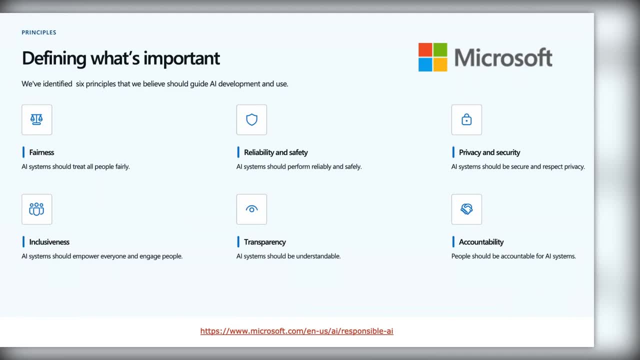 privacy and security, so you're not sharing pii data without proper processes in place. inclusiveness, so um ai systems should empower everyone to engage people. so you actually like showed, when you do collect data, you collect enough data of everyone and make sure there is no bias in it. uh, making sure that you can actually explain the decisions. 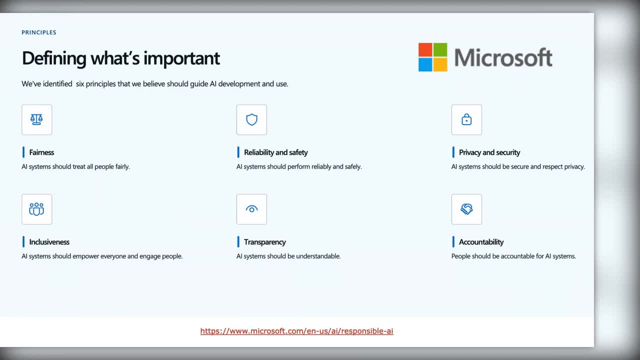 your ai models are making and you have transparent systems in place for describing how you built it so others can review, and so things can get pre-reviewed and you have accountability if things go wrong. there are actually certain people that are accountable for these ai systems, so this: 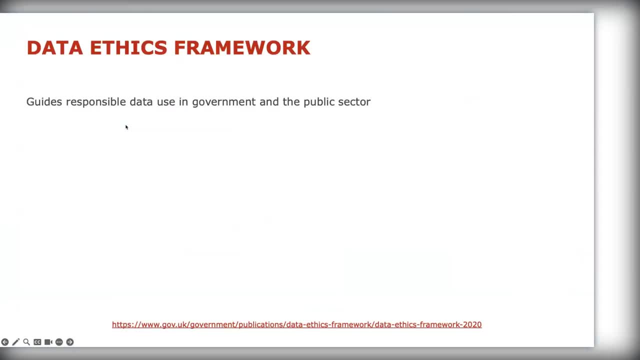 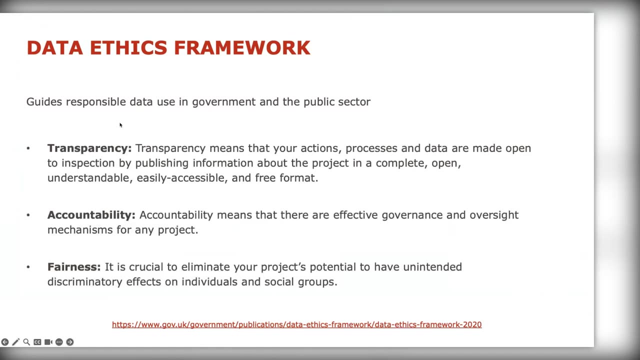 is a very interesting example of a framework that microsoft has put together, which is a good set of principles. there is also data ethics framework by the uk government office of ai, so this also focuses on transparency, accountability and fairness. so there is, like, certain themes in place, um so when? 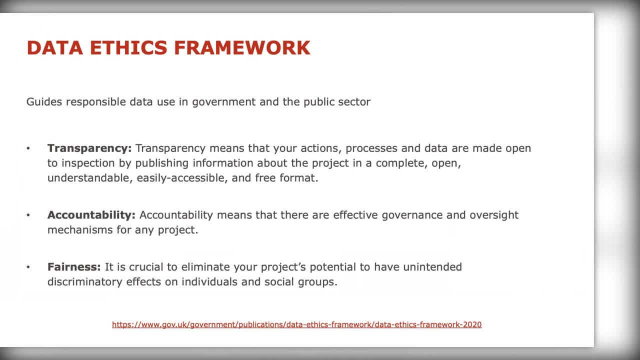 the transparency is basically means that, like um, actions, processes are made open to public for judgment and review and you publish that information so that, like others, can identify if there is any mistakes you've made and then you can then make a review of it. and then you can make a review of it, and when you 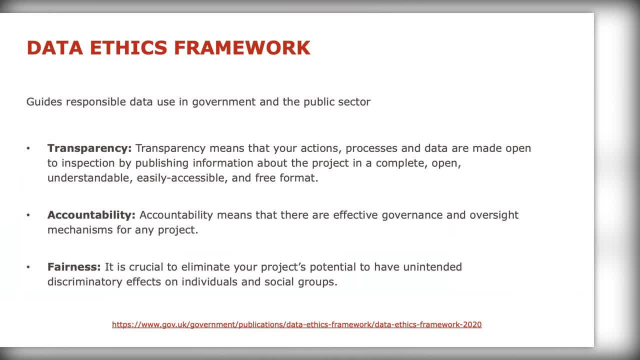 publish it. that way it's all easily accessible and free for everyone to review. accessibility, accountability- basically same thing. uh, we need to make sure that there are mechanisms in your projects to make sure, um, there is a whole like review process. people are accountable if things go wrong, so that any, any system that goes into production, it has gone through enough review. 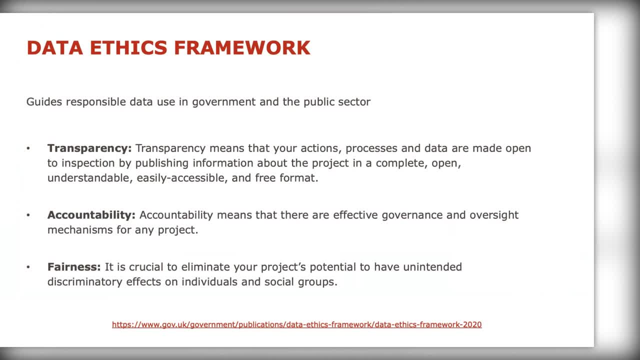 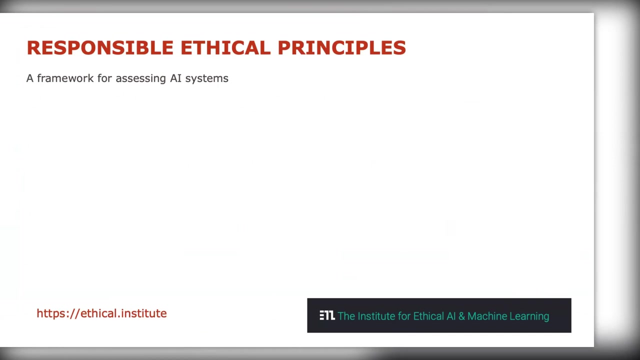 process. and also fairness- again, no bias in your data, so any unintended or intended discriminatory effects should be avoided. AI systems that are going to interact with consumers, So this goes into way more detail if you follow the link once we share these slides. Lastly, this is my favorite Ethical Institute, So the URL for this is ethicalinstitute. 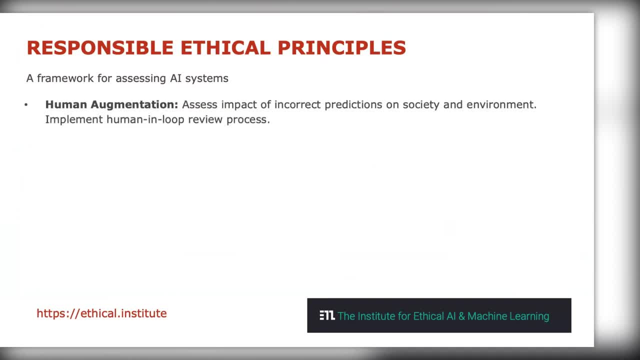 It's a machine learning institute for ethical AI machine learning. They have put together a framework with, I think, 8 to 12 items in it. that also goes way beyond those that we've mentioned previously. So one is: when you're building AI systems, you need to make 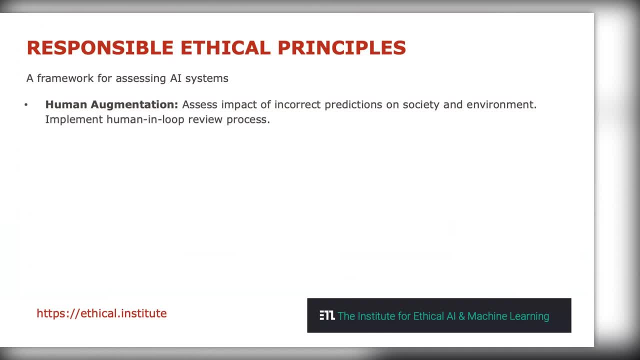 sure that impact of incorrect predictions on society and environment, like those risks, are identified and you have actually implemented mitigations in place to make those risks are eliminated or reduced, minimized as low as practically practical. This includes human in-loop review process, for example. So you have implemented systems and processes in place in your project that are going to be implemented in your project. So you have implemented systems and processes in place in your project. So you have implemented systems and processes in place in your project. So you have implemented systems and processes in place in your project. So you have. 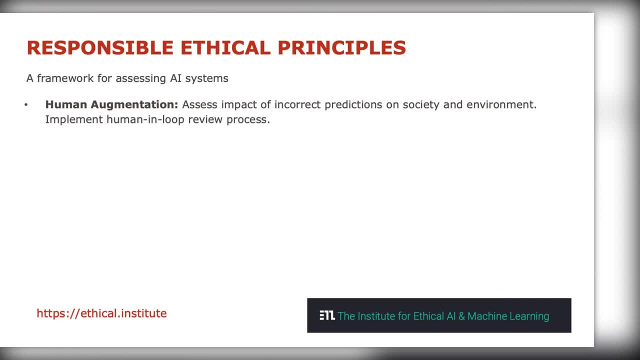 some inhuman involvement in how these AI systems work. Second one is bias evaluations. You understand, monitor and document bias in your data, So you have effective data analysis process to identify this bias and you have competent people for doing so. You can explain by justifying the processes that you've made to build your AI systems and 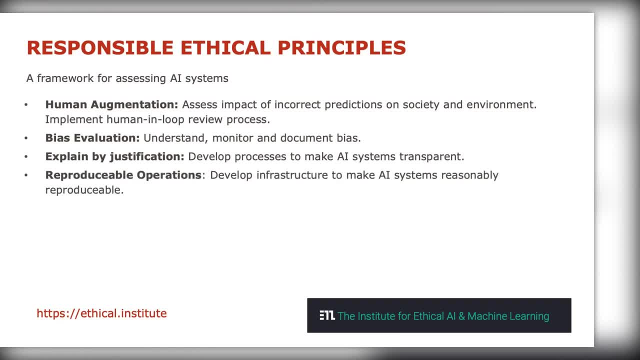 clean your data sets. You can reproduce your results. So you have infrastructure and systems in place that allows you to reproduce an AI system by just following a set of instructions and you can identify why that AI is reproducible. If your AI systems are going to cause job loss. 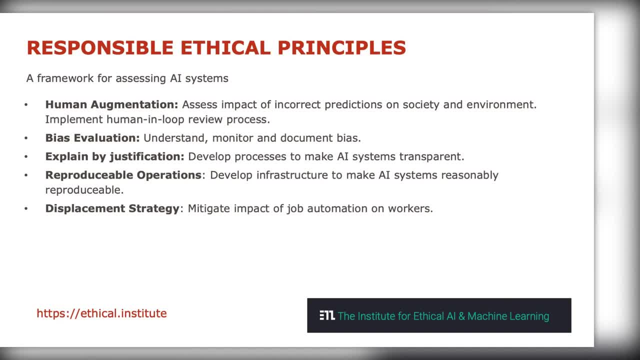 you have mitigated impacts of that, So you have actually plans in place for any displacement of workers. In terms of accuracy, the metrics you are choosing are suitable. So it comes back to evaluation metrics. And also, you are following any kind of GDPR guidelines, any kind of data privacy guidelines, So you are 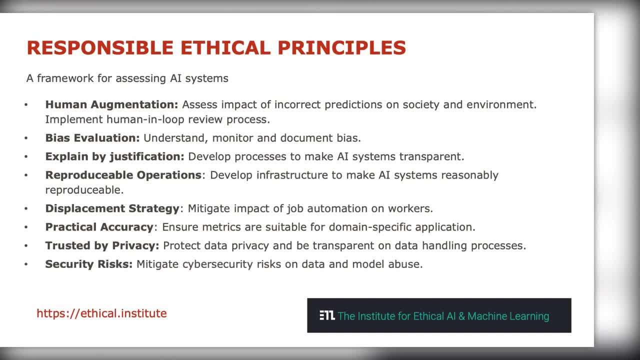 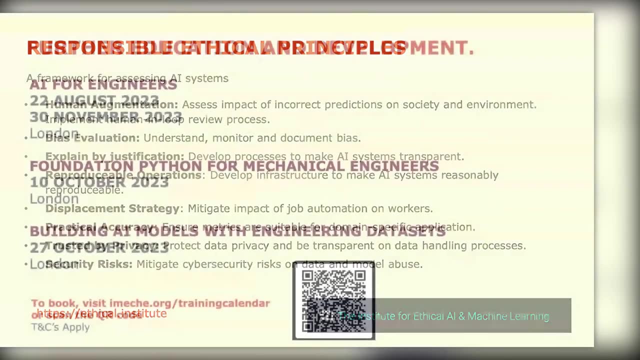 in any data handling process. follow those guidelines. Same thing with security: making sure you have enough cybersecurity measurements in place, standards in place, such as Cyber Essential Plus and all of those things, So that then any private data or any data, there is no model and data abuse, So your model is not leaking data. 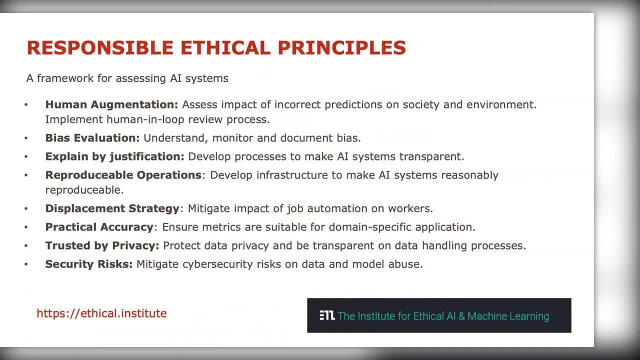 any private data to the public and it's safe to use your model even if someone starts abusing it. So this kind of like puts the whole framework in place. Hopefully these are very useful for you And hopefully you've learned quite a lot from today's workshop. 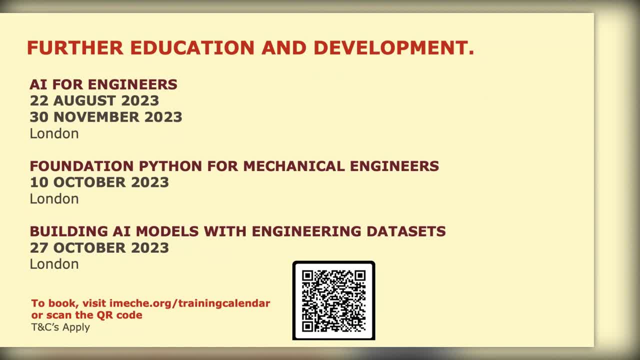 today's webinar. Anything that I've discussed today that kind of was not clear, we can answer in the Q&A session now. But if you want to learn more into deeper detail, there are some of the stuff and topics I talked about today. We do have these workshops, So AI. 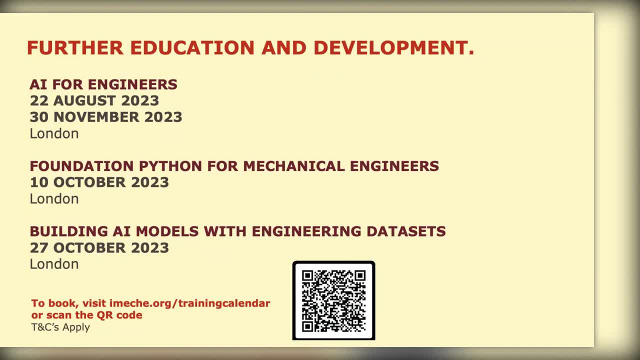 for Engineers goes into more commercial aspects, while the other two workshops they're all full-day workshops, So there is enough content to go into all sorts of details. So if you don't know Python programming and you want to learn it, there is a Python programming. 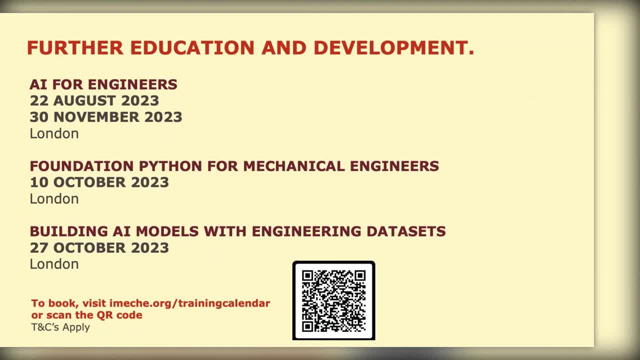 course on 10th, from beginning all the way to the intermediate advanced levels And then Building AI is basically a continuation of the Python course that allows you to then build AI models on engineering data sets that are predicting, for example, energy demands from demand and supply. 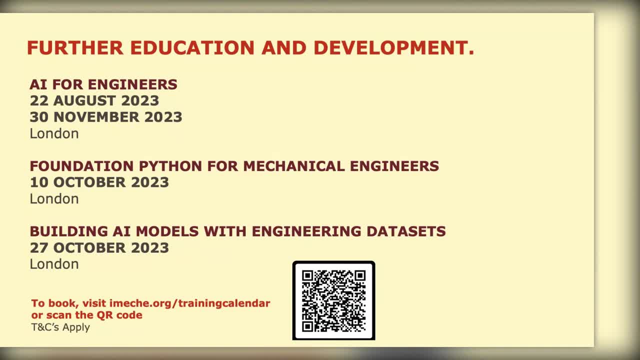 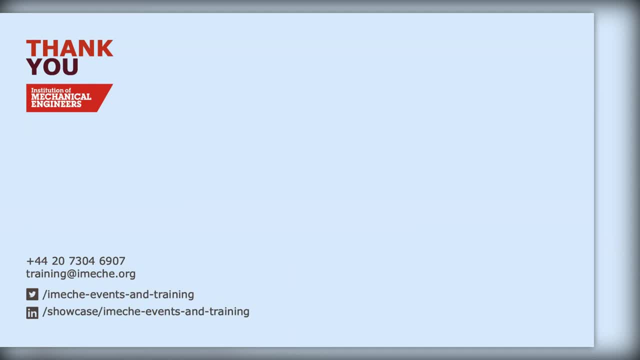 data set of energy data, But other than that, I thank you everyone for attending today. I think this is a good time now. Hopefully we have some time for Q&A. We can go through some of these questions that you may have posted in the chat. 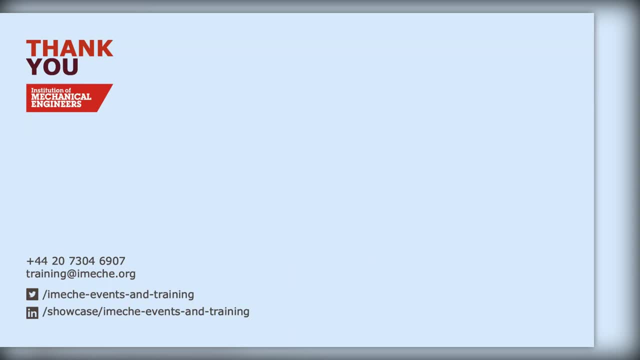 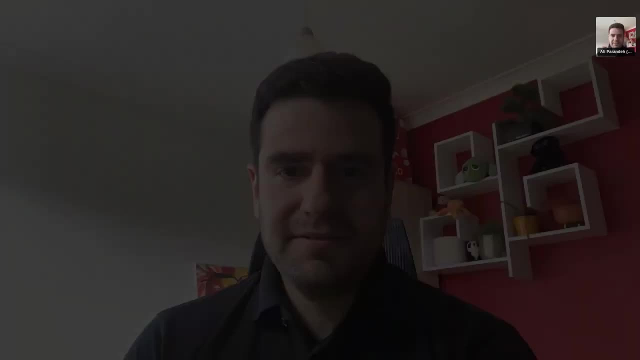 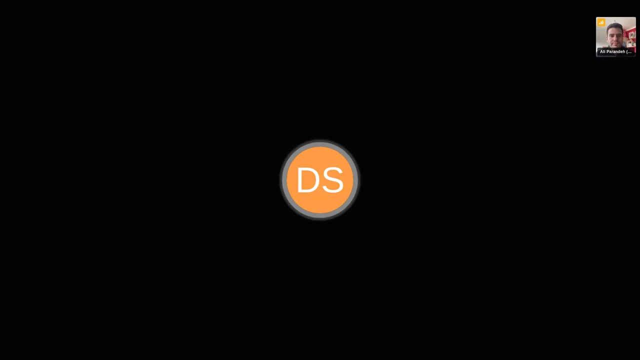 Right, Yeah, Thank you very much, Ali. That was fascinating. Definitely there was a lot to take in there, a fascinating subject and something I'm sure a lot of people have learned from today. So thank you very much. Yes, I mean, we have got some questions, absolutely. 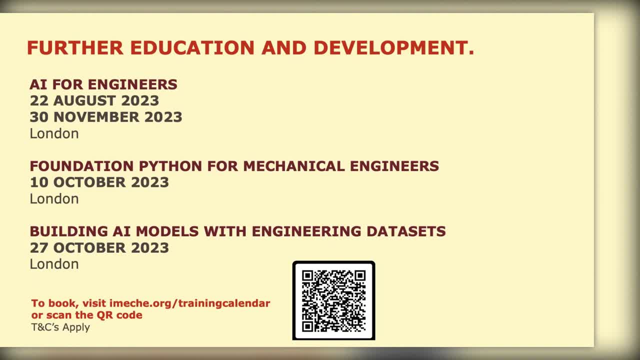 I'll just get your breath back. So one of the first questions came from Ed Blackwell. He goes: why is the black box not widely understood by humans? Is this just because there are so many mathematical functions? That is the case. yeah, Those neural networks that I show in the slides. 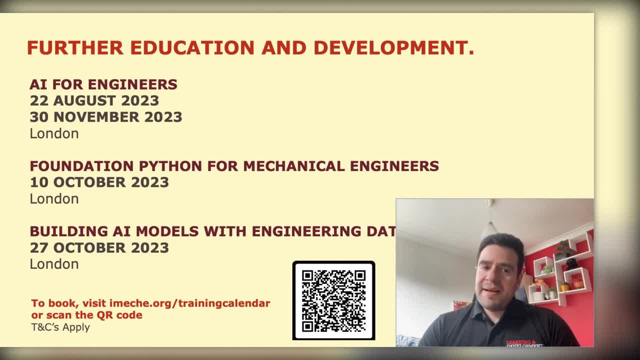 they are very simple. Most often you have about 200 layers. Some of these models are massive. They need, let's say, 40 gigabytes of RAM, random access memory, to just load the model into memory so you can use them, And they need a lot of hardware computational power. So the amount 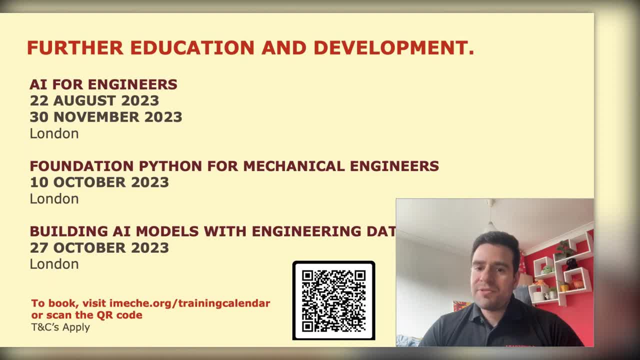 of mathematical computations going under the hood in these neural, massive neural networks. they are very deep And the architectures use very complex connections and patterns of how the data flows through. So it's very hard to understand how the data gets crunched and the mathematics work under the hood When we're building AI tools. any AI model is basically. 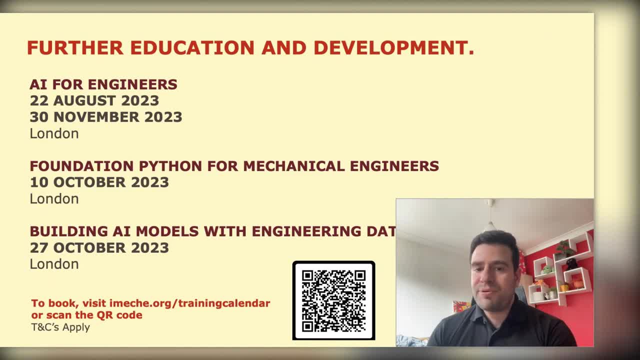 it's a mathematical function. So as long as you can define your problem as a mathematical problem, you can build an AI model for it. But often, if your problem is very complex- so, for example, I don't know identifying a cat from a dog- it's still very complex. It's still very complex, It's. 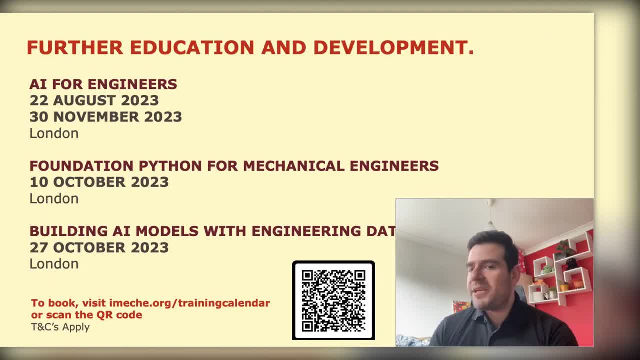 still a very complex problem because under the hood computers don't see pictures the way we do. They see just numbers, And it's because of the fact that these numbers gets crunched so many times at such a high level dimensionality it makes it really hard to understand what's going. 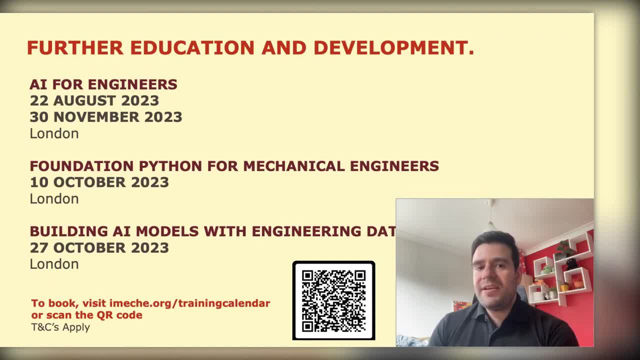 on mathematically under the hood, So you can just see a loss function or some metric is going down. Your loss is going down, But you don't understand why it's going down. What is it exactly that the model is learning? And that's why there is some amount of code going down. And of course you're. 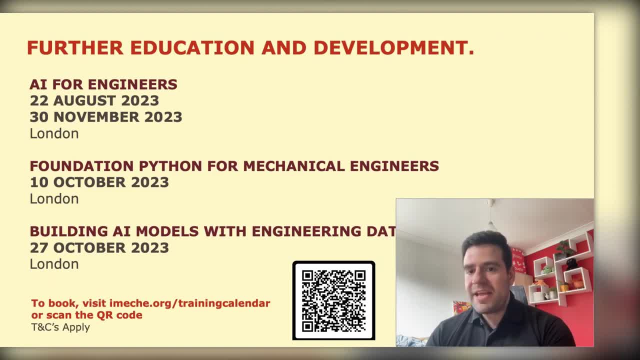 like there is so much research is going on into explainable ai tools to help us understand different layers of the neural network. what's happening in each one? fantastic, thank you. thank you, ali. um, yeah, we definitely have got some fascinating questions here. another one quite interesting one here. i'm not sure if you can. 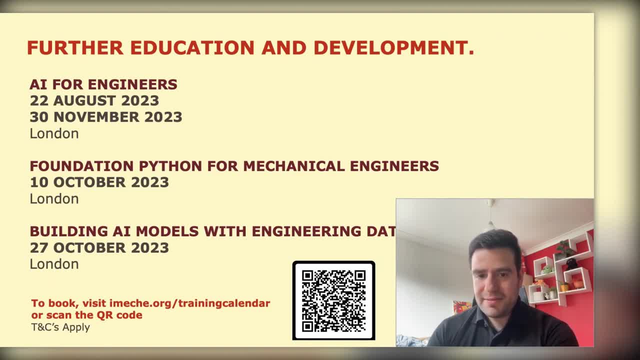 help here with. from william you, um, will the ai field propose laws similar to the three laws of robotics? um, i think, yeah, i think, i'm not aware of those three laws of robotics. so, um, i can, i can have a look and come back to you on that question. 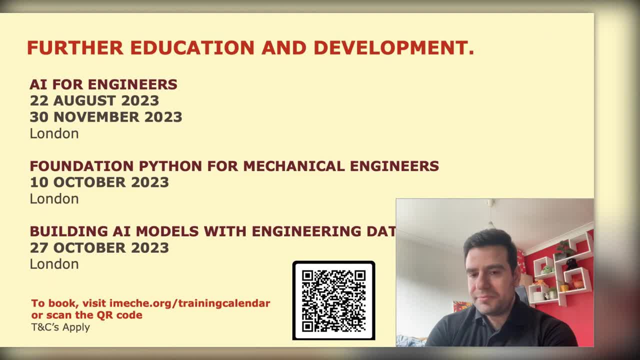 that's okay, thank you, um. this is from thomas reeves. what additional skills do you think we need in our organizations to learn to manage and accept the outputs from these ai systems? um, so there is a mix of commercial and technical um skills that might be required and part of the ai for. 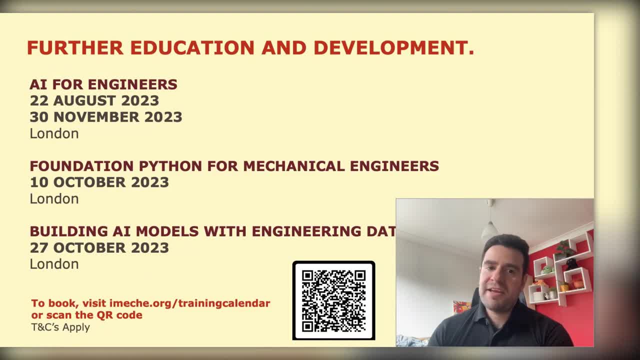 engineers. course, we're going to talk about building capability, ai capability in organizations, and there is a whole session on it. when it comes to scoping ai projects, um, part of this is you definitely, if you're going to be building anything that's very custom or like a proper system, you can use no code tools to build ai models these days. 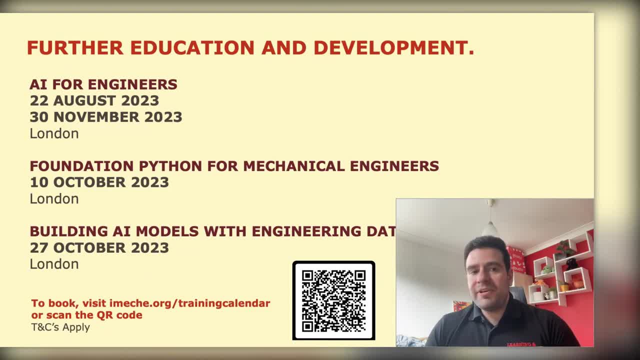 however, if you want to build anything that is actually proper, real, real real world scenarios, you will need to write programs. you will need to write, in most of the time, in python, and you need to use deep learning frameworks that are written in python, and it's more about understanding. 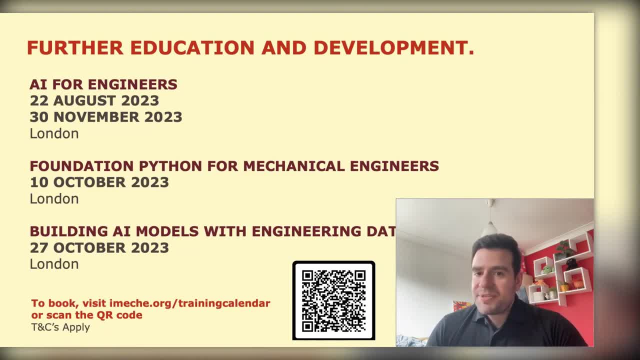 like of all the data science terms and the data science concepts, statistics and mathematics. so how these algorithms that you're using are crunching the numbers? um, because, if you, if you don't understand statistics, you know you, you will, you will end up with these, those pitfalls We just mentioned today. so you need to understand. 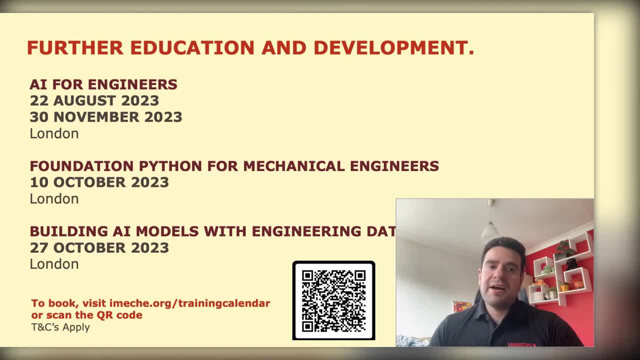 the whole process of how ai models are built and how, uh, the mathematics work, and there are some software engineering bits that you will need to know, that the, the organization needs, as well as commercials, Commercials such as intellectual property- who's going to be whose intellectual property will their models will be like? what if the data you 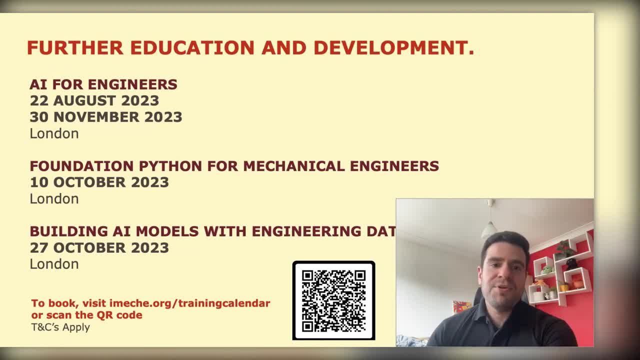 use is not yours, it's like it's the clients data. so there are always like complex bits around it that you will need, but oftentimes the technical team. you will require engineers who understand the data. you will require programmers who can write in python. this could be engineers as well. 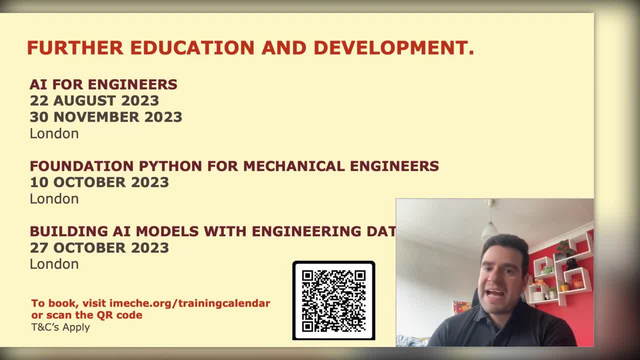 and you will need project managers who understand agile projects, because oftentimes these projects are more iterative. they need to go back and forth to progress. it may sometimes you may not be able to implement it in a waterfall manner, and you will need commercial people with experience in ai. 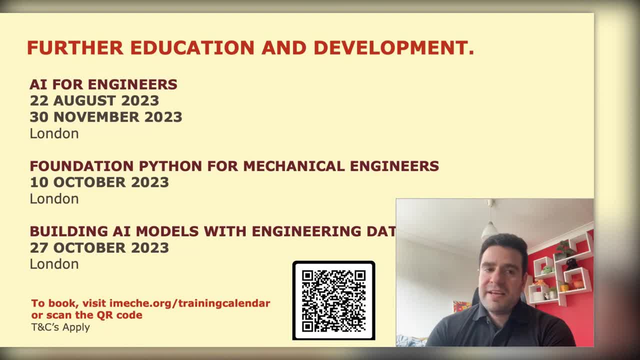 on the commercial side so that they can sell, they can gather data for these, for these ai projects, and they can support these projects. sorry, ali, i was talking. i hadn't unmute himself. i was just gonna say we're coming sort of very close conscious of time here because a lot of people will probably be finishing. 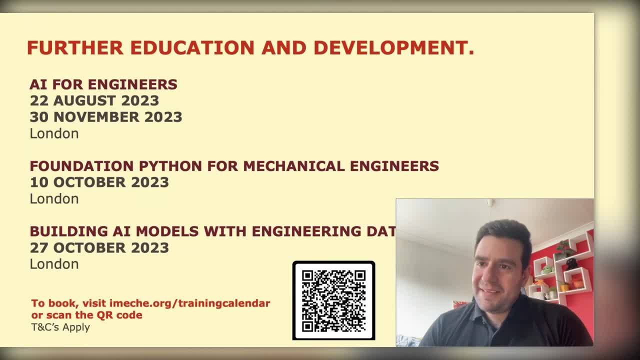 you know, i don't know if you can hear me off their lunch breaks, etc. so, um, we haven't got to get around time to answer all the questions, but we will have them recorded and we'll get them to feed them to you, ali, and we'll be able to. 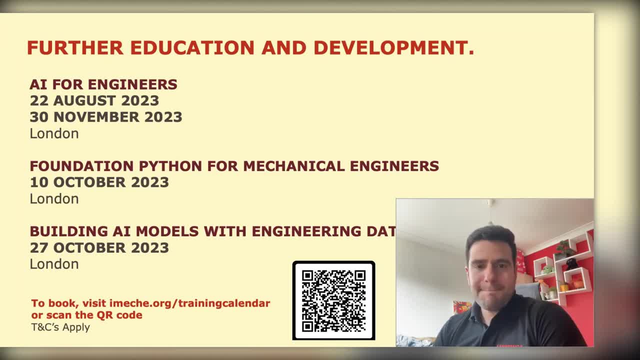 respond back to everybody who has asked questions, so, which is good. um, thank you again to phil lutzons, and he's just put actually into the chat box the uh three laws of robotics there. so, uh, someone's actually given a bit of guidance. um, i'll give you one more question then, ali. um, 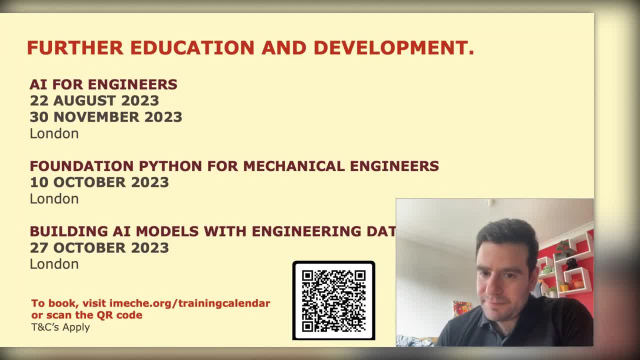 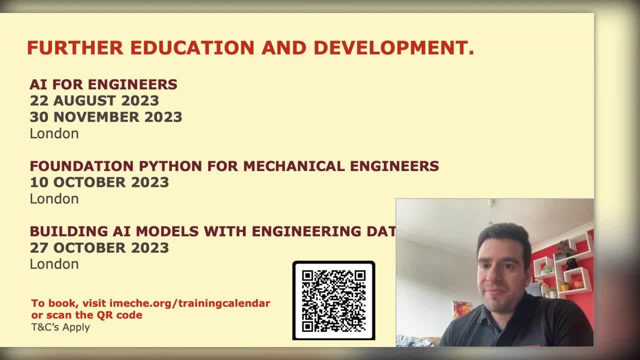 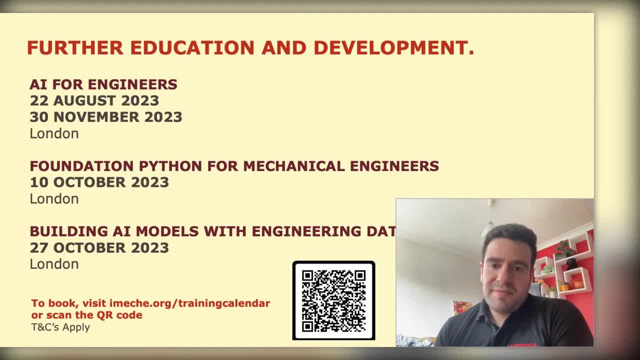 apart within the within the market, because normally small companies have very good specialist skills that normally large companies don't have and they can use that to their advantage to amplify that benefit. brilliant, thank you very much, ali um right. well, i, i have noticed a lot of the comments. 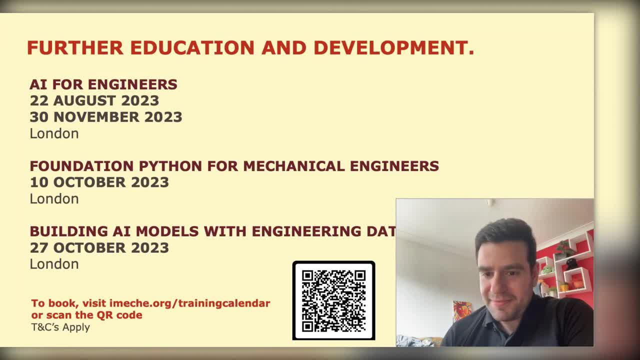 coming through and a lot of the comments have come to say you know how fascinating they found this, how interesting they found this webinar, so that's a really good feedback we've had so far. but, yeah, just want to say thank you very much, uh, for your time, ali. that was uh really interesting.